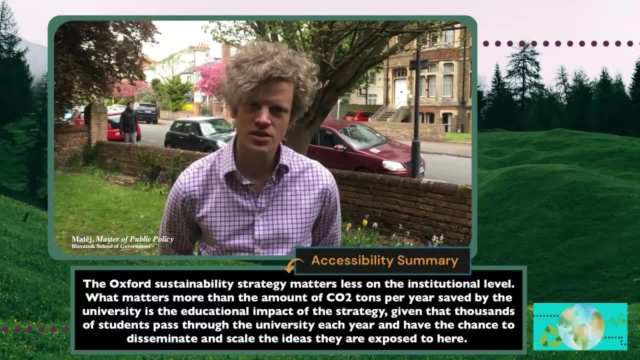 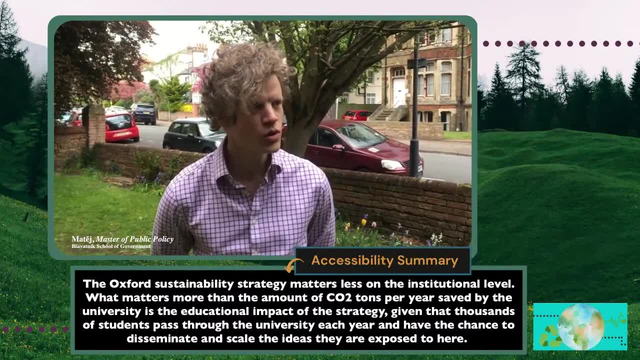 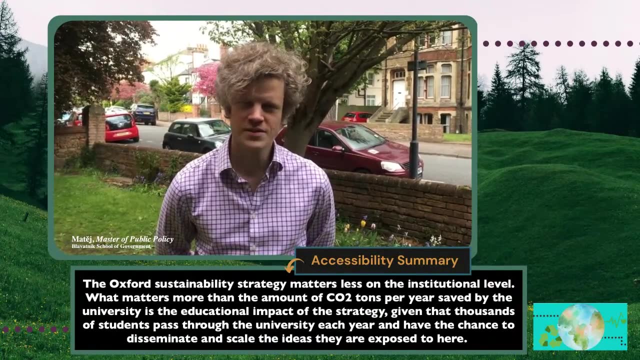 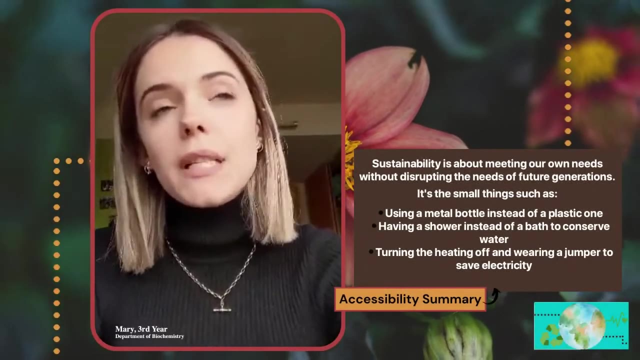 So I think the educational purpose of any strategy that we build is far more important than an actual CO2 tonne per year saved by the university itself. The university is a body of people, not an assemblage of buildings, So to me, sustainability is being able to meet our own needs as well as being able to 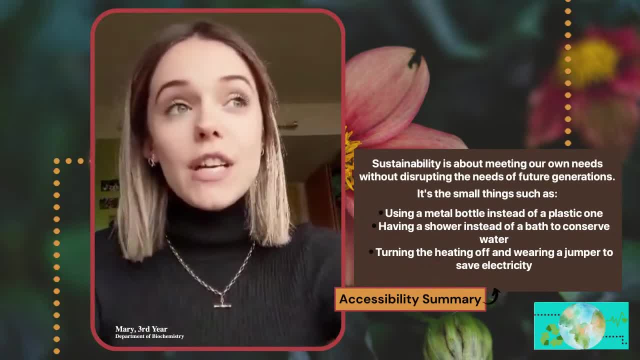 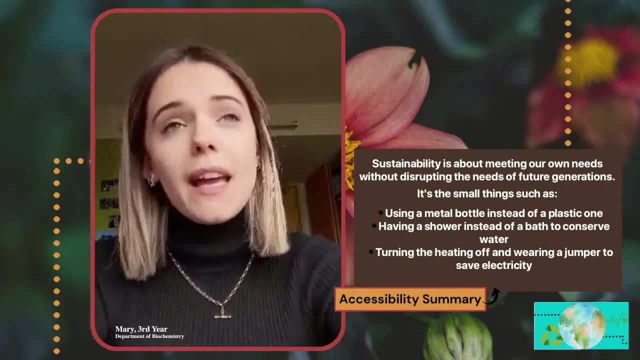 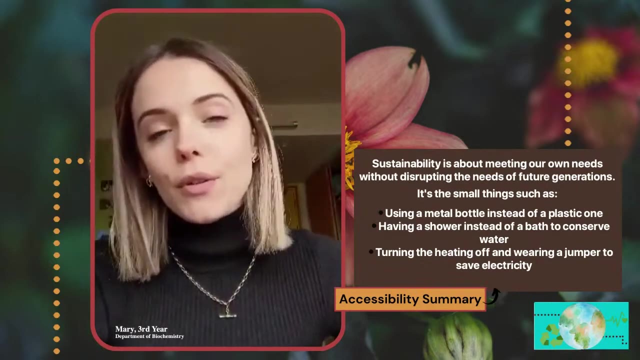 meet the needs without compromising the needs of future generations, And I think there's so many things we can do now to ensure that future generations aren't negatively impacted by what we're doing. And it's small things like using a metal bottle rather than a plastic water bottle when you're going to the gym, et cetera. 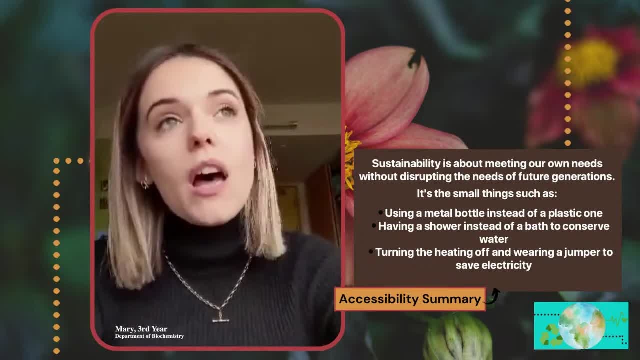 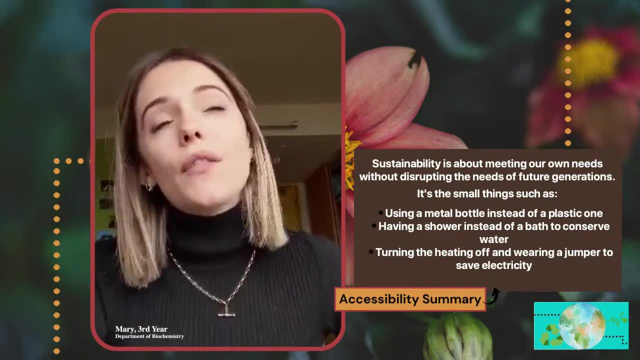 or having a shower instead of a bath to conserve water, or turning the heating off and putting on an extra jumper just to save electricity, and things like that, And obviously it reduces the burning of fossil fuels And it's just simple things that people can do every day. that, if 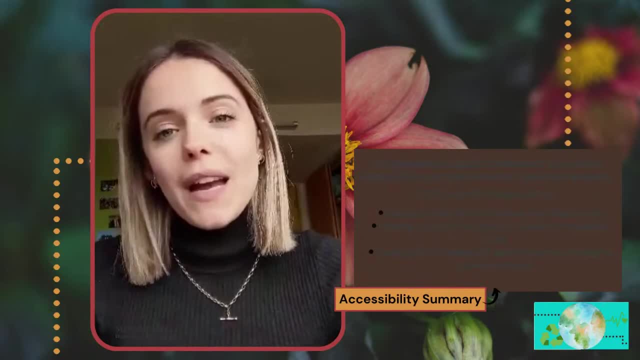 many, many people did it, then it makes such a huge impact. What do you think is the most important thing about the university? What do you think is the most important thing about the university? What do you think is the most important thing about the university? 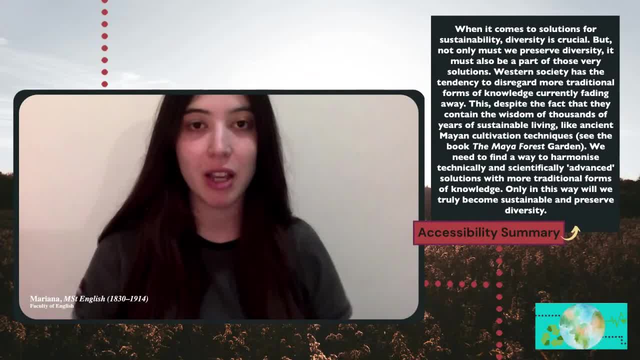 The first things that come to mind when I think about sustainability is diversity, But sometimes we're so focused on diversity or preserving diversity as a goal that we forget that diversity also has to be a part of the solution. In Western society especially, we have a tendency of thinking that solutions only come in the form of progress or technological. 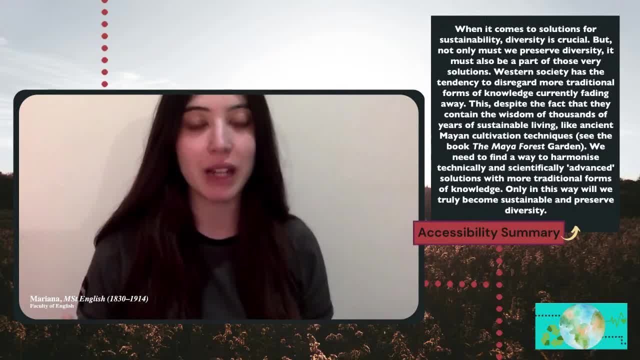 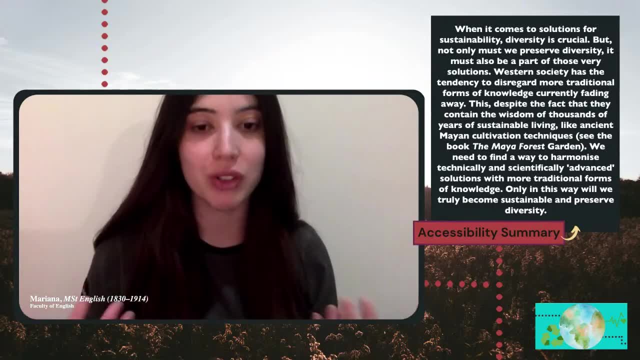 advancement or innovation of some sort, that we don't realize that sometimes the answers have been right under our noses for a really long time. I think that a great example of this are the more traditional societies that have lived perfectly sustainable lives for thousands of years. There's so much we can learn from them. There's so much we can learn from, for example, 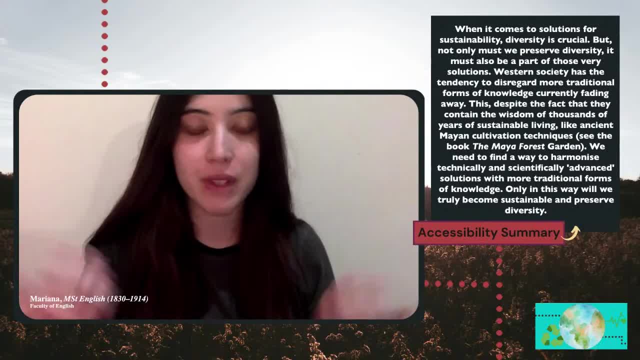 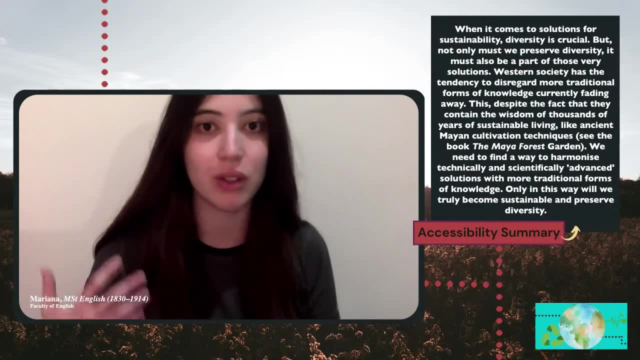 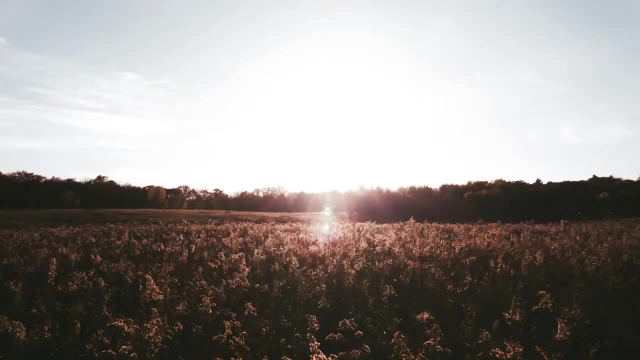 ancient Mayan cultivation systems. So I think that it's just important to remember that the knowledge of a scientist can be just as valuable as the knowledge of a forester in the Amazon when it comes to building a more sustainable future. What do you think is the most important thing about the university? 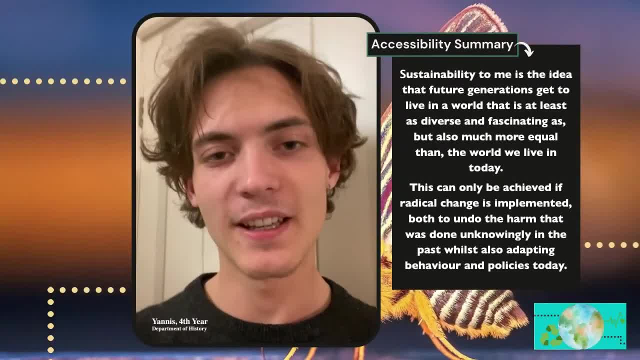 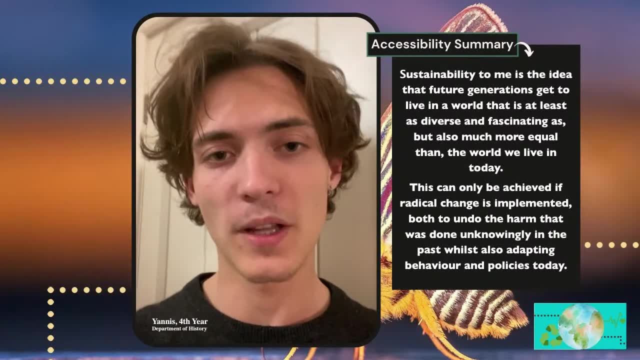 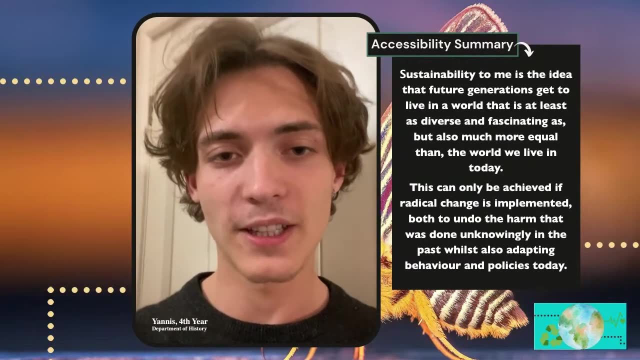 Sustainability to me is the ideal that future generations get to live in a world that is at least as diverse and fascinating as, but also much more equal than, the world we live in today. However, I realize that that ideal of sustainability can only happen if radical change. 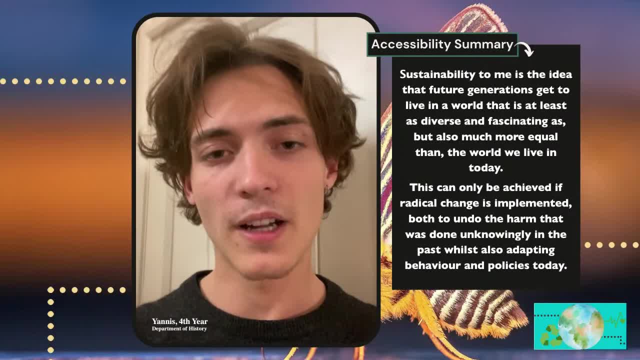 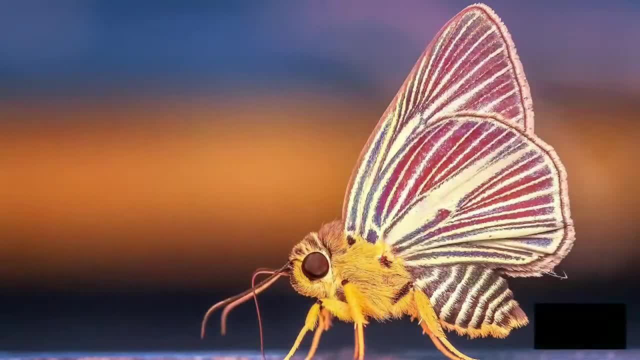 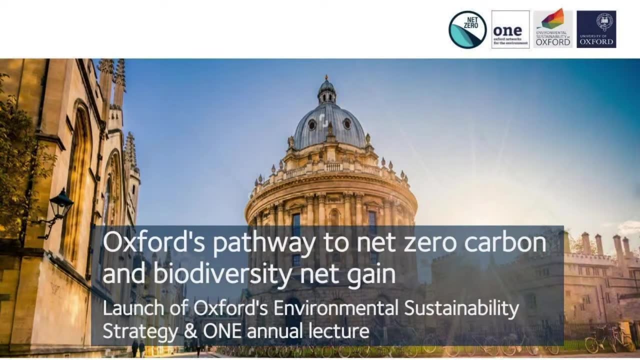 is implemented both to undo the harm that was done unknowingly in the past, while also adapting behavior and policies. today I'm going to hand it back to you, Jim, to take some questions. Good afternoon and welcome back to this afternoon's event. Thanks very much indeed to the 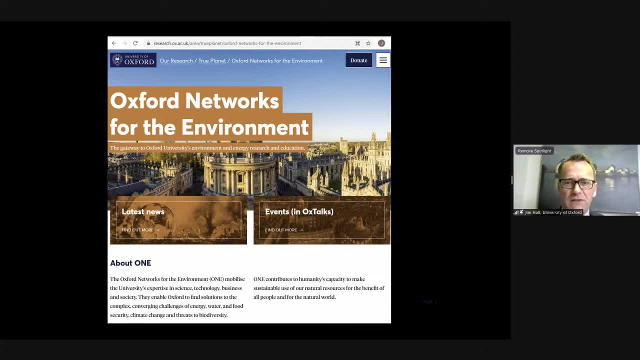 students who've recorded those videos which you've just seen, and indeed all of the students who've been working behind the scene to put the sustainability strategy together. My name is Jim Hall and I'm chair of the Office of Sustainable Development at the University of London. I'm the director of the Office of Sustainability at the University of London. 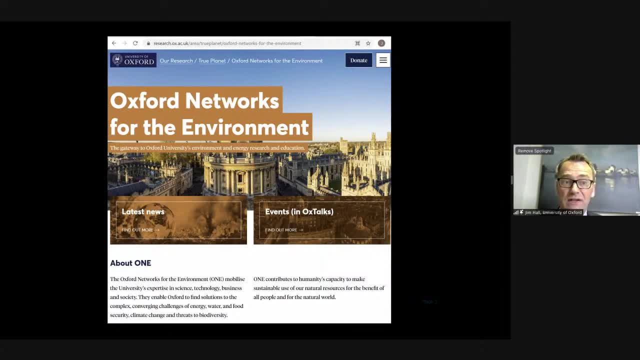 Networks for the Environment, who are co-hosting today's meeting. In a moment I'm going to introduce the one lecture for this afternoon by Professor Yadvinder Mahli, but first let me give you an update on the activities of the Oxford Networks for the Environment during this extraordinary year, and it's been. 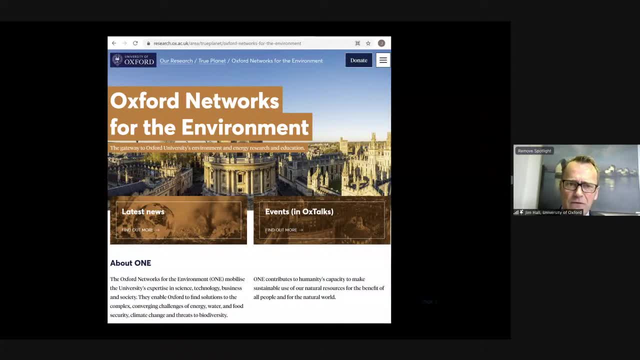 extraordinary in at least two senses, hasn't it? First, because of the pandemic, has locked down the university and driven one's activities- the Oxford Network for the Environment's activities, like today's lecture and panel discussion- all completely online, which has taken some adapting, as we all have. 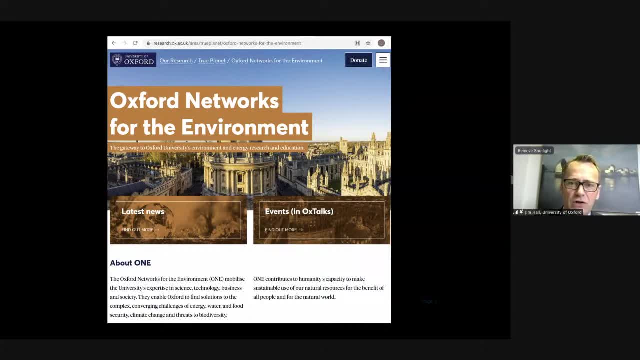 but it's also enabled us to reach much, much larger audiences through our work. An has also been extraordinary because of the ever-growing saliency of environmental issues- climate, energy, water, food, biodiversity- and a growing recognition within the University, as we just heard, of the importance. 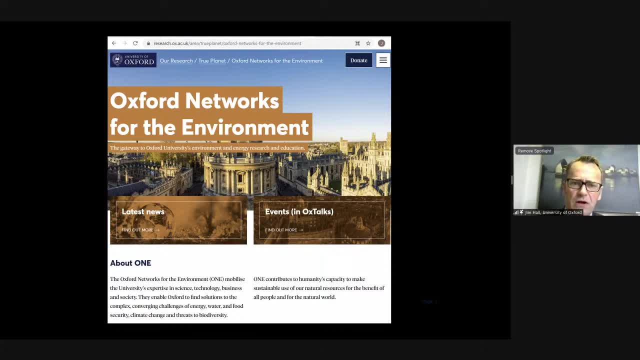 of Oxford's contribution in research to addressing those issues. The Oxford Networks for the Environment were created almost 10 years ago with the aim of joining up Oxford's research and enabling us to better tackle the great environmental challenges that we face. I describe one as having inward facing and outward 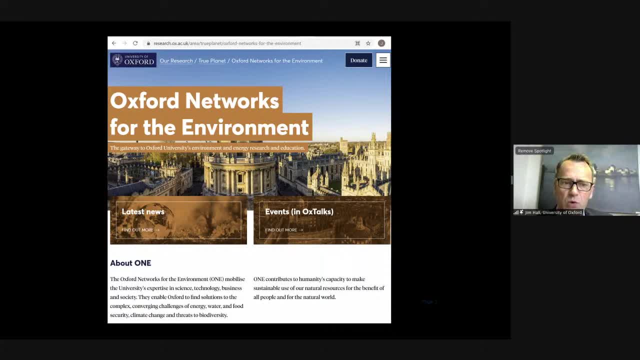 facing roles. Within the university, one promotes networking, shares information and, in particular, helps to join up interdisciplinary teams to respond to, and then they create big research opportunities. And then, externally, one provides the unified shop window exposing everything that we have to offer and so that enables us to interface with stakeholders in government. 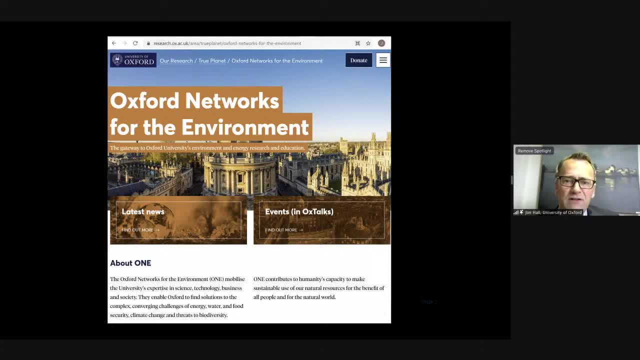 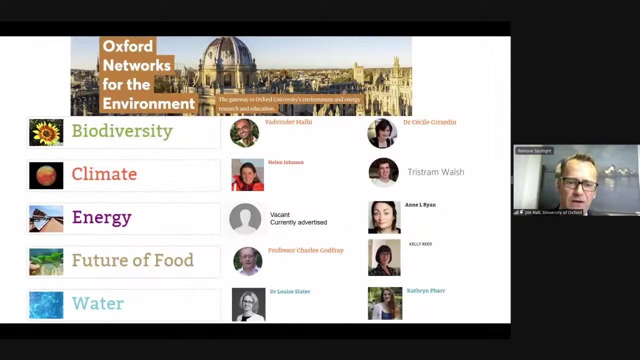 business and communities, And one example of that, for example, is you: the coordination of the university's research inputs to COP26, where colleagues in the Oxford Climate Research Network are helping to coordinate Oxford's response to an extremely complex but obviously crucial gathering. We do these things with the help of five network coordinators, who 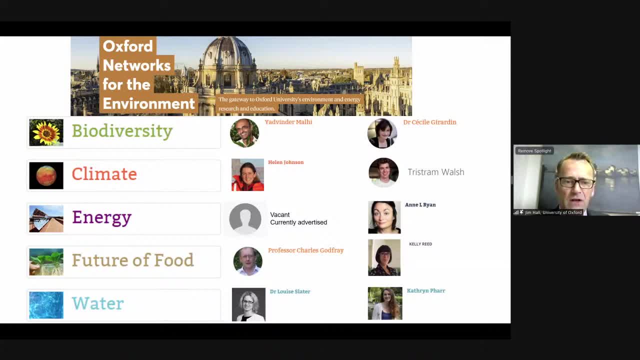 work with five academic network coordinators. We do these things with the help of five network coordinators who work with five academic network coordinators who work with five academic network conveners, though the energy convener post is currently vacant And the coordinators run. 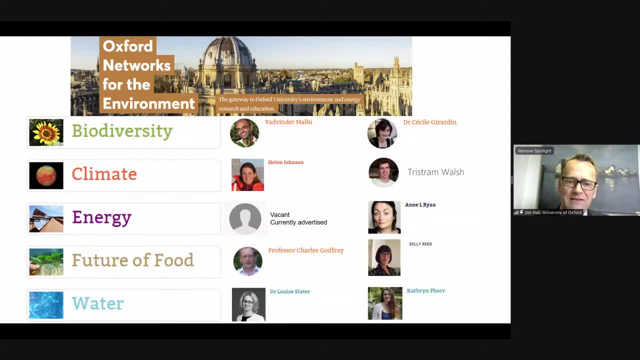 literally hundreds of events per year. They operate mailing lists, run social media, which I hope you're signed up to, and maintain five very active websites. We've recently advertised for student volunteers to assist the coordinators, particularly around areas of media communications organization. 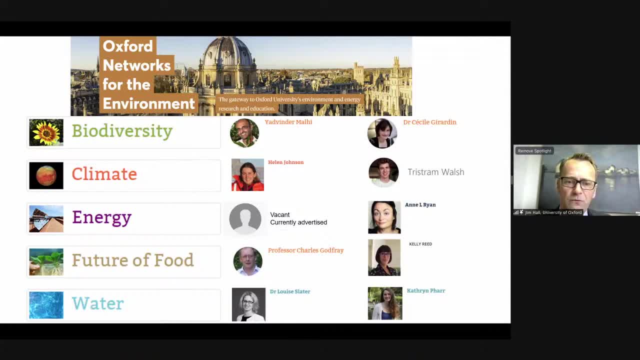 and social media, And we were amazed by the response which yielded more than 40 student volunteers who will be working with us in the future to further extend the reach of one in particular into the student body. Running five networks takes a bit of funding. 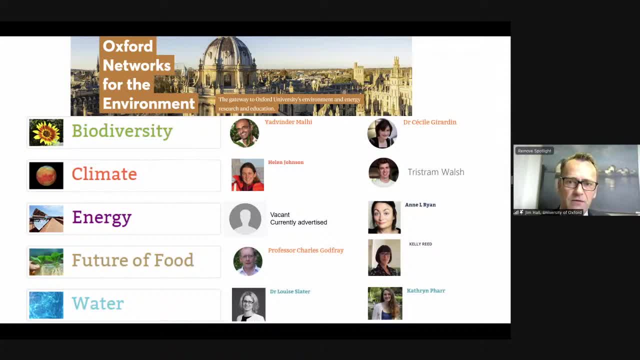 which we're most grateful is provided by the MPLS division, by the School of Geography and the Environment and by the Oxford Martin school of technology, and we're very fortunate to have the support of the MPLS division and the Student Body for today's research on climate change And the Minnesota school of geography and environmental importance can be found in the MPLS division's position. We are very appreciative of the participation. We hope to see you again on Tuesday. Thank you very much. 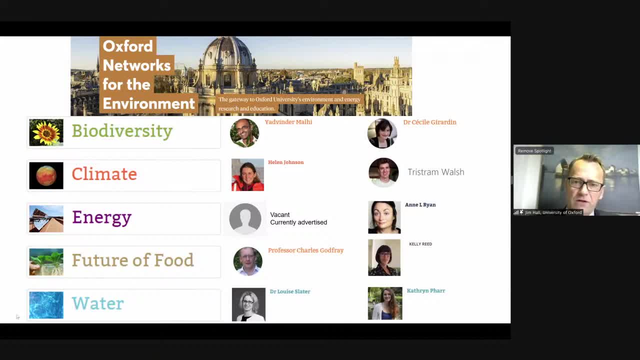 Thank you. And without that financial support we wouldn't be able to do any of what you've just heard about. And measuring the benefits of initiatives like one is not easy, because many of the things that one aims to do are actually quite intangible. 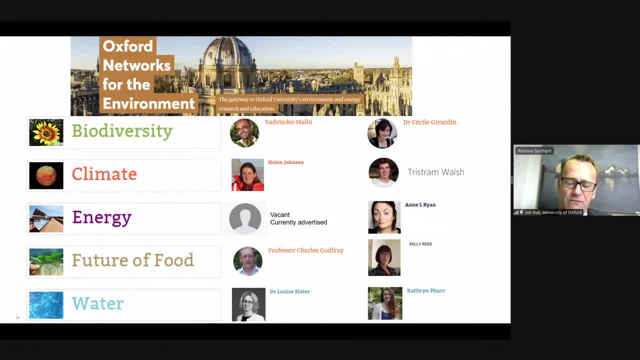 like knowledge sharing about what's going on in the environment across the university. And also it's hard to measure the benefits, because attributing big successes to one is not straightforward, because we don't have the counterfactual. But we do have some very big successes. 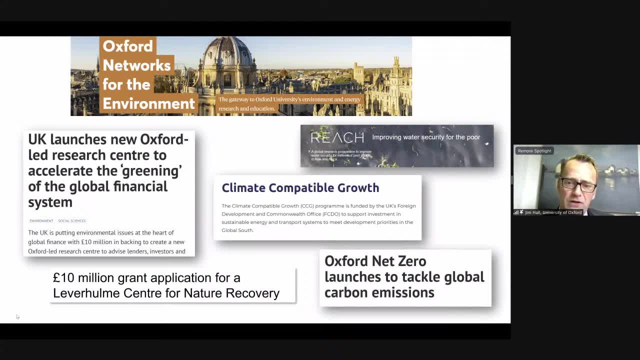 Here's just a few examples, including Oxford Net Zero, which Sam Bankos told us about in the introduction, which was a great example of Sam He explained, of interdisciplinary working across the university to tackle some massive environmental challenges, And those challenges and opportunities for Oxford's research to make an impact are getting ever greater. 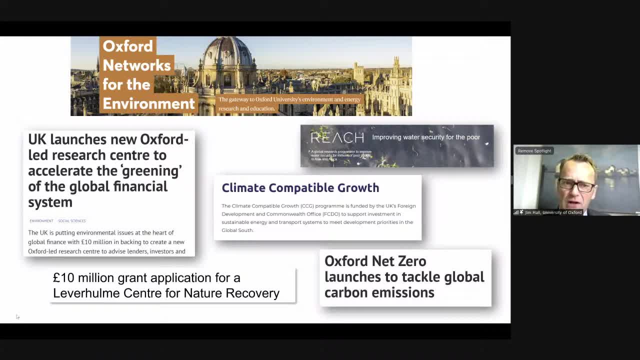 For example, the Wellcome Trust is focusing on climate and health as one of their big themes, So I'll be chairing discussions with representatives from across the one networks and the medical sciences division to discuss how we respond as a university And actually, if you're an expert in climate and or health and would like to get involved in that, 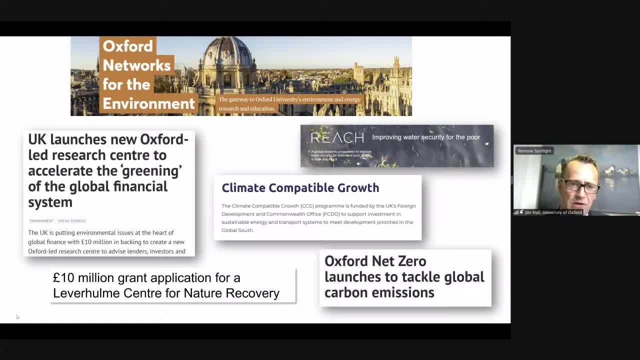 please get in contact with Tristram Walsh, the climate network coordinator. Today, as we've heard, is the formal launch of the university's sustainability strategy, which one has really welcomed and is supported throughout its journey. As we're all aware, the university is now under the very first act of its own. 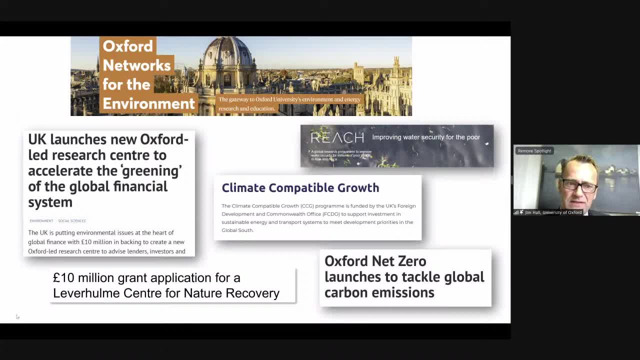 and it is now on the verge of its gestation. It's very important that the university gets its own house in order if our research and policy advice is to be taken seriously, And it's through, as we've heard, research and education that the university has the greatest potential to have a beneficial impact on climate and the environment. 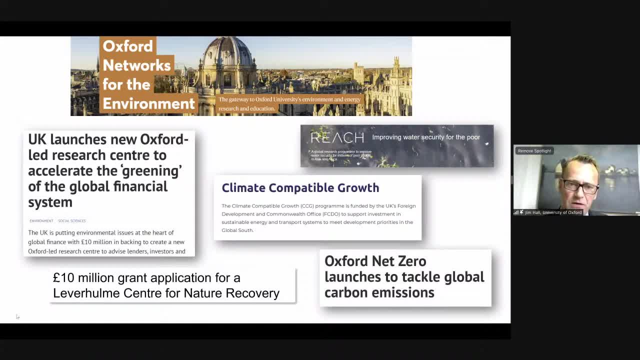 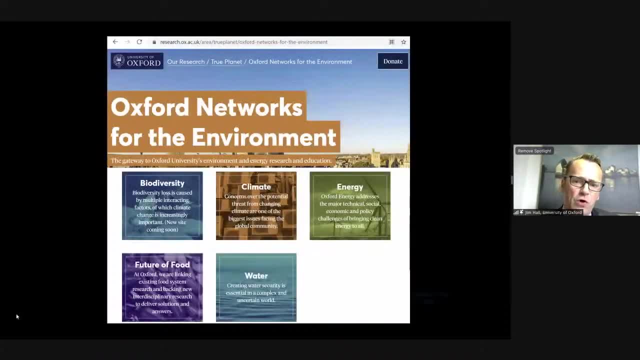 That's where we can have the greatest leverage. So you won't be surprised to see one as being rather central to our lives, Thank you. Thank you. central to the research parts of the sustainability strategy, Though one is primarily a set of research networks, we're also very supportive of the efforts within the sustainability strategy. 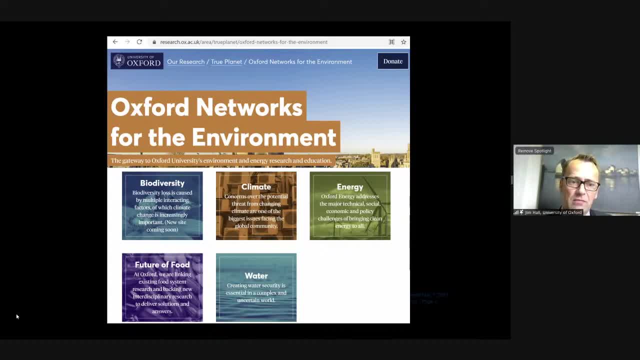 to advance environmental education. A fantastic example of that you heard from Ellie Holton about the Net Zero Homeschool, which was led with great inspiration and passion by the Oxford Climate Society. But we were really pleased that several one academics- Miles Allen, Matt Seddon- 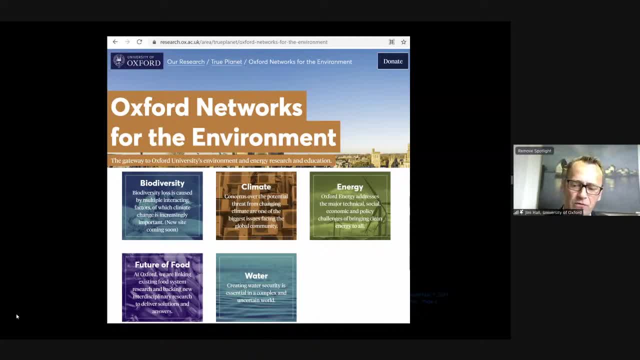 Tim Gruber, Steve Smith were able to contribute to that Net Zero Homeschool And we're really very pleased to see the sustainability strategy's commitment to look systematically at sustainability education across the university. I'm sure, as we'll also hear from the 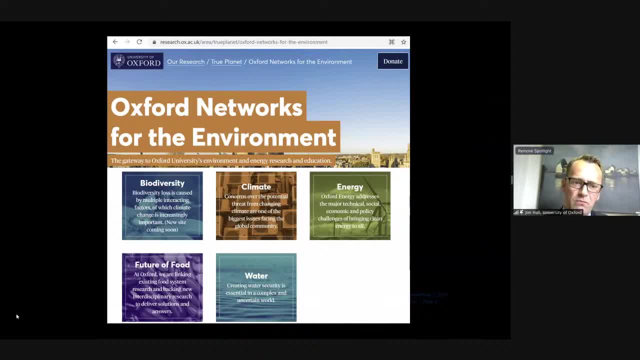 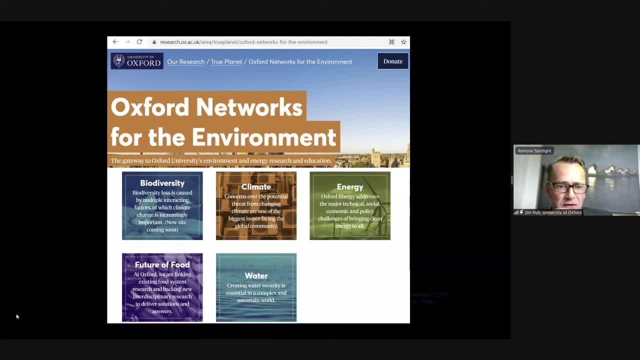 challenges like climate modelling and food systems. One is deeply engaged locally in Oxford City and Oxfordshire in, for example, energy innovation and energy efficiency, local transport and ecosystem restoration And in that sense we're all very, very committed to the in a moment. our research goes from global to global, as well as working on global science. 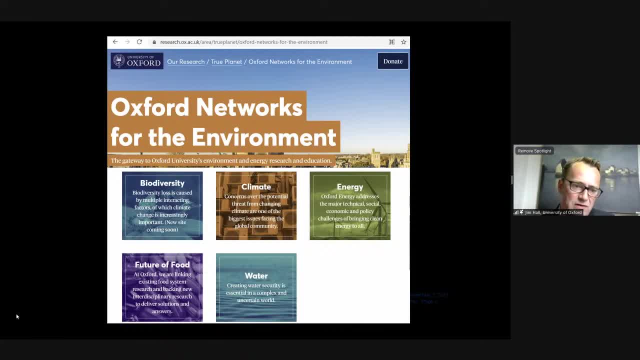 challenges like climate innovation and food systems, And in that sense, we're all very, very, very well aligned with the sustainability strategy, as the vice chancellor herself outlined. very well aligned with the sustainability strategy as the vice chancellor herself outlined. So we're very pleased to see the commitments in the sustainability strategy would provide. 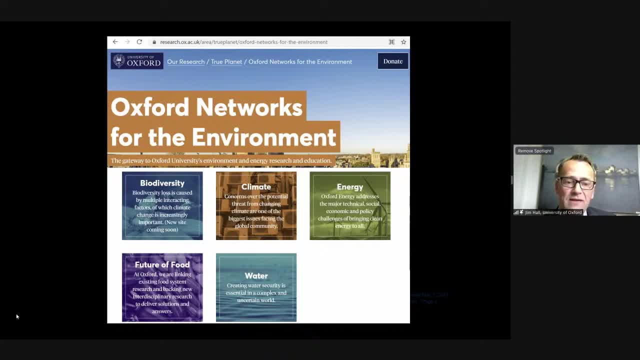 a high level endorsement of one, And reflecting that, the Oxford Networks for the Environment homepage, which you can see here, has been migrated to the Sustainability Strategy True Planet space of the Oxford University University, which you can see here, has been migrated to the Sustainability Strategy True Planet space of the Oxford University University. 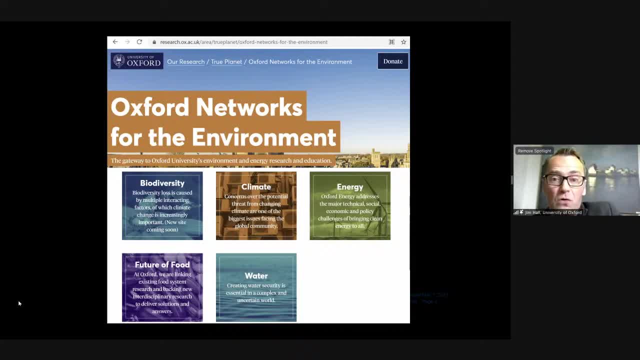 main web space. You can follow one's activities through those websites, our mailing lists, our social media, And I hope you'll join the many one activities during this incredibly important year. So now to the start. this afternoon's one annual lecture from Professor Yadvinder Mali. 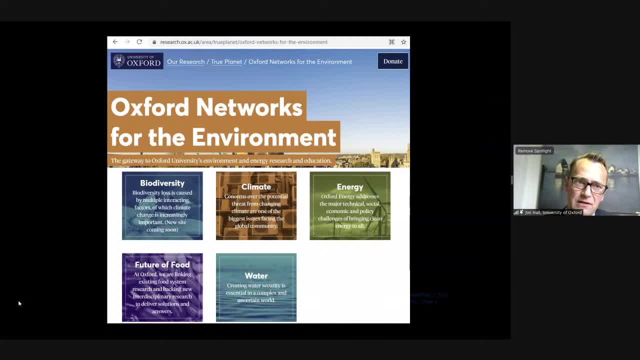 who actually probably needs a little introduction. So he's a member of the University of Oxford and indeed around the world, as he is world famous for his research on tropical forests ecosystems. Amongst many Excellence, he's a Fellow of the Royal Society, a recipient of the Royal Geographical Society's Royal Medal. 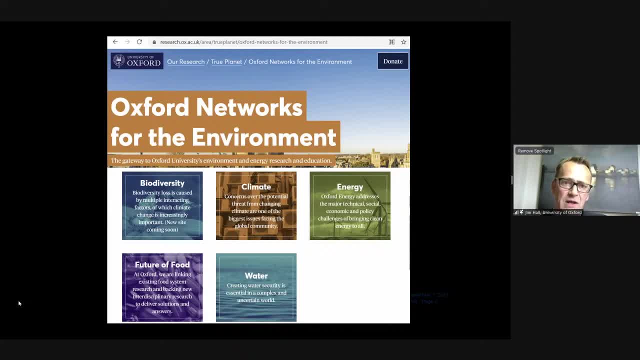 and was honoured with a CVE in London in 2016,, leaving his PhD with a Emeritus Award, year's Queen Birthday Honours And, as we'll hear, his research is not just in the tropics but extends to all sorts of biomes. He's actively researching in whitewoods and is responsible 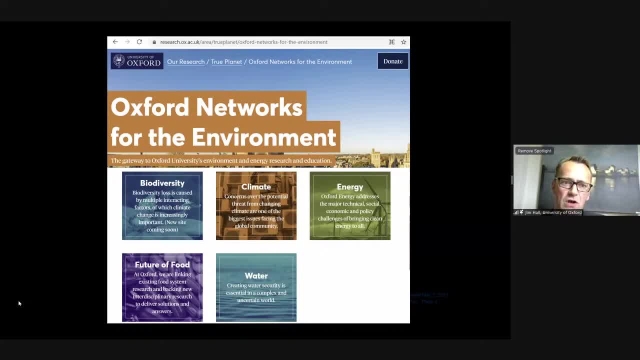 for ecosystem research and conservation across Oxfordshire, So he is the perfect person to give this year's one lecture at the launch of the University's Sustainability Strategy. Nirvinder Okay, thank you, Jim, for that wonderful introduction. Let me just share my screen. 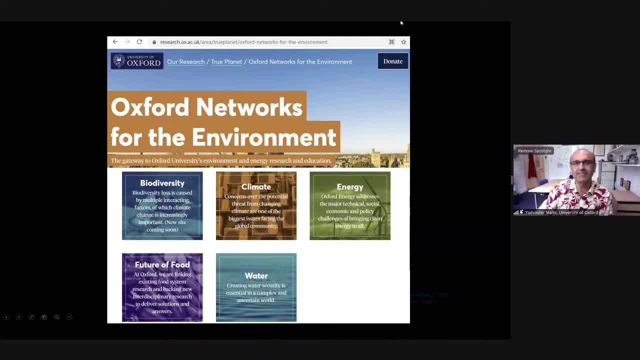 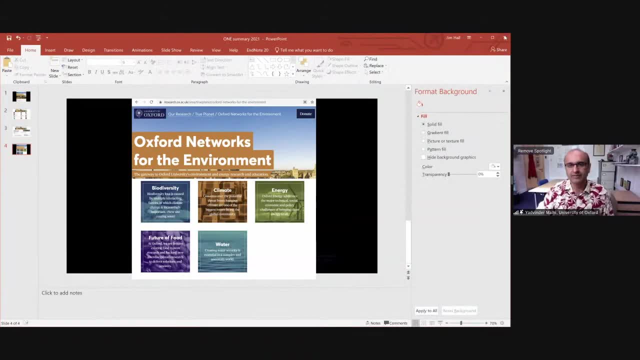 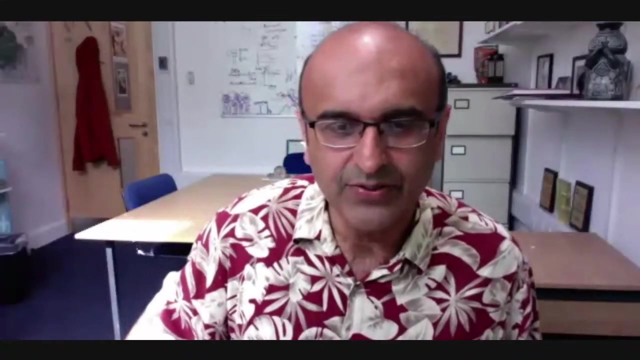 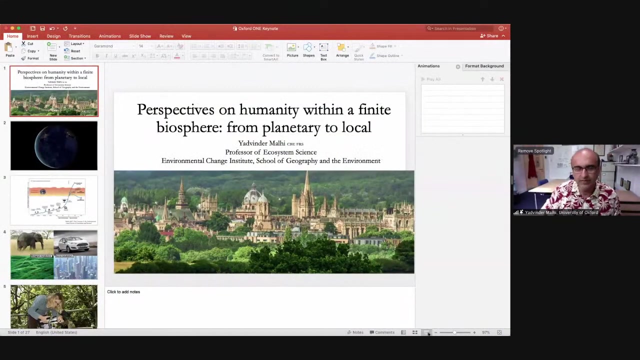 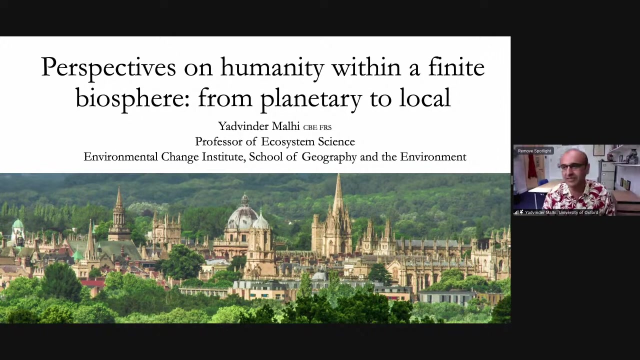 Can somebody give me permission to share my screen? Okay, so, Jim, if you could stop sharing, Okay, great, Okay, great. Thank you for the introduction and for inviting me to speak today, And what I'm going to do in this talk is perhaps take a different scale of thinking about sustainability and just give. 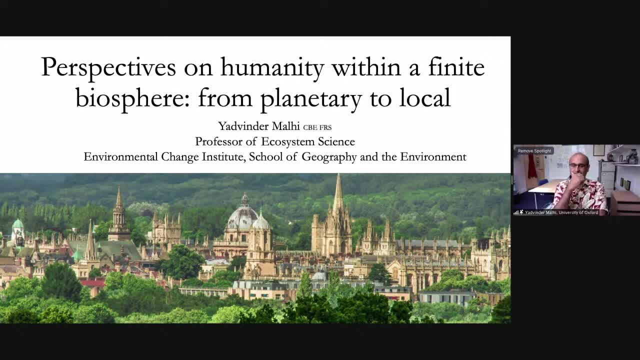 a few different perspectives on sustainability through a few slightly alternative lenses from the ones that we usually address, just to have a slightly different perspective on it. When I was preparing this, I grabbed this photo from the University webpage and I like it particularly because it really shows the University, but it really shows it embedded within the local. 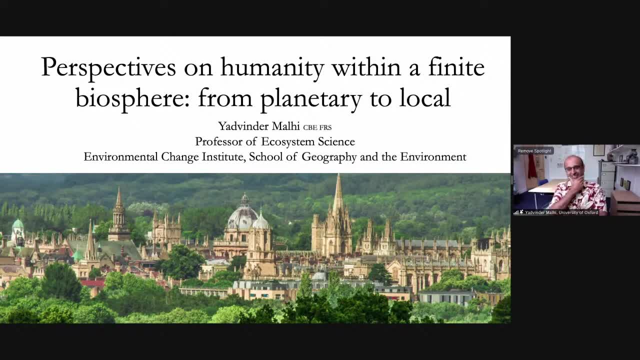 biosphere. In fact, from this angle it actually looks like it's sitting in the middle of a continuous rainforest, But what I think it does show is the importance of the geographical location of the University in the local biosphere and, within that, in the global biosphere, That's. 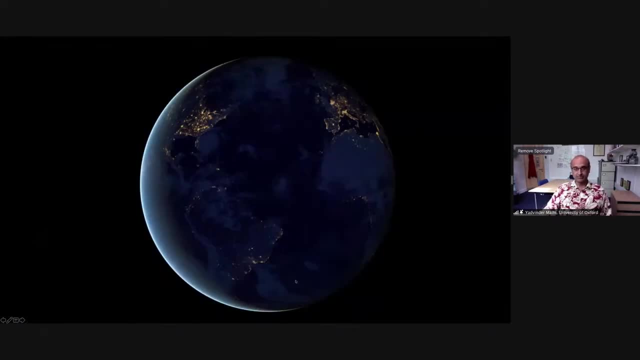 one of the themes that I will pick on in my talk. I'd like to kick off a lot of my talks, often with this image, which is an image of the planet with the lights of human activity and cities, in particular, lit up at night. I like this image for a lot of reasons. I think it's 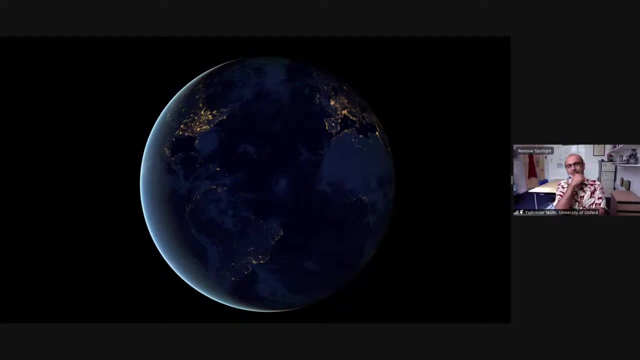 important to always remember that this image frames every human being alive and every human being that has ever lived, And, more profoundly than that, it frames every living organism that we know of that lives now or has ever lived in this entire vast universe, Until the Mars rovers dig up some surprise for us, perhaps in the near future, And that's a profound 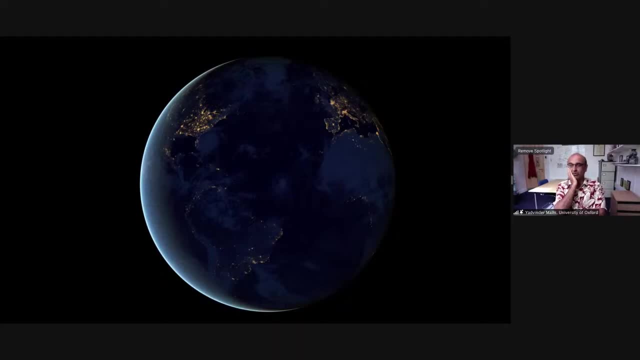 really humbling thought. in this entire vast cosmos, All the living organisms we know of are found framed in this single picture. It also highlights many of the glories of modern human civilization: The technology that enables us, in the midst of a pandemic, to sit here to communicate. 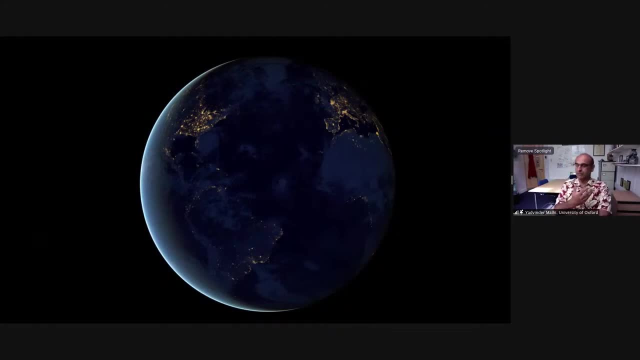 with each other. The technology that enables us to sit here to communicate with each other, To be sitting in relatively comfortable housing and in generally healthy conditions, and to be able to communicate like that. That is one of the glories of modern day life. 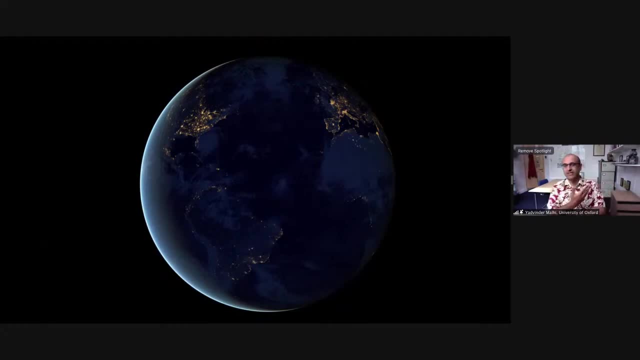 But it also highlights many of the challenges that we face in sustainability: The expansion into the biosphere, an abuse of the biosphere that increases the risk of things like this pandemic. The injustice and inequality of our distribution. Some continents here are lit up brightly. 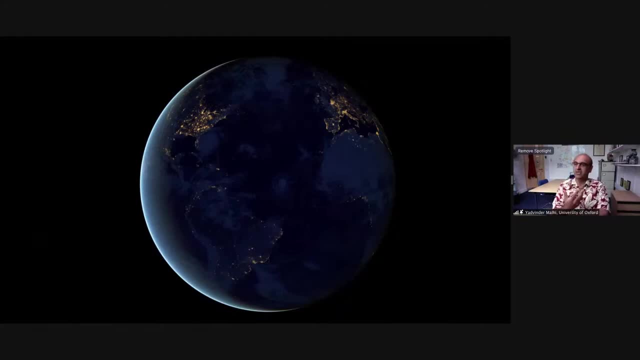 Other continents equally populated are in energy starvation and they don't have access to the resources they need for people to live decent lives. And the feature that will be the theme of this sustainability question is also the simple abundance of human activity on the scale of the planet, And, in fact, seeing this planet as a 3D globe exaggerates the size. 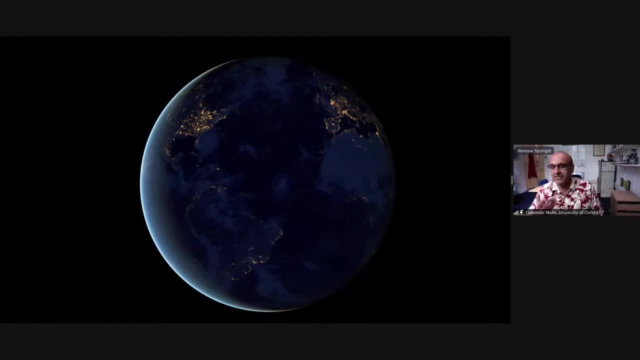 of that planet, When we realize that all of that human activity is occurring in a thin shell of this image, A few kilometers deep of atmosphere and a few meters of biosphere that are holding on and sustaining all this activity. And I think that is perhaps one of the profound shifts that 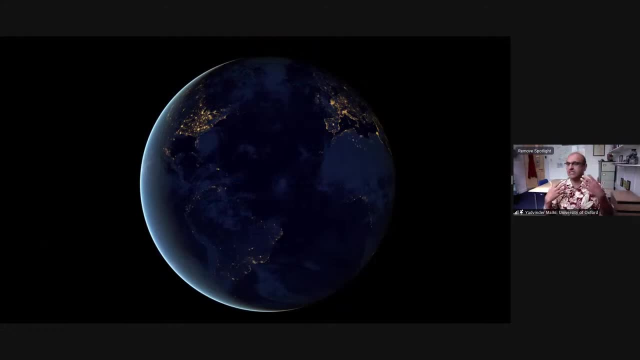 we're going through in our age, A profound shift in the way we see ourselves in the universe. That is as profound as a shift that came about with the Copernican revolution, where we de-centered the earth as the center of the cosmos, or the Darwinian revolution that de-centered humanity as a centerpiece of a living creation. 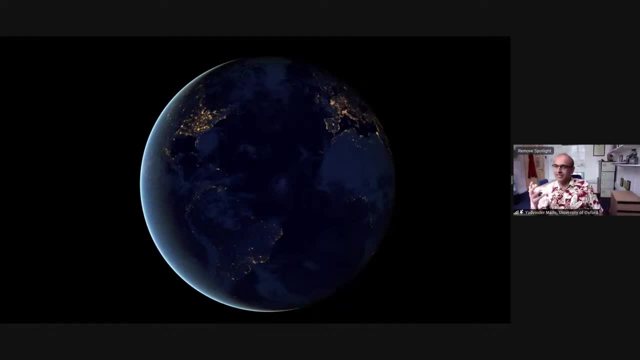 And that realization is slightly opposite to that Darwinian Copernican trend, but it's that realization that we are large relative to the planet, That the planet is small and humanity is large, And learning how to live with that realization and how to adapt that. 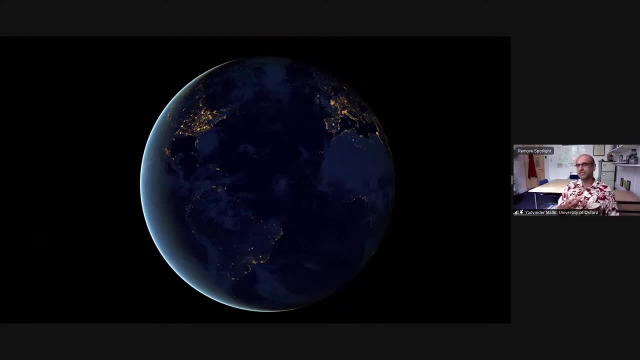 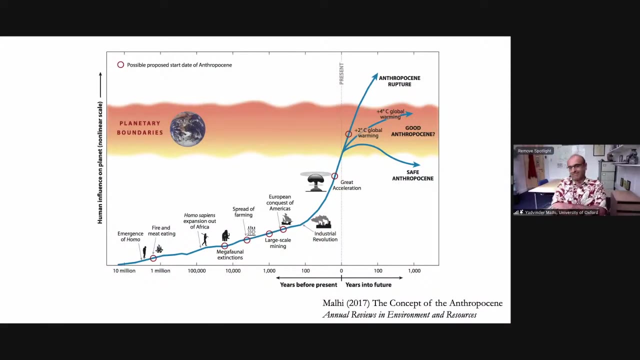 realization, I think, is the key, I think it's the key, I think it's the key, I think it's the key, The fundamental challenge of sustainability of our times. And this realization has many framing. So one framing that is increasingly popular is this: 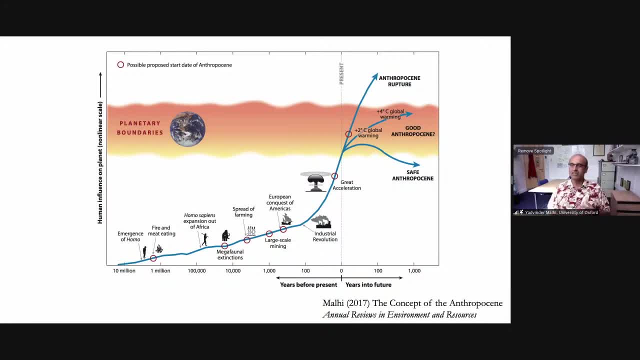 idea that we're entering a new geological epoch, of the Anthropocene, a geological epoch dominated by human activity, And this image captures a broad framing of this idea of the Anthropocene. that human influence on the planet goes back a long time and has a and has been increasing over time. 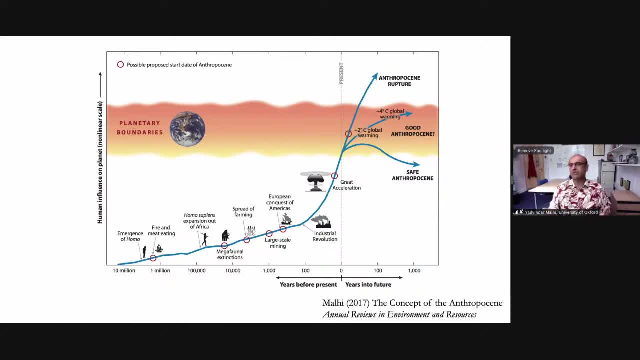 But really over the last century there's been a great acceleration of human influence to the point that it's beginning to hit what are termed planetary boundaries And there's a danger that we'll rupture and pass a significant number of these planetary boundaries and tip the entire system into a fundamentally altered state. 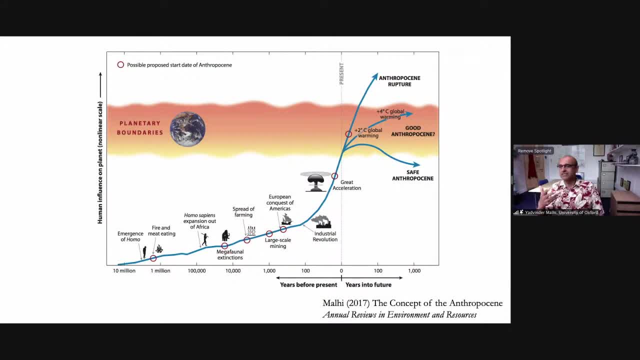 that is very difficult to survive in or very different from the state that we have grown up in as a civilization throughout the Holocene. And that boundary can be around climate, but it can also be around biogeochemical cycles. It can be about the biodiversity web of life. 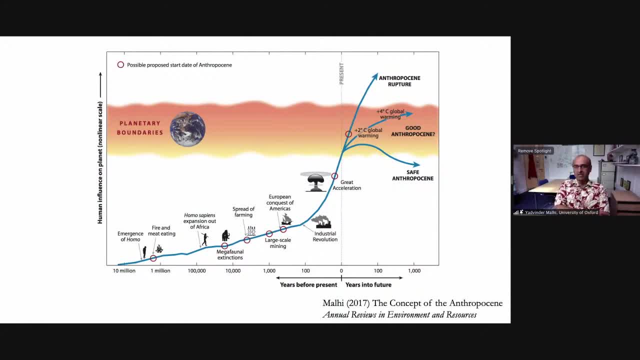 that sustains all life on Earth. And so, for the next few slides, I want to explore one way of thinking about that. that blue line in this chart, In this particular diagram. we have it without any particular axis or label. but for the next few slides, 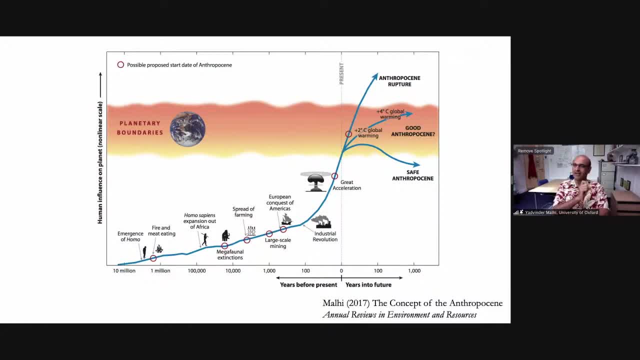 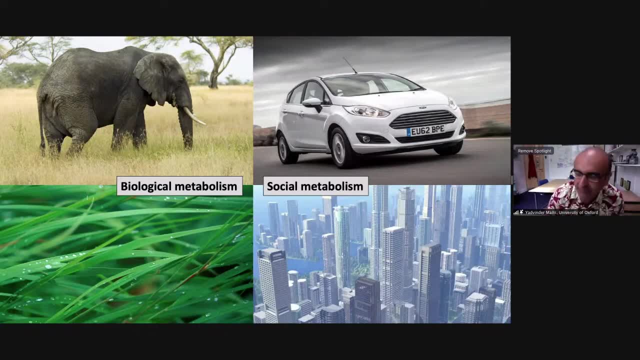 I'm actually going to put a number on that blue line and one possible way of thinking of that blue line over time and conceptualizing it, And this is through the idea of metabolism. Now, all biological organisms have a metabolism, the energy that flows through us. 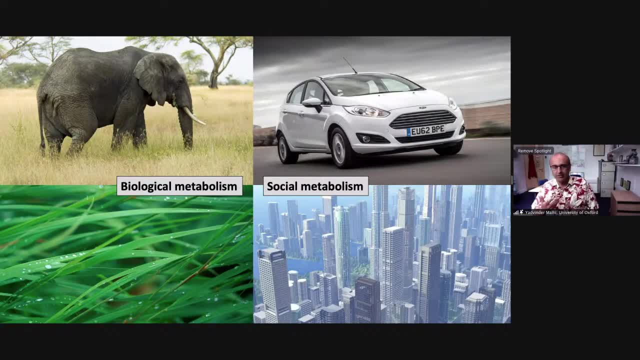 that enables us to function as living organisms, whether we're animals or as plants, have a metabolism as well. But a broader concept that is used is the idea of social metabolism, that as social entities and technological entities, we have a much wider use of energy that sustains us as modern human beings. 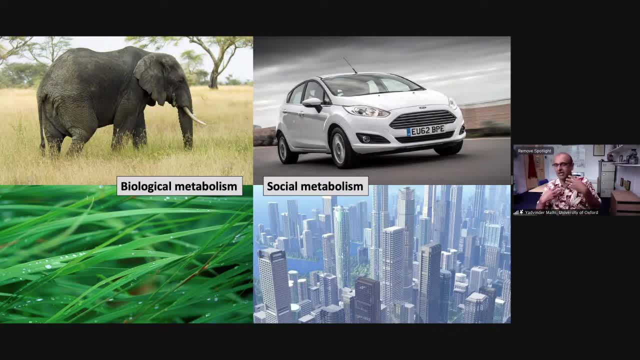 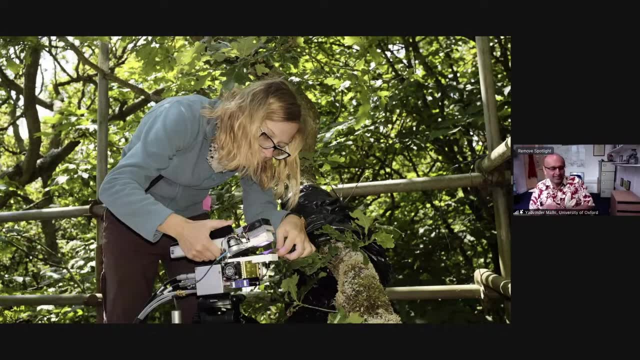 That's embedded energy in things such as our infrastructure, our transport systems, et cetera, And we can make biological metabolism. We can measure. this is a former student of mine, White and Woods, measuring the metabolism of a leaf, And we can scale this up through measurements. 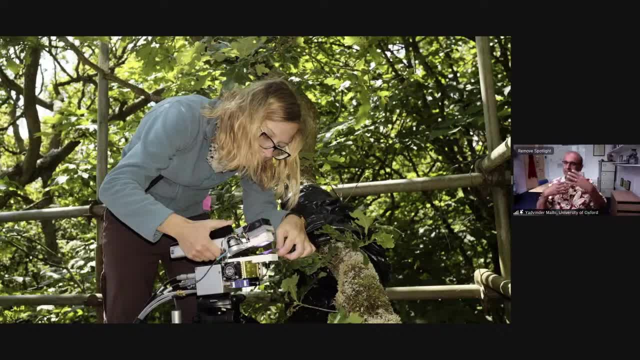 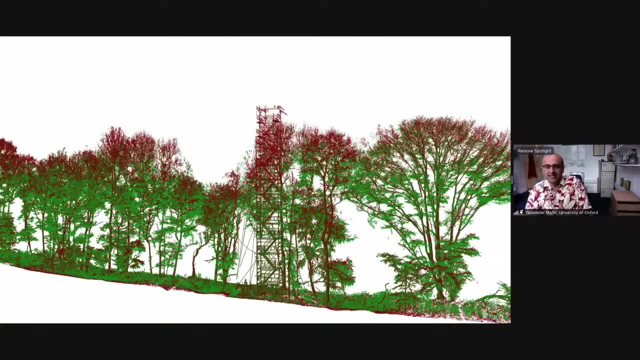 of forest scale and satellites and models and come up with the metabolism, the biological metabolism, of our biosphere, the amount of energy flowing through the biosphere. This is the 3D laser scan of our work at Boynton Woods, just outside of Oxford. 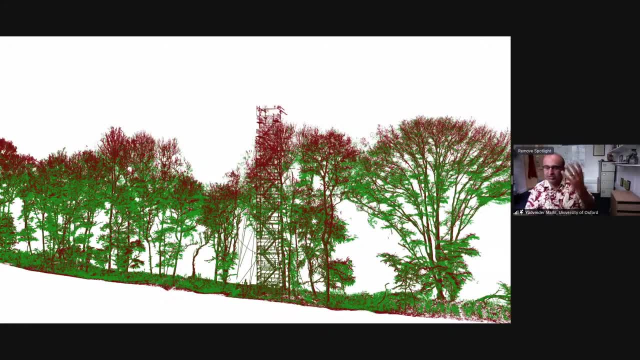 which shows a tower, on top of which we have instrumentation that can measure the flow of carbon dioxide and water in and out of the canopy of Boynton, and we can measure the metabolism of that woodland and how it's responding to local change and to global change. And so a question: 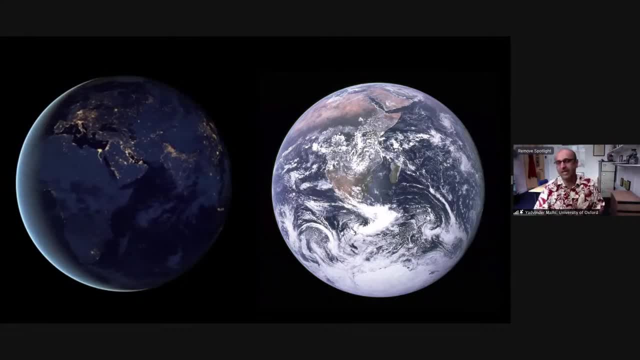 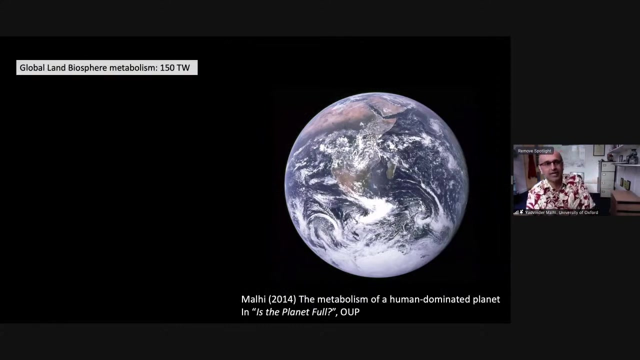 we can ask is: how large is the biological metabolism of Earth and how does that compare to the human social metabolism, not just now but throughout human history and also into the near future possible scenarios for this century? And so if we can calculate the metabolism of land, the biosphere on land is around 150. 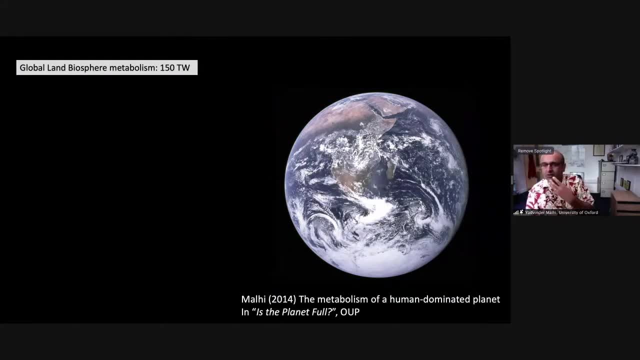 terawatts, the total mass of energy flowing through life on land. So how much energy is flowing through humanity? If we go back 10,000 years to this early Holocene, we can estimate population density and energy consumption by hunter-gatherer lifestyles, and it's about 0.002% of the energy that's flowing. 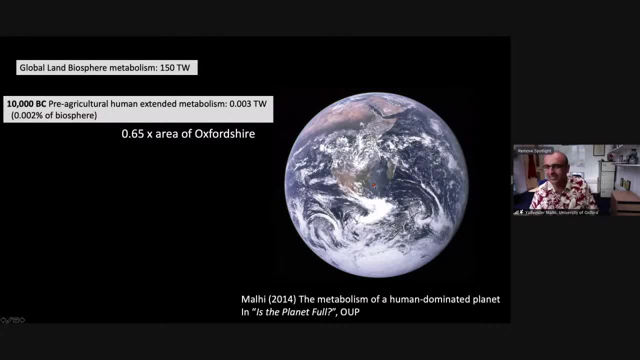 through the biosphere. So all already exaggerated to have this little red dot in the center of this planet. So that sort of represents, rather overemphasized in this case, the size of the human metabolism compared to the whole planet, which is the size of the planetary land surface metabolism. And 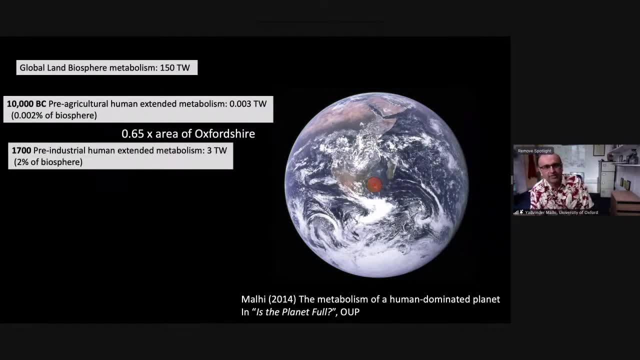 if we go to around 1700, the pre-industrial human metabolism, we see that that circle has grown larger to be around 2% of the circle of the biosphere metabolism. If we go so, as I said, the bit reconfirmed. 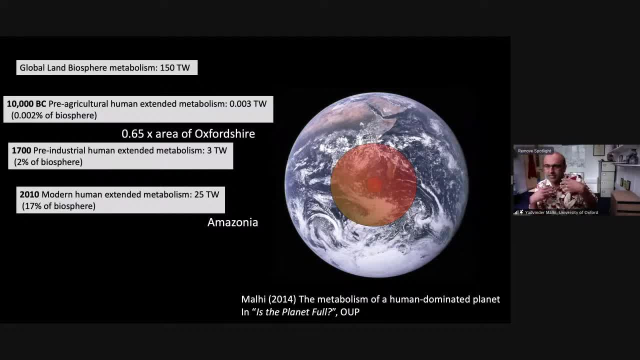 10,000 years ago the entire metabolism of humanity was equal to the biological metabolism of woodland and around half the area of Oxfordshire, just to give you a relative scale As we go to modernity. modern human industrial metabolism is around 17% of the biosphere metabolism, which is roughly the. 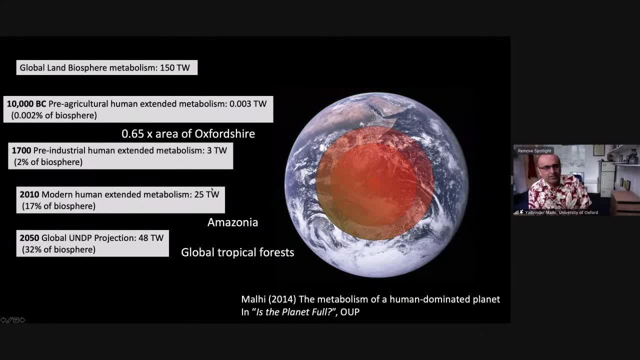 same amount of biological energy flowing through the Amazon tropical rainforest. If we go into the near, If we go under the UNDP projection- typical projection for 2050, this metabolism has increased to 32% of the biosphere metabolism. If we go to a global China where everybody on Earth has the same per capita energy consumption, 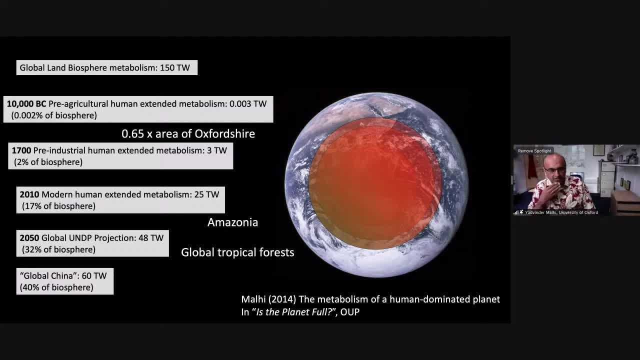 as the average Chinese citizen today. that's at 40% of the biosphere, And if you go to a global USA, we hit 120% of biosphere metabolism. And why does this metabolic comparison? why is it interesting? It is partially because the metabolism has a direct impact on the planet, but also it's 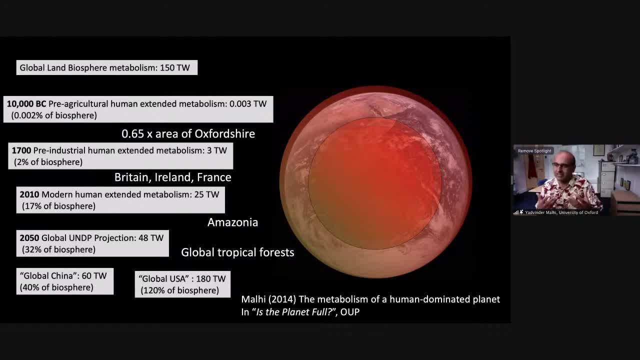 our capacity to do work to alter the planet around us, And what this shows us is that it is this blue line that, in that previous graph I gave you. it gives an idea of how large humanity is compared to the planet that sustains, and 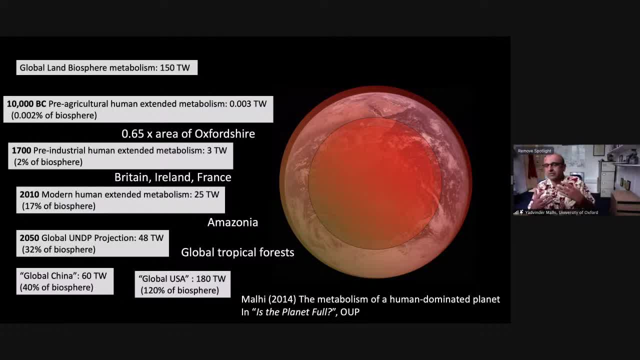 supports us And clearly we're approaching some sort of fundamentalism. When we have a metabolism that's larger than the metabolism of all the rest of life on Earth, there are limits and challenges that emerge from that. But even now, when our metabolism is at 17% of that, profound challenges and one species. 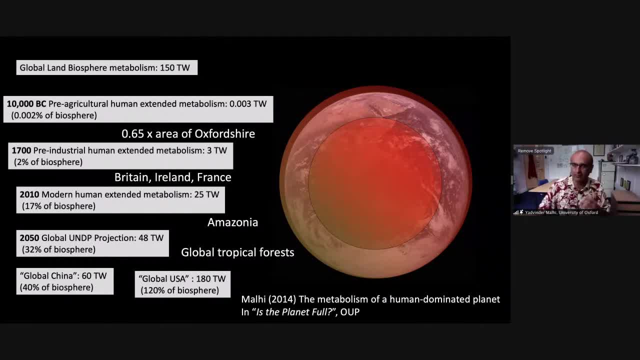 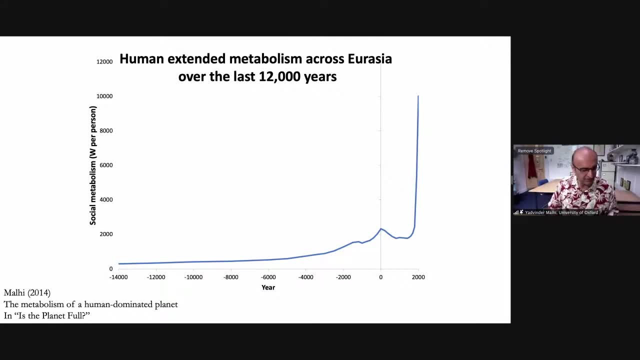 is producing 17% of planetary metabolism and there are profound challenges associated with that. We can see how this has changed over time. this metabolism. If you look over the Holocene, we see a gradual increase As agriculture expanded and intensified- an interesting potential plateau since the Roman. 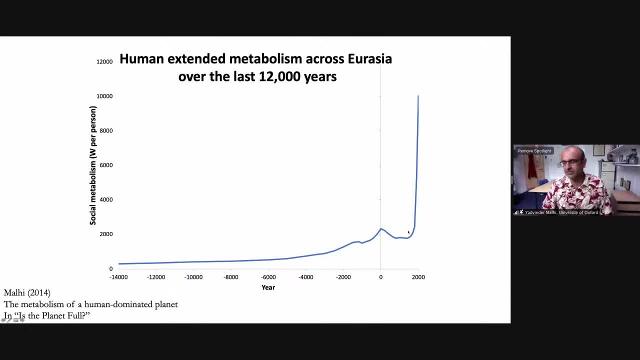 Empire and Han dynasty for the last 2,000 or so years. I haven't got time to go into the speculation around that. But then this surge of metabolism that occurs since the Industrial Revolution- And you can see this line- is shooting almost vertically off this chart. 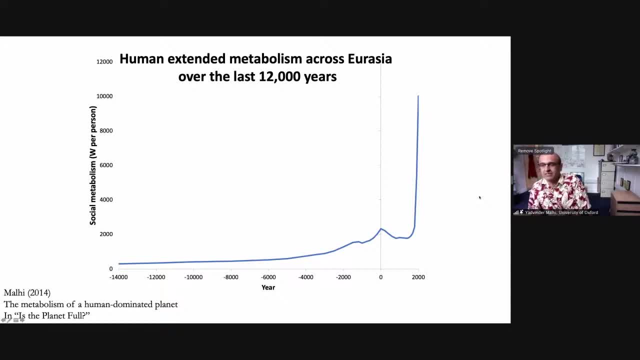 And one of the laws in Most biological or physical systems is that lines like that cannot persist for long before feedbacks kick in, whether involuntary feedbacks or, in our case, potentially conscious feedbacks- to try and alter the trajectory there into something that flattens out. 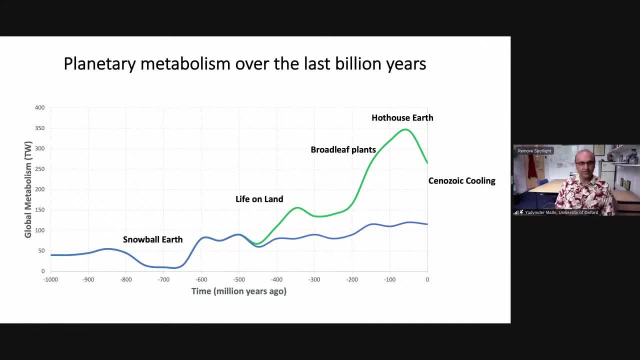 We can take a larger scale. look at this question as well. So here, 10,000 years wasn't ambitious enough. So here we have a look over the last 1,000 million years at the metabolism of life on Earth, And this is very speculative. 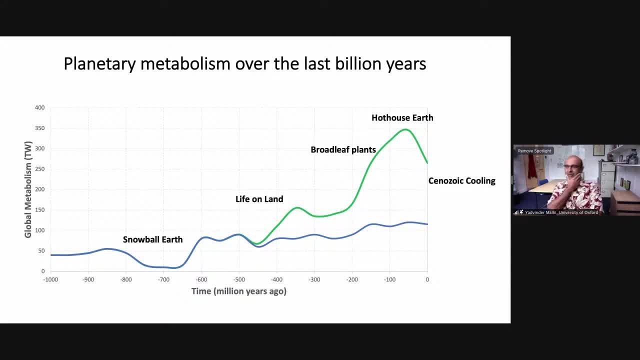 So I'm sure if there are any scientists listening on here they probably have niggles about this and suggest alterations to this, But this gives us the broad pattern of how the metabolism of life on Earth might have varied over the last 1,000 million years. 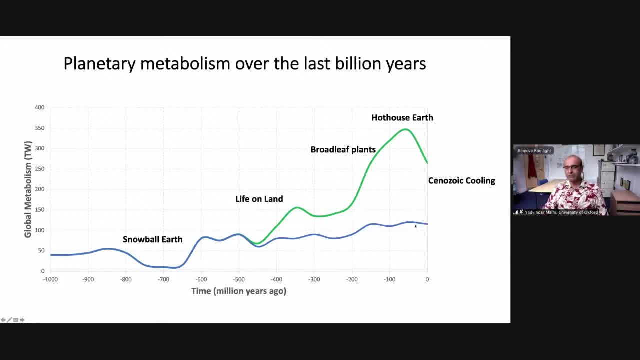 And what we see is periods of low metabolism. Blue is the marine metabolism. So until around 450 million years ago the entire planetary metabolism was marine. And then we see life on land expanding. There's the Green Line And we see this increase in total metabolism where an energy source that was previously 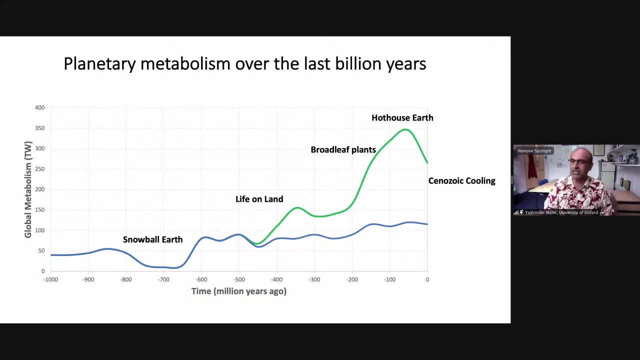 unavailable to life, which is all the abundant solar radiation available on land becomes available. And it becomes available because the biosphere cracks the trick of how to access and retain water on waterless land surfaces, And that enabled this expansion of the biosphere, this increase of metabolism that peaked in 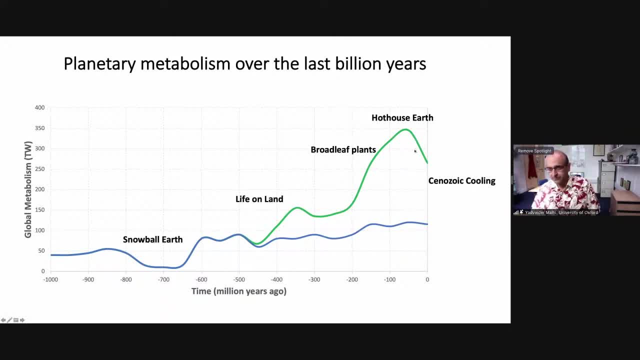 the late Cretaceous, And then we see the evolution of the biosphere to the Eocene period and under much warmer conditions, and then it's been gradually decreasing as the Earth has cooled over the last 50 or so million years. And one thing that we can do with this metabolic framework is compare the energy flow through. 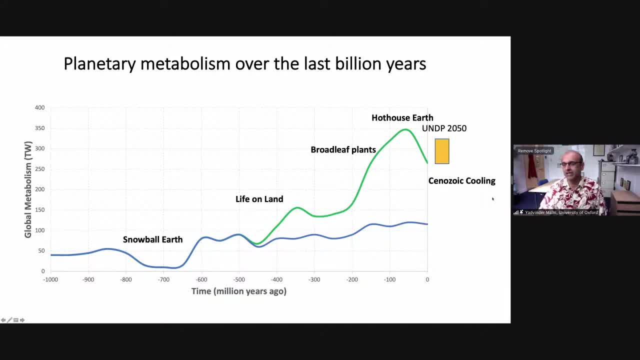 the biosphere through Earth history, with the energy flow now and in the future through humanity. So if we go for that UNDP mid-range scenario, what's the total amount of energy flowing through the biosphere? Well, we can see that the energy flow is much larger than it should be compared to this. 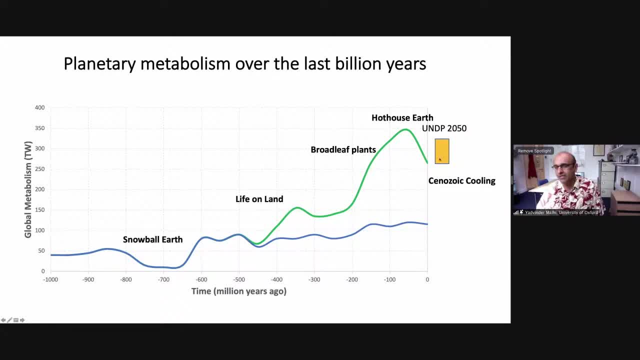 global Earth system picture And we see that it's significant. It's on the order the increase of energy flowing through the combined human biosphere system and we are embedded within the biosphere, We are part of the biosphere, We are part of nature. 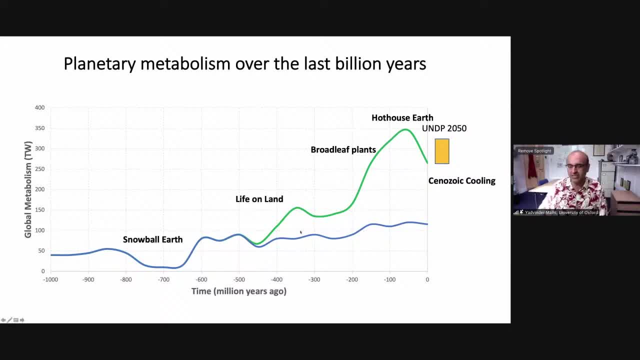 And combined energy is similar to the transition that occurred with the advent of life on Earth, And if you go for the extreme global North America scenario, we see it's much, much larger than that transition. So I guess what this is saying is that the challenge we face is not only significant. 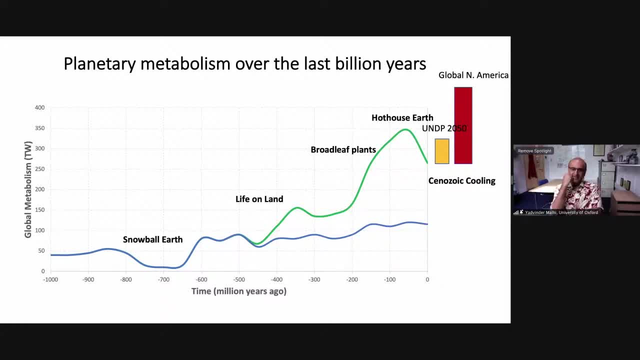 on the timescale of the Holocene, which is often the deep time perspective that we take. but in some ways the Anthropocene is a rather immodest description of the challenge that we're facing, The transition that's occurring in the nature of the biosphere, the nature of life on Earth. 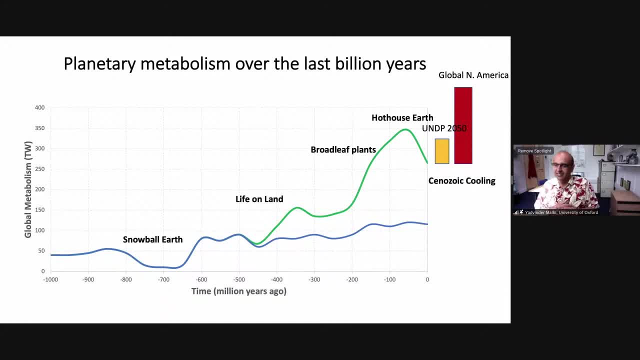 is profound on deep Earth system timescales in terms of how it's altering biogeochemical processes, climate processes- And that's the challenge we face: The nature of life on Earth and the evolutionary patterns of life on Earth. This is one way of capturing how profound this is as an event in the entire evolution. 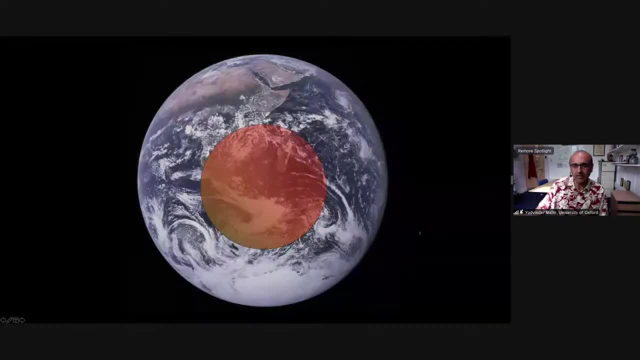 and history, deep time, history of life on Earth, And this metabolism matters for a number of reasons. A large metabolism. I would argue that it's almost the underlying challenge that we face, from which all the other challenges that we have spin off. 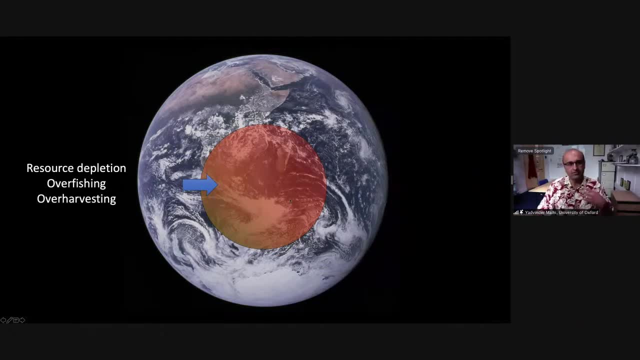 So a large metabolism is hunger. It leads to resource depletion, the challenges such as overfishing, overharvesting of resources- and it produces waste products- metabolic waste products, which lead to climate change, acidification, plastics, human industrial waste and all those challenges. 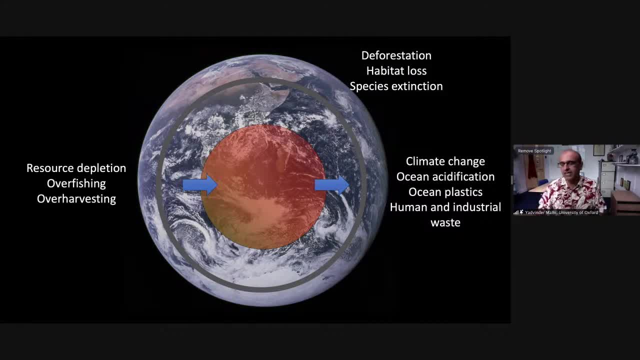 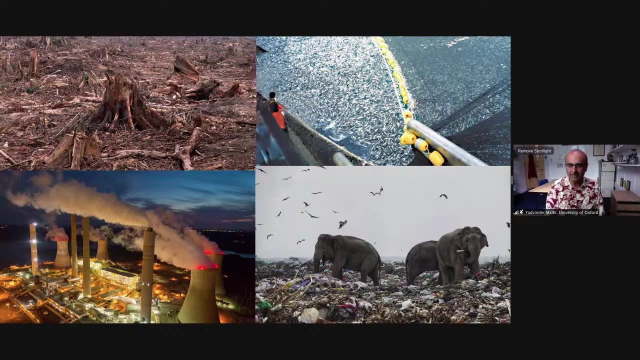 And the metabolism also occupies space and displaces space from other denizens of the biosphere. the processes such as deforestation, habitat loss, species extinction, And so a number of the challenges that we face around sustainability, fundamentally spin off from the challenge of this large and entangled metabolism, entangled with the other processes. 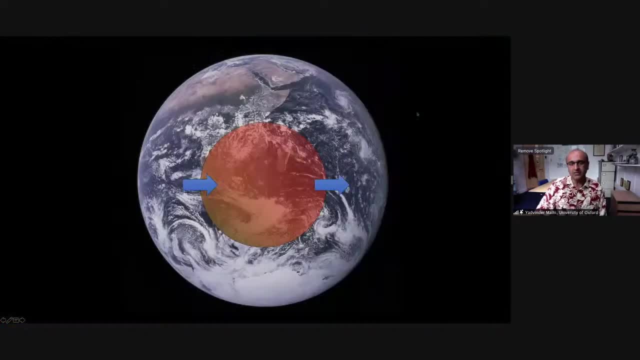 of the atmosphere and the biosphere, And so, to address this, there are two ways that we need to think about limiting the impacts of this metabolism on the biosphere. One is to re-stabilize the growth of this metabolism so that it doesn't keep on expanding. 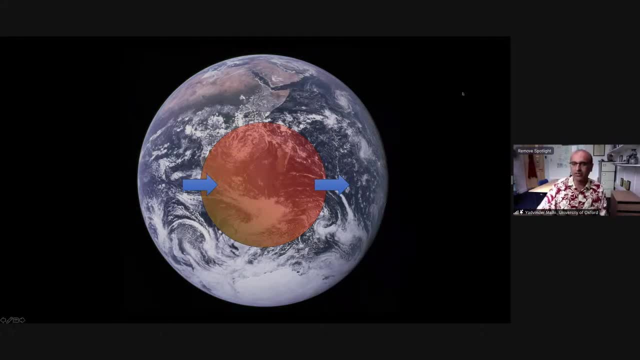 And the other is to stabilize the growth of this metabolism so that it doesn't keep on expanding, And the other is to re-stabilize the growth of this metabolism so that it doesn't keep on expanding and encroaching on the biosphere. 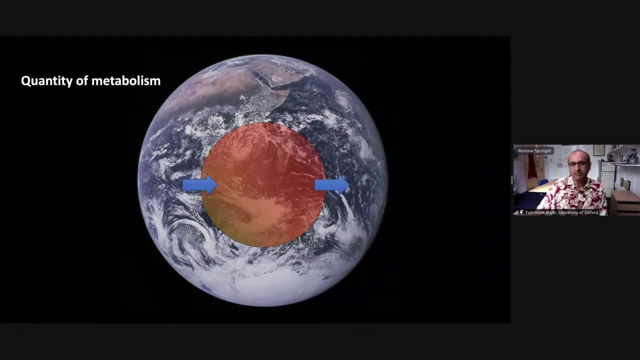 And that's the quantity of metabolism. But the other one is: the more that we can make this metabolism circular, the more we can decouple this metabolic activity of the metabolism from the planetary metabolism, the less impact it has, outside of its boundaries, on the surrounding planetary metabolism. 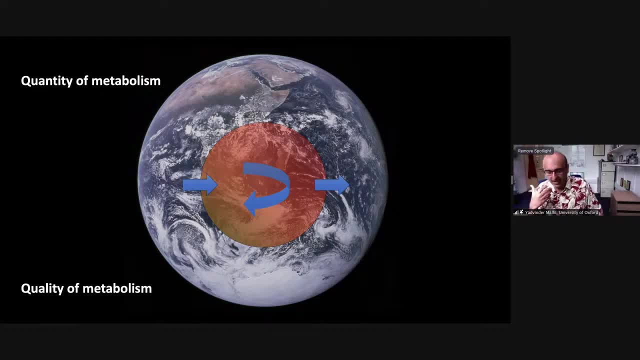 So processes such as renewable energies that have less waste production, recyclable materials, things that make this metabolism circular. So we do have the risk point. the risk point is also the transverse effect, which is to us there's a lot of risk, but we're. 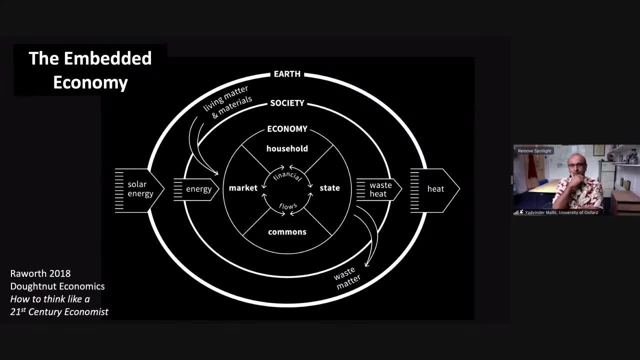 not taking away from this Another way of thinking about this. our colleague Kate Raworth describes the economy as embedded within society, which is embedded within nature. so, rather than society approaching externalities to an economic model of the world, the economy sits within applications, so that the economy 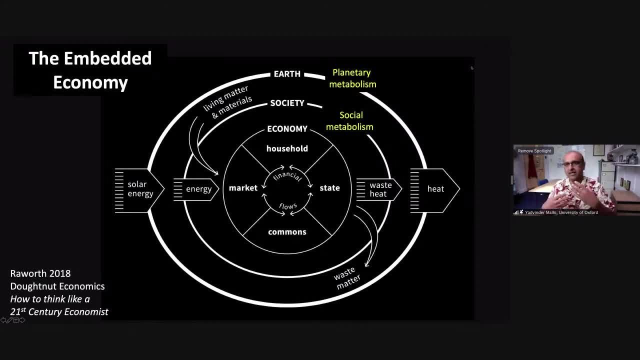 can be partirically taught and motifated, And, as we have the αν be of energy crashes along a pinballticnt's universe, redeeming the, And we can think of the society, the energetics of the society, as the social metabolism sitting inside the energetics of the earth, as this planetary metabolism. 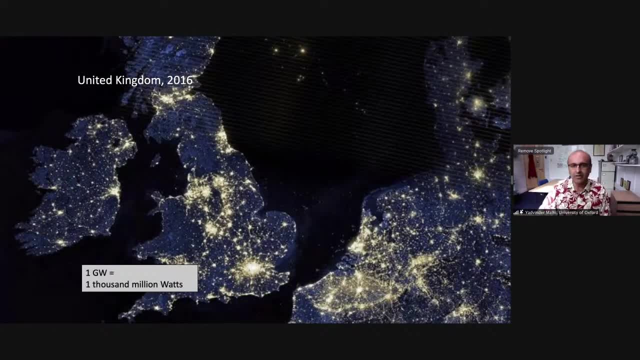 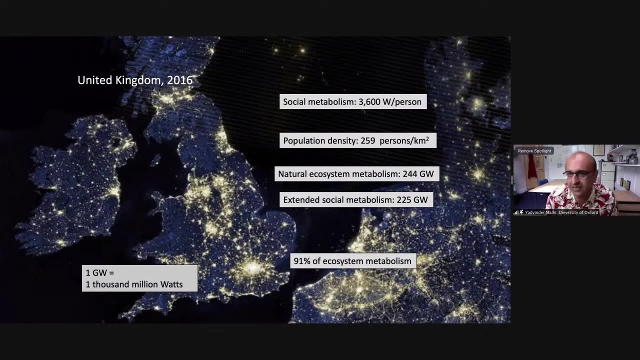 Let's move in, moving away from the global to a local scale. If we look at the UK, I'll just click through some of these numbers quickly- We can do this calculation for the UK as a whole, calculating the per capita metabolism and the population density. 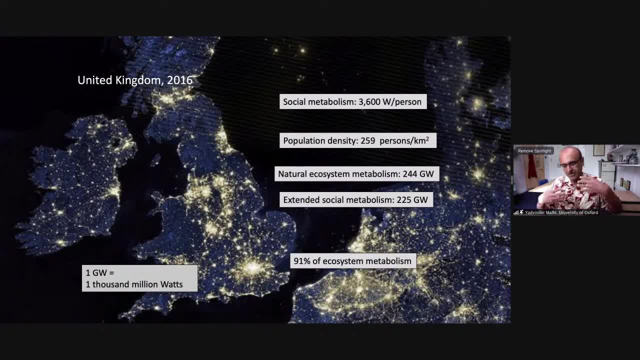 And we see that broadly the amount of energy flowing through society in the UK is roughly the same as the energy flowing through the biosphere of the UK. So we're much closer to 90 or 100 percent of that compared to this 17 percent globally. 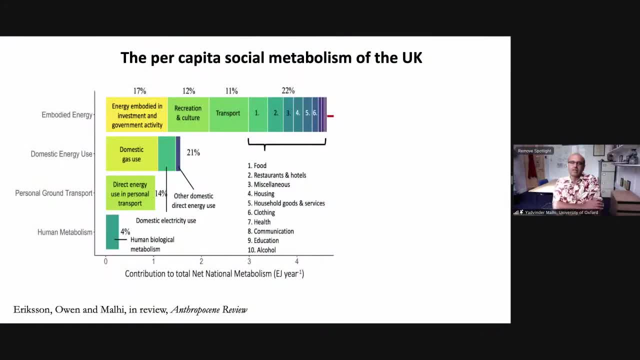 And we've explored that UK metabolism a bit more. This is a work that was led by my former master's student, Frederick Erickson, and is currently in review, where we break down this UK metabolism And we look into its components and look at how much of it is coming through infrastructure, through transport, through energy use, and how much is the biological metabolism. 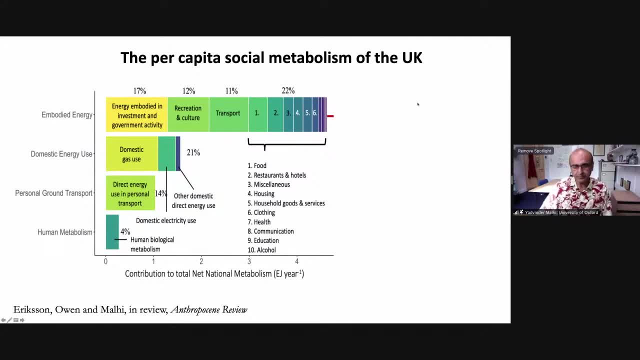 And you can see the breakdown there. But also you can also see how much of that is a domestic metabolism, which is the half of it, and how much of it is embodied metabolism that comes from other parts of the world and the goods that we consume in particular. 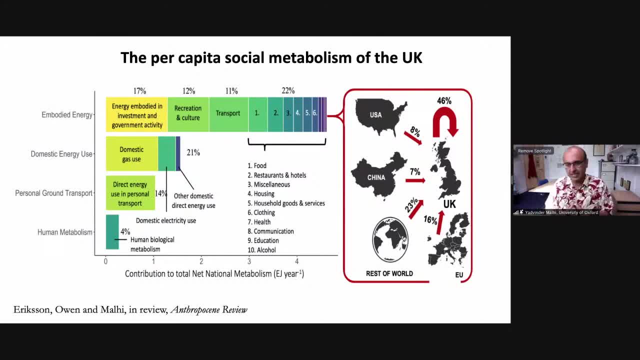 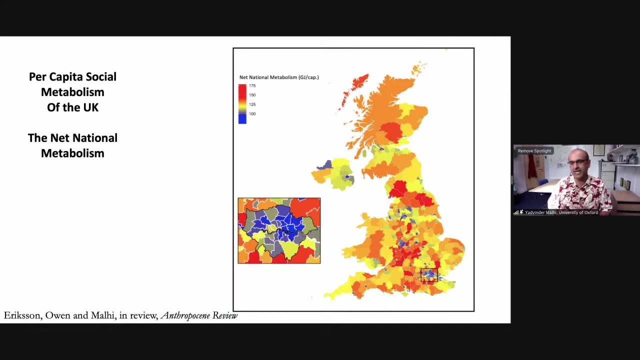 And you see that part of the way that we're able to sustain metabolism And one of the reasons why we're able to sustain such a large metabolism on this small island is that half of our metabolism is imported from other parts of the planet. And also in this analysis, we were able to use data to break down to a finer scale and look at districts and regions within the UK and come up with this image of the per capita metabolism of the UK. 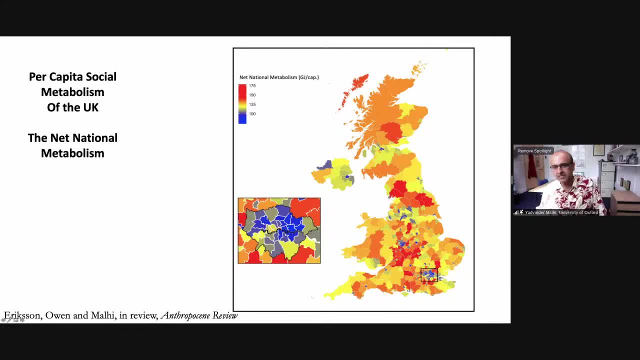 And you can see interesting patterns start to emerge here that we see places such as cities such as London generally having lower levels of per capita metabolism. And you can see interesting patterns start to emerge here that we see places such as cities such as London generally having lower levels of per capita metabolism. 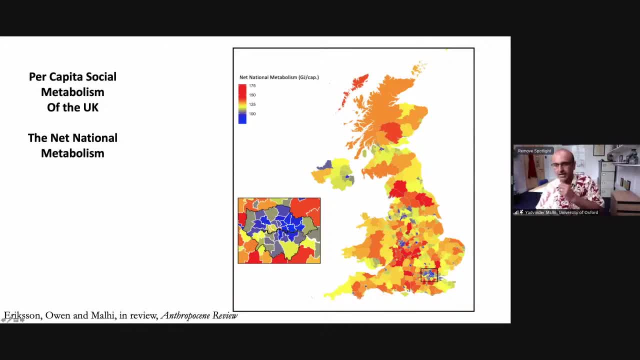 And you can see interesting patterns start to emerge here that we see places such as cities such as London generally having lower levels of per capita metabolism than remote rural areas that have more transport per capita costs, etc. So you see interesting geographical patterns that are worth exploring. 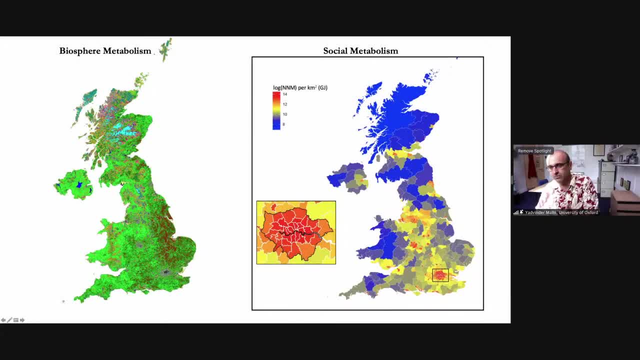 And if we do add a spatial level here, so this is now per kilometre squared rather than per capita. on a logarithmic scale you can actually compare that spatial pattern with the spatial patterns of biosphere metabolism And you can do some interesting analyses. 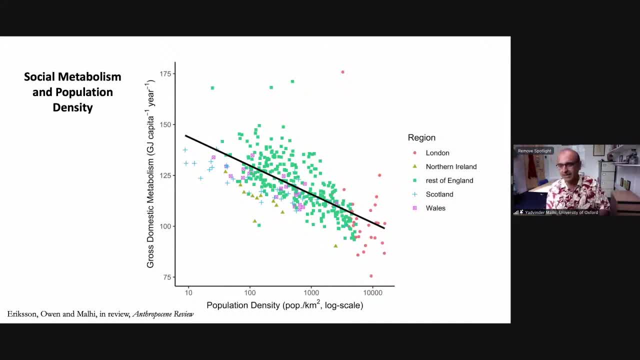 So we can look at the relationship between population and population. So we can look at the relationship between population and population. So we can look at the relationship between population density and metabolism. and we see, the denser the population, the lower the per capita metabolism. arguing that cities are very efficient ways. If you're going to have a lot of people on this planet, cities are very efficient ways to have those people, more than pretty suburban or rural areas, because of infrastructure gains, of housing efficiencies, etc. So the per capita metabolism is often lower in densely populated areas. If you're going to have a lot of people on this planet, cities are very efficient ways to have those people, more than pretty suburban or rural areas, because of infrastructure gains, of housing efficiencies, etc. And we can also look at other relationships. 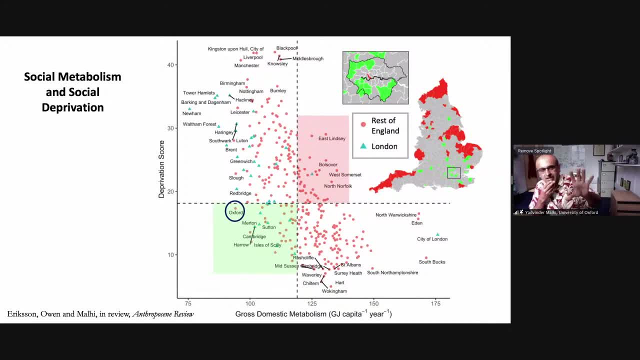 So here we plot deprivation For England only. we have deprivation scores for each region against per capita metabolism And you can see overall there's a broad negative correlation. So the less deprived region is generally the lower the deprivation. So the wealthier areas in the bottom right here tend to have lower deprivation and higher per capita metabolism. 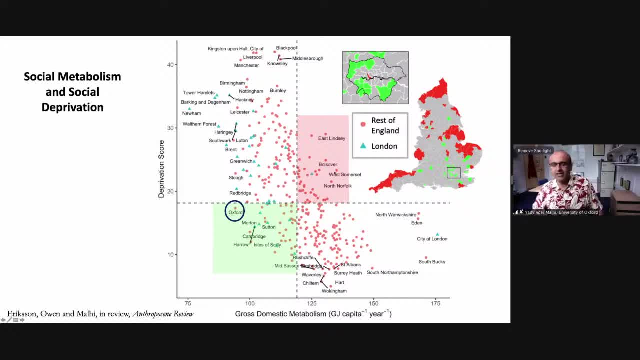 And vice versa in the top left. But beyond that, I think what's more interesting is the variance in this diagram over the overall trend. There are areas here that have relatively lower metabolism and low deprivation and areas that have relatively high metabolism and high deprivation. 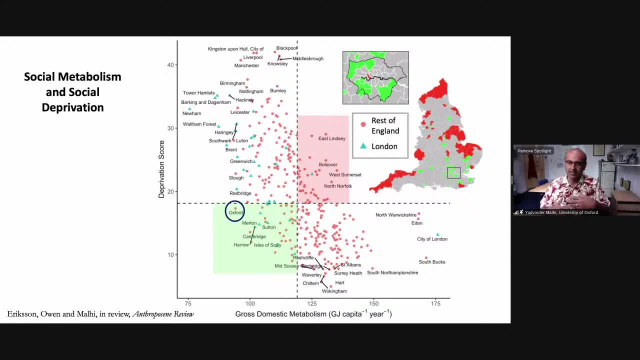 So where is the potential to nudge this while reducing deprivation, while not increasing the metabolic footprint? And here we are. in the map. We've highlighted areas that are red, which have a disproportionately high level of deprivation for their metabolic footprint, And in green areas they have a low level of deprivation for their metabolic footprint. 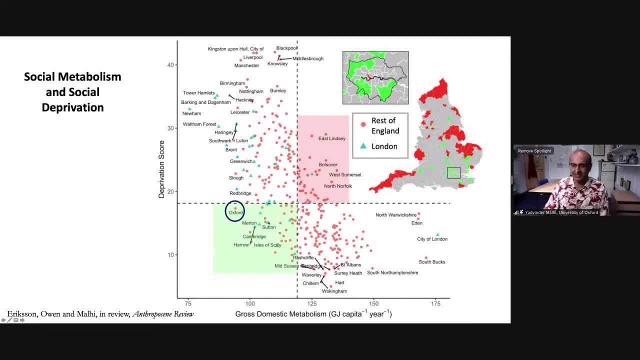 So Oxford actually comes out kind of interesting in this bottom green here. I think part of that is geographical accidents, As a city with a large student population from relatively privileged backgrounds quite often has quite low levels of deprivation but a low overall metabolic footprint. 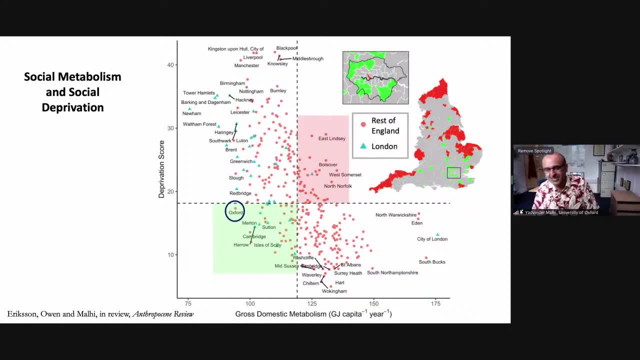 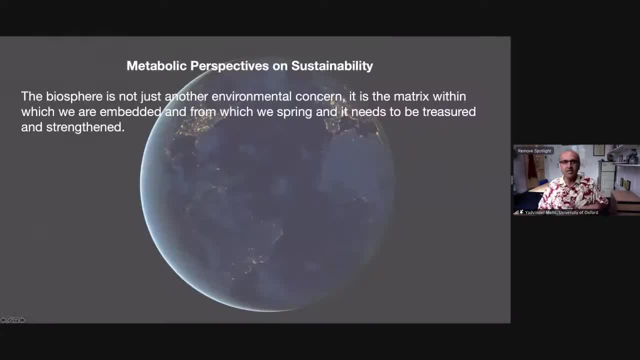 Right. So I think if you can't draw too many conclusions and satisfaction from that alone, but there are interesting patterns here that can be explored and discussed further, And so, in terms of the broader perspective on sustainability, there are a number of insights I think this metabolic perspective can give. 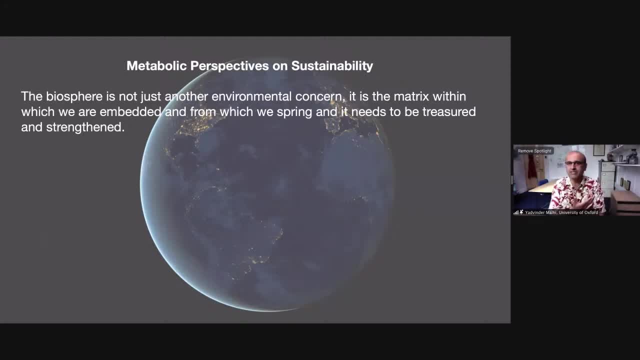 Firstly, the biosphere is not just another environmental concern. It's the matrix within which we are embedded and from which we spring, And it needs to be treasured and strengthened. This isn't just another externality that we need to consider. It is 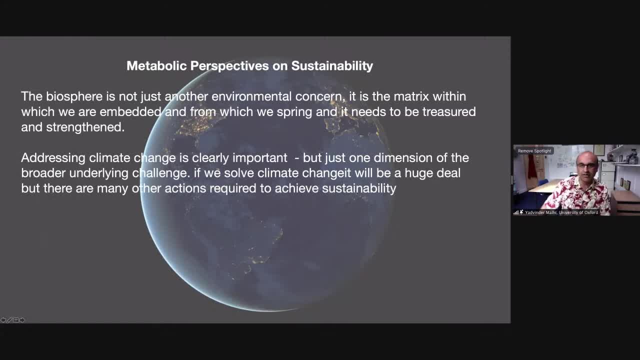 It is the matrix that embeds us and from which we emerge. Addressing climate change is clearly important, but it is just one dimension of the broader underlying challenge. If we solve climate change, it will be a huge deal, But there are many other actions required to achieve sustainability. 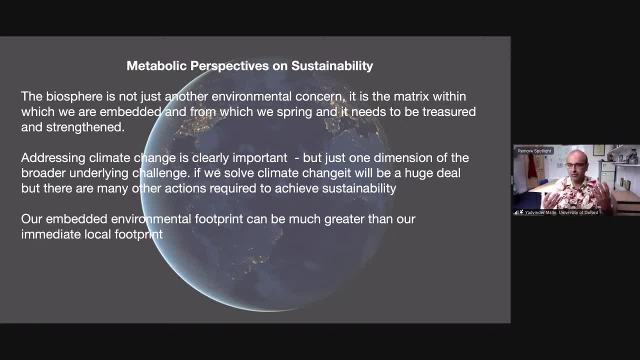 And our embedded environmental footprints. this external footprint can be much greater than our immediate local footprint. So we have to think about that embedded footprint And I think that's one of the insights that's come from the analysis that's gone into the sustainability strategy that many of our impacts, say in terms of biodiversity, are much more about an embedded footprint than in our local land footprint per se. 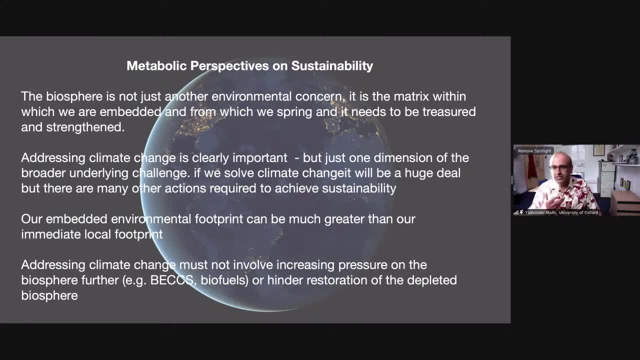 And addressing climate change must not involve increasing pressure on the biosphere further. The biosphere already is challenging enough: meeting food demand and supporting the rest of the biosphere And the variety of life on Earth. And if we come up with actions that increase pressure on the biosphere through biofuels or BECCS or other strategies, or hinder restoration of the depleted biosphere, 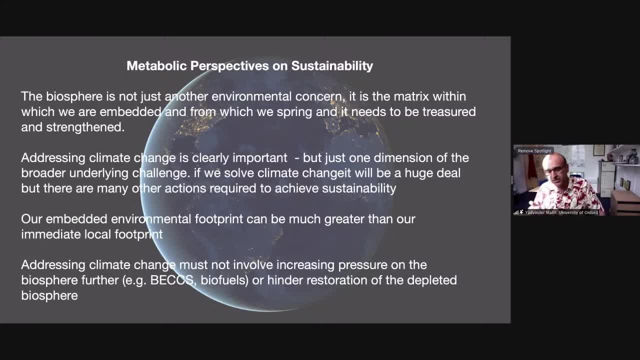 So lands may be degraded, but there's potential to restore those lands rather than saying, oh, they're degraded. Therefore, we can use them for biofuels or other strategies. I think strategies that increase pressure on the biosphere or hinder restoration of the biosphere are things that we need to avoid. 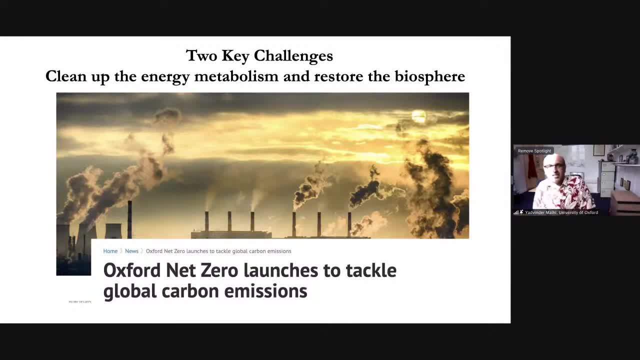 So two key challenges from that are: we need to clean up our energy metabolism and to restore the biosphere. Earlier on we heard from Sam about the net zero initiative and the important contribution the university is making to thinking through how we clean up the energy metabolism. 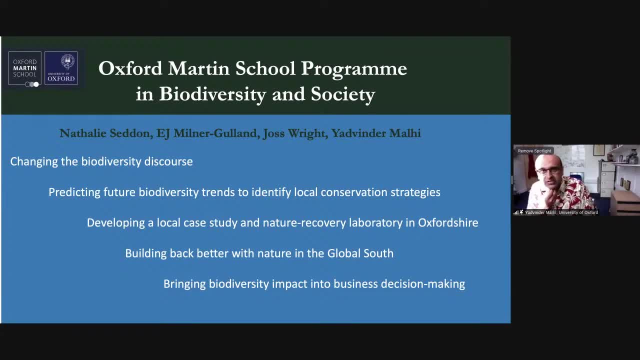 I'd like to mention something else that's also launched this week, which is the new Oxford Martin School programme in biodiversity and society, which is a million pound programme looking at that biosphere aspect. So we're looking at a range of things around the challenge, looking at a range of things around the biodiversity discourse, predicting future biodiversity trends and developing a local case study. 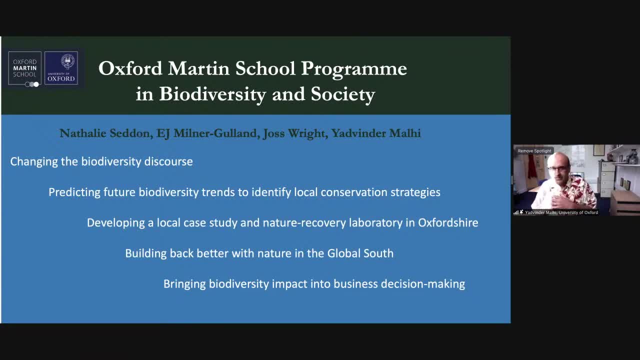 something I'll go on to a little later- building back better in the global south and bringing biodiversity impact into business decision making. So the university is also getting its act together and thinking in an integrated way around the challenges around biosphere recovery and nature recovery as well. 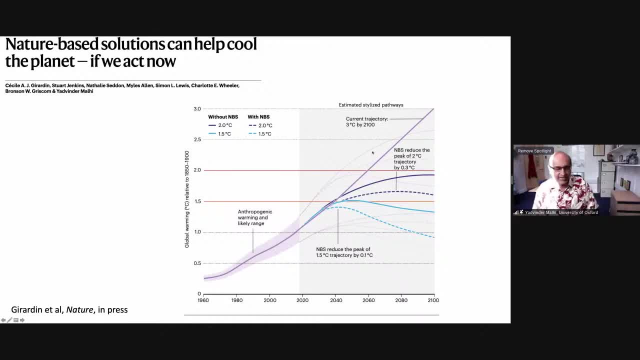 And With this figure I'm probably running into hot water with nature embargo rules, but so be it. This is a paper that I couldn't resist showing, because it combines activity from a range of academics across the university, people like Miles Allen and Natalie Seddon, and Cecile Girardin and myself. 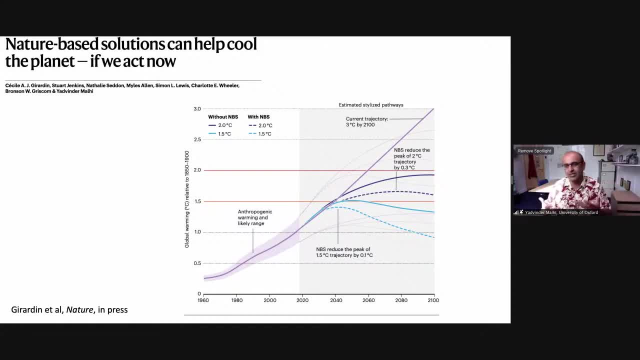 And it shows the type of joined up thinking that is possible when we combine these biosphere and climate perspectives, And this will come out as a commentary in Nature next Thursday. So what we show here is say, for example, the blue line is a 1.5 degrees pathway and then the dashed blue line is an ambitious nature based solutions strategy and how that would modify a 1.5 degrees pathway. 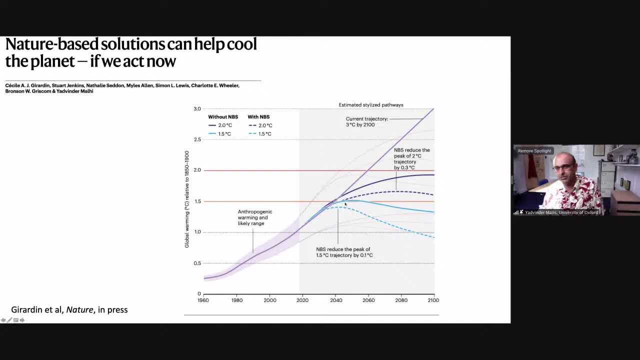 So it has a modest effect on reducing peak temperatures and contributing to that peak temperature goal, but has a larger effect post peak temperatures and the cooling that we may want to address after we stabilise it as a peak temperature. And the darker blue lines show the similar contrast for a two degree scenario, where there's a longer time for nature based solutions to make a contribution and contribute. 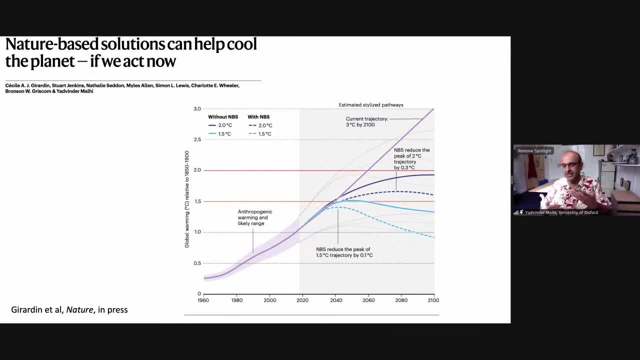 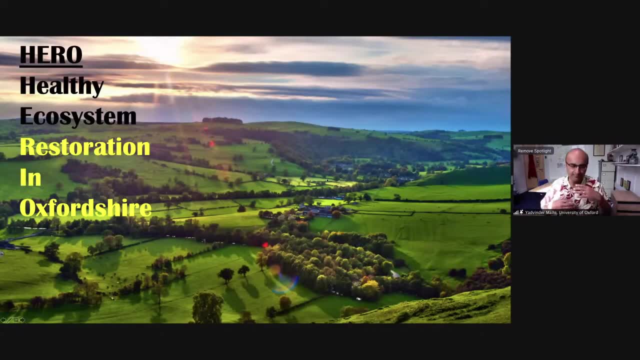 But it shows that sort of joined up thinking between biosphere thinking and climate thinking that is possible when we get our act together. Finally, I'll end with a part of this new Martin School programme which we've called HERO, the Healthy Ecosystem Restoration Programme in Oxfordshire, which is trying to develop this local county and 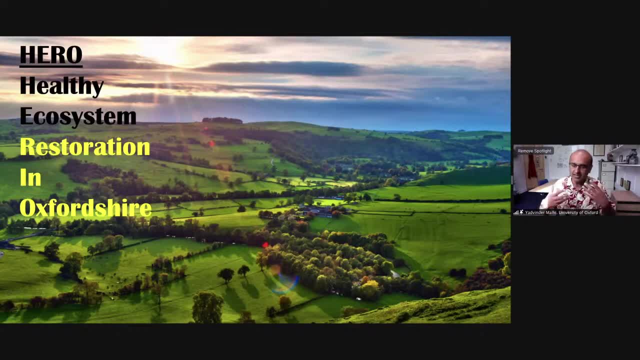 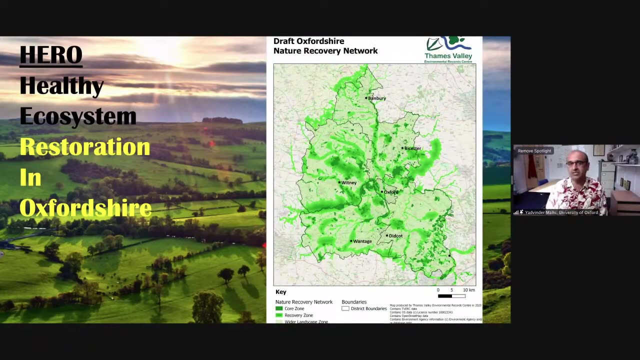 environment as a case study where we can look at a number of these challenges around biosphere sustainability, nature recovery and see how we can deliver on the ground and also provide lessons that can be applied nationally or internationally around this challenge and contribute to things such as the nature. 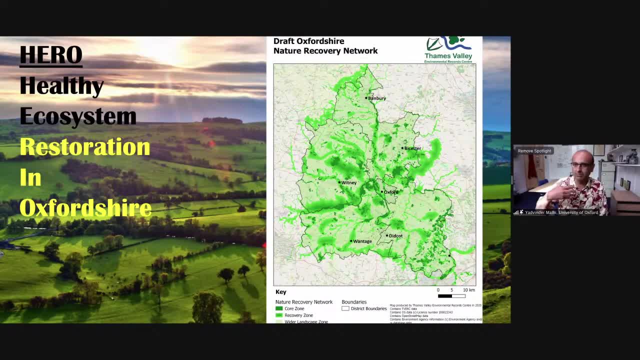 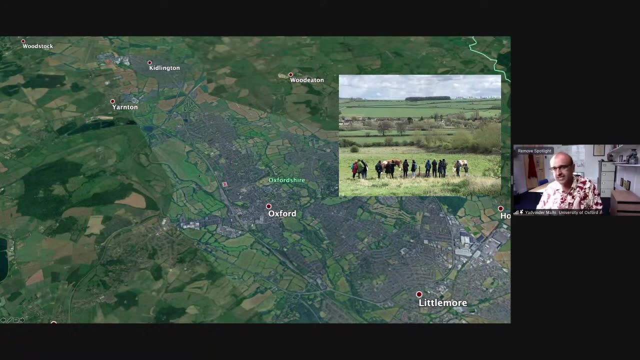 Working with local partners can help design and understand the potential for nature development of a nature recovery network for the county and use this as an example That could be More widely spread. So, in the case of Oxfordshire, how can we look at the landscapes around Oxfordshire and come up with designs in agricultural lands and restoration lands in intact woodlands that facilitate climate resilience, climate adaptation? 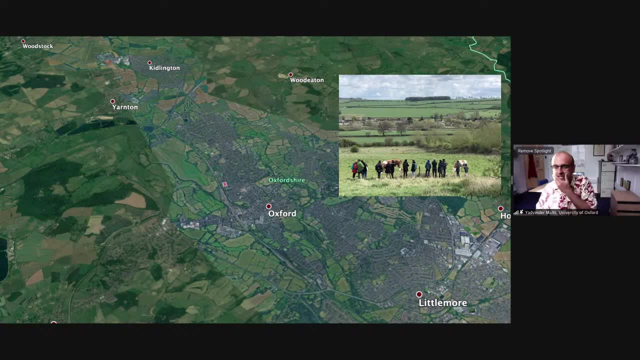 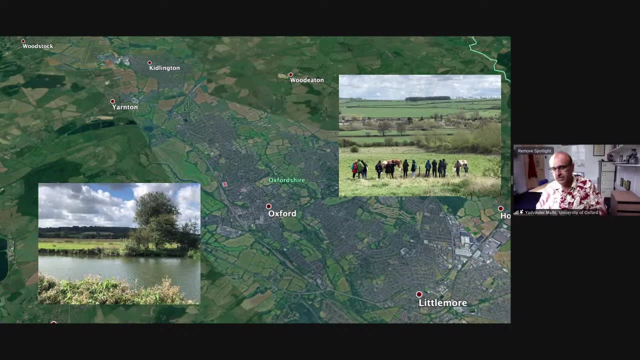 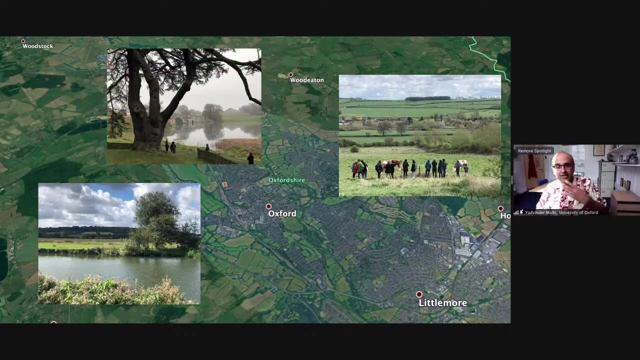 Here we're looking at a flood management scheme in northwest Oxfordshire a few days ago with our students. How can we think about possible nature recovery in part of the university estate or beyond This ambitious project? This project is about the ability of the university to bring back biodiversity into landscapes and working across a whole range of landscapes across the county. 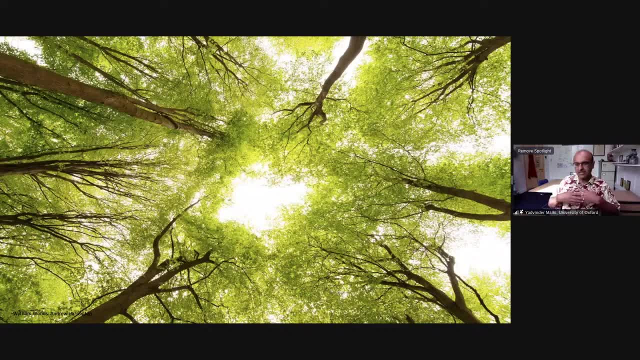 So, to conclude, I think this is a really exciting and important year for both sustainability and for biodiversity. The awareness of nature, local nature, post pandemic, is greater than ever. Appreciation of it is greater than ever. I think previously, until the last few years, biodiversity was a huge part of the current climate change. 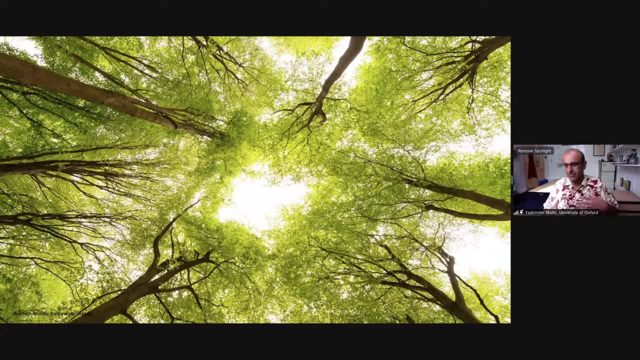 Biodiversity has often been seen as nice to have when we think about global sustainability, And I think now we realize it's both fundamental and critical to the challenge of a sustainable future. And in this delayed super year that Harriet mentioned, we have key international meetings on biodiversity and climate change that will hopefully set the agenda for the next decade. 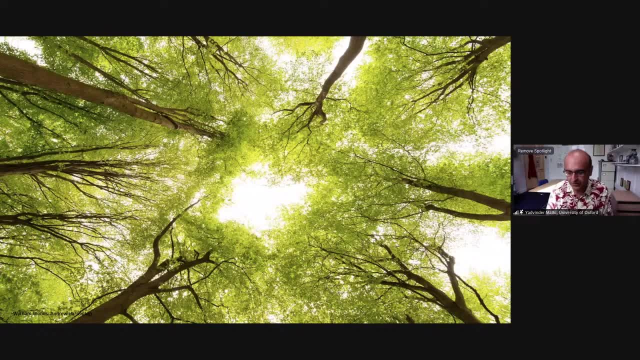 And I believe there's a real opportunity for the university to be at the forefront of events and thinking about how to do this this decade, at scales from global to national, to local And locally in particular. I think what we have here is a chance to really create a sustainable community of practice, embedded in the city and the region and spanning everything from energy to transport, to climate change to agriculture. 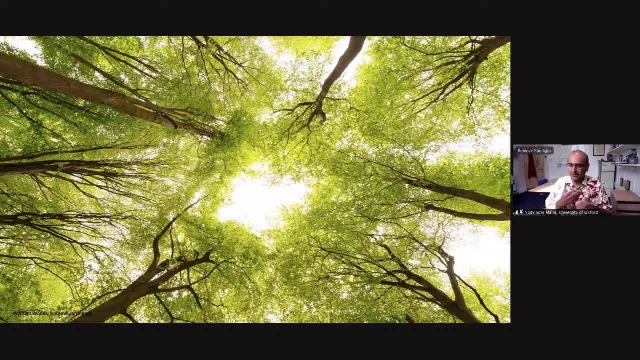 To nature recovery, And I think here I think we can take inspiration from the medics. Oxford Medicine has a global reputation, enhanced even more over the last year, But at the same time that global research is embedded in a local community of practice, where these ideas are tested out for the practical hitting the ground is carried out and explored and understood, 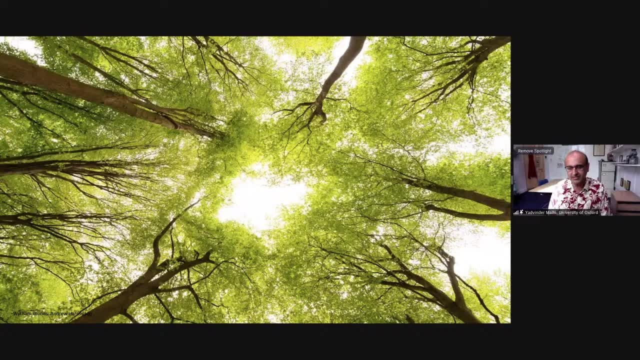 I think we could do something the same with the sustainability. Can we develop a strong local community of practice with our partners where we can look at these global questions and but also have this model case study area where we can develop and think through the practicality of converting from academic thought to practical delivery? 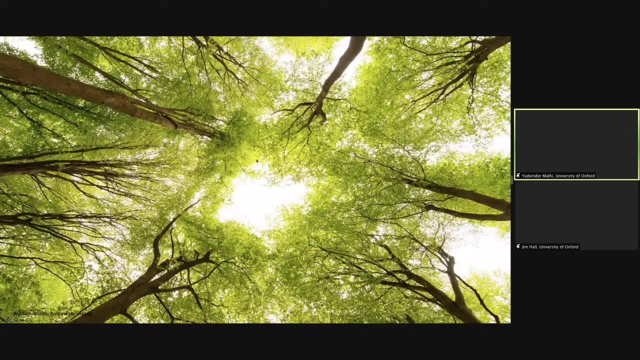 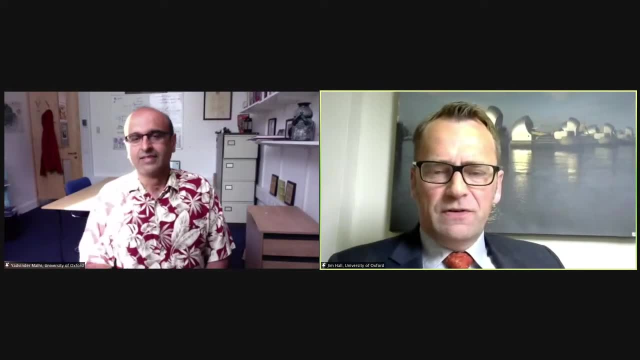 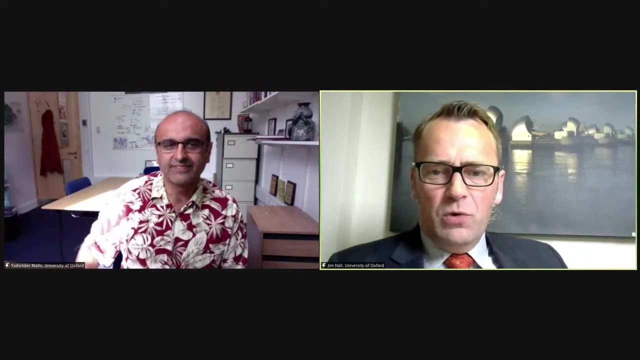 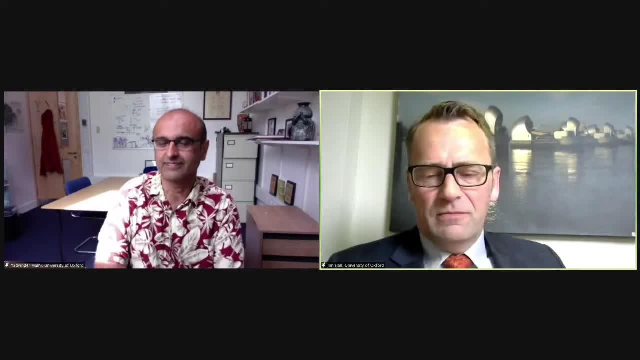 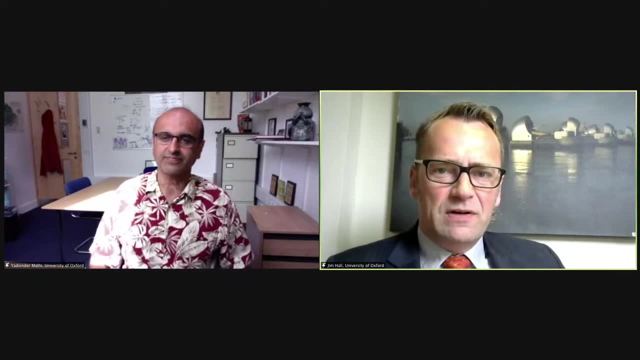 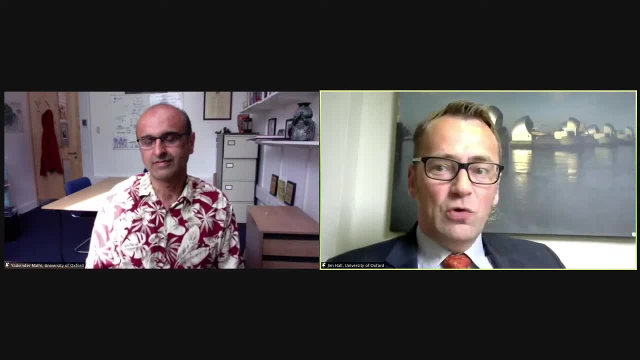 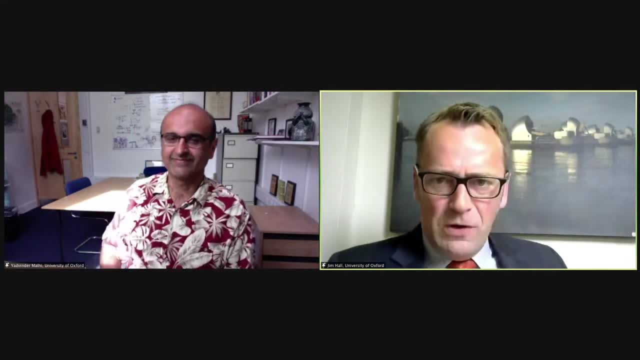 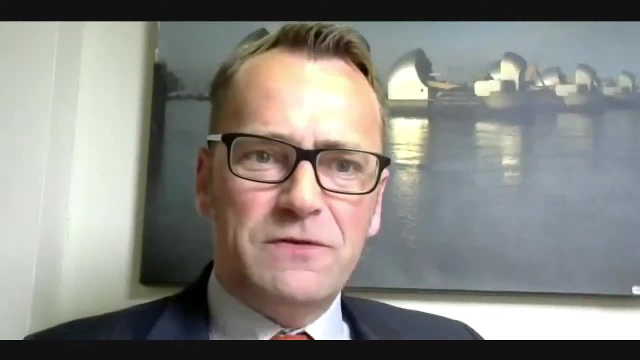 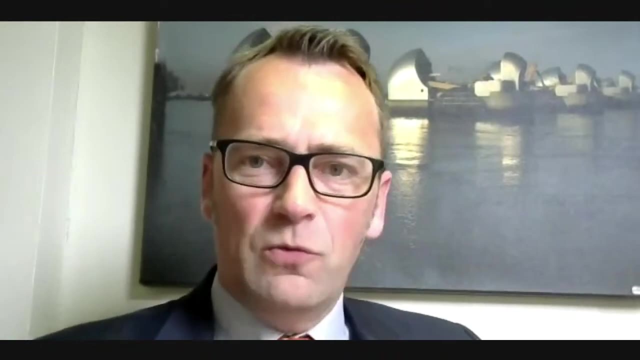 in a fantastic way, taking us from the cosmic and the origins of life back to this small town that we live in. Unfortunately, we don't have time for questions, but we're going to go into our next panel, which has a brief, to reflect further on the. 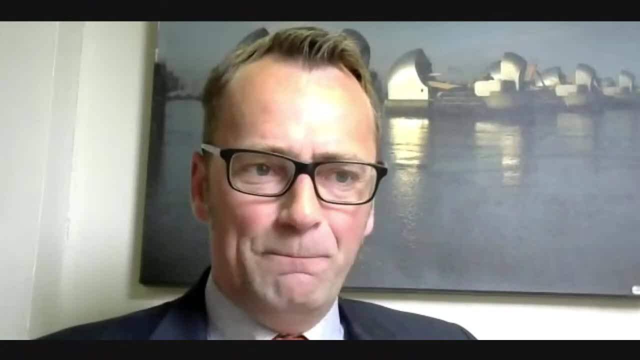 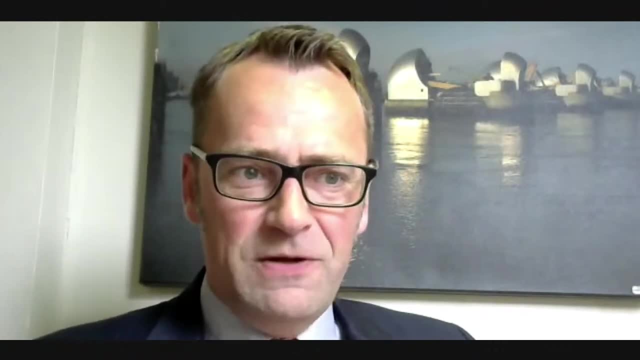 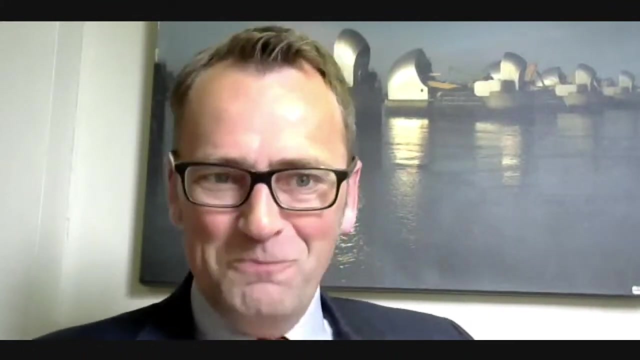 and to look at ways in which we can help to address them And to lead that panel discussion. it's a great pleasure to welcome Fiona Harvey, who many of you will know is Environment Correspondent for The Guardian. Fiona, welcome And thank you for chairing this last panel of the afternoon. 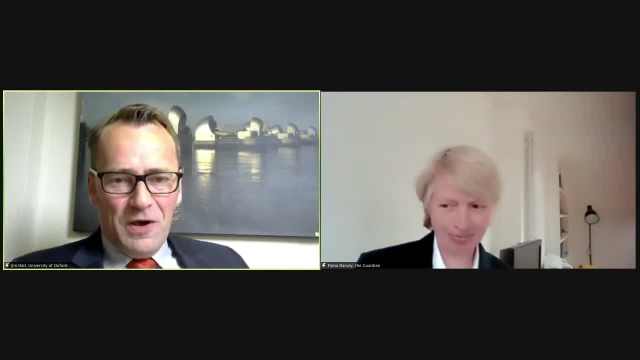 We have until just before 5.30.. You've got questions on Slido And I'm sure you've got some questions up your sleeve as well, And, members of the audience, please keep those questions coming in on Slido Over to you, Fiona. 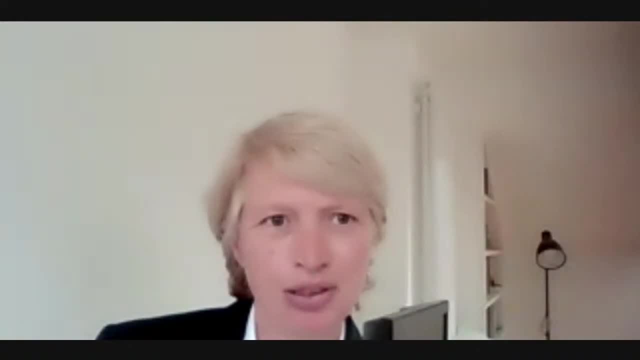 Lovely. Thank you very much indeed. Thank you for that introduction And thank you for that illuminating lecture. Thank you for that. We're going to move on to the panel. We've got a great line-up of panelists for you. 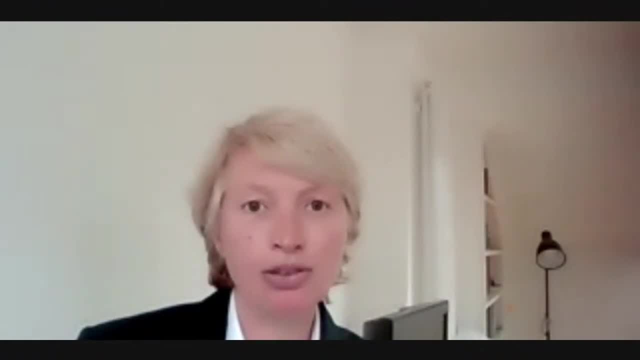 I'll introduce them one by one. I'm going to start them by asking a clear question to each of them To start with, which is: how is the university contributing to local, national and global goals? I'm going to give each of our panelists a chance to answer that question briefly and concisely. 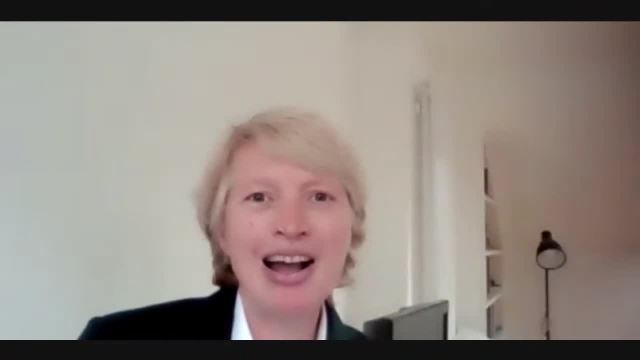 Because this is later on Friday afternoon and we'd like to keep things to time. I'll give them a chance to answer that in a moment. Just to remind you in the audience, please submit your questions through Slido now. Some questions have come through earlier, but a lot of them have been answered in the previous panel. 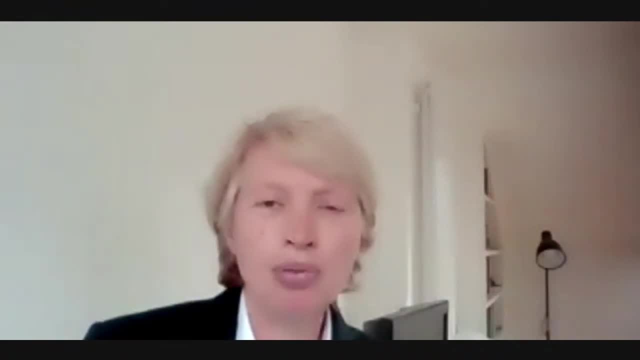 So if you want your question to be answered, please submit it now. Or if you've asked one before, resubmit it so that we know that you want it to be put to this panel. So please do that through Slido now. 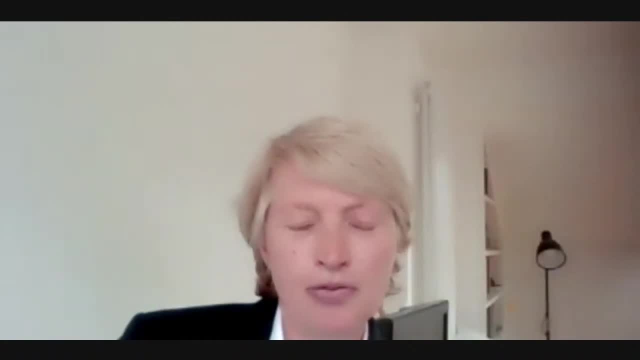 But I'll turn to our panellists for this first question. As I said, how is the university contributing to local, national and global goals? And the first panellist on that will be Cameron Hepburn, who is Professor of Environmental Economics at the University of Oxford. 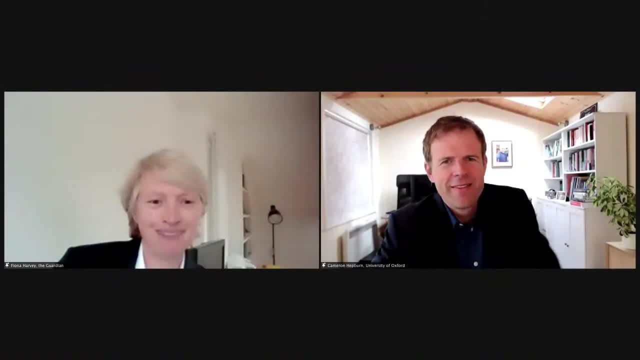 Cameron? how would you respond to that? Thanks, Fiona, Lovely to see you. I'm delighted to be part of this event, So let me give a quick one on each of them. So local, well, I think we've just heard a fantastic swathe of innovations, efforts that we're putting forward as part of the sustainability strategy. 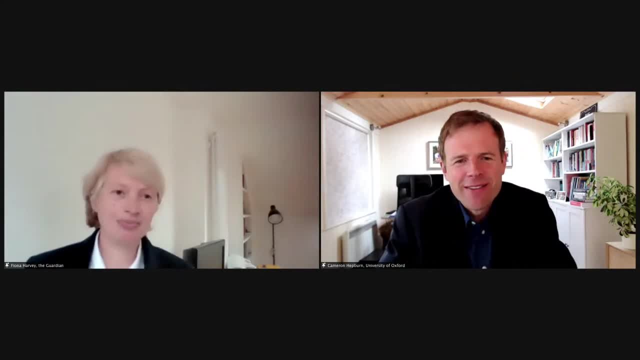 So I won't add to that National I'm here looking at, among others, Claire O'Neill. We contribute to the national meeting of national goals by providing this country with brilliant secretaries of state, among others, But we also provide an awful lot of leadership on the scientific side. 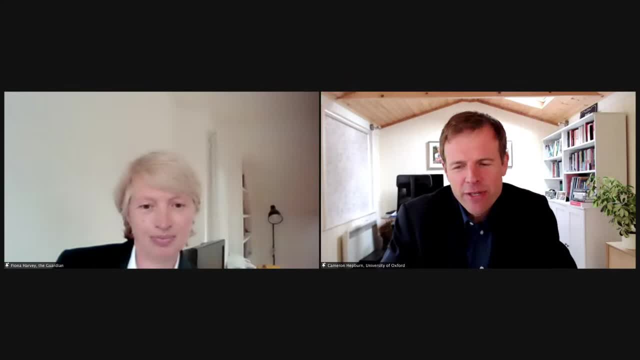 There are numerous challenges. We have a lot of great scientists, chief scientists of the UK government who have and who have been Oxford people And, of course, right now we're providing input into the Committee on Climate Change, getting us to net zero. 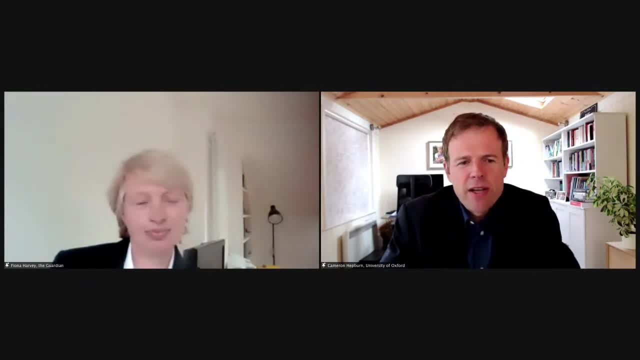 And then, on the global side, Fiona- I just emphasised the amazing science, some of which we've just heard of today- whether it's really in identifying the fact that we have to get to net zero as a scientific, as a physical requirement. 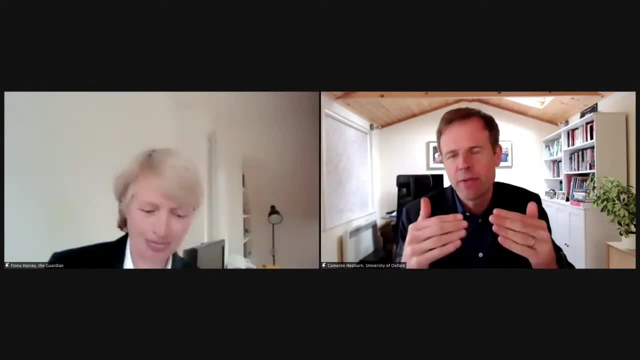 or whether it's teasing out the implications from that. There is a particular carbon budget and, as a result, capital stock that you can build out before you're above two degrees And, as a result, if you go above that, you're going to have stranded assets. 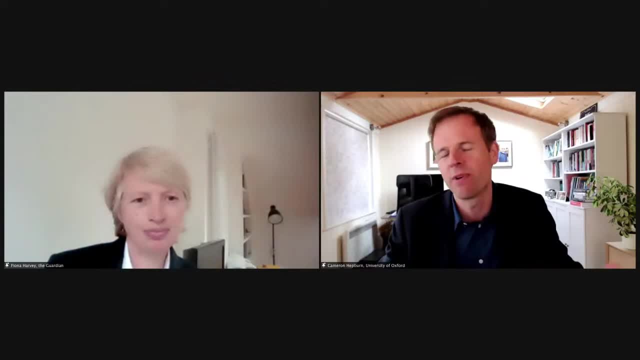 And, as a result of all those things, you need to have a net zero investment framework. It's Oxford University that has contributed each of these ideas in large measure to the world that the world is now picking up and following and putting into place. And then, of course, you'll hear shortly. I won't steal their thunder. 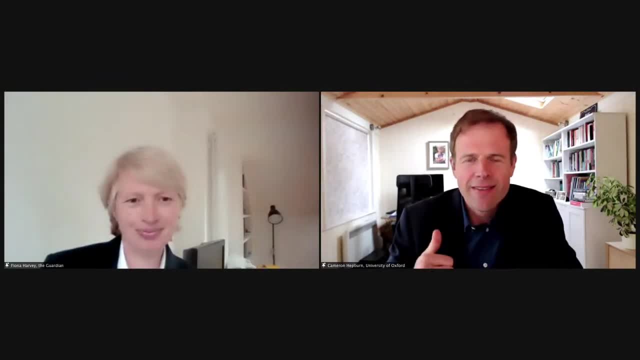 But we've got a lot of work to do. We've got brilliant scholars here who are contributing on nature-based solutions for net zero, on greenhouse gas removals, for net zero, on carbon capture and on the idea of where are these sensitive and strategic intervention points to take us there as swiftly as possible. 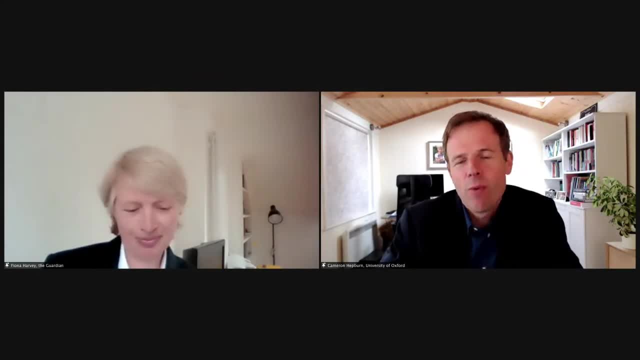 And finally, how do we recover from the current pandemic in a way that leads us and the world onto a pathway that can restore our biodiversity and to get us to net zero emissions? So that's pretty quick, but they're my three answers, Thanks. 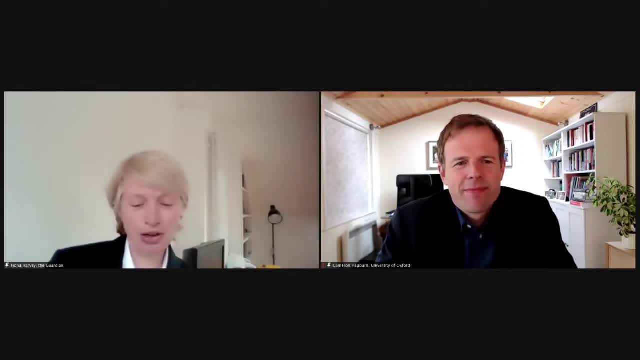 That's great. Thank you very much. You've provided a model of conciseness and clarity for the rest of our contributors. Thank you for that. So I'm going to turn next to the same question: How is the university contributing to local, national and global goals? to Natalie Seddon, who's Professor of Biodiversity also at the University of Oxford: 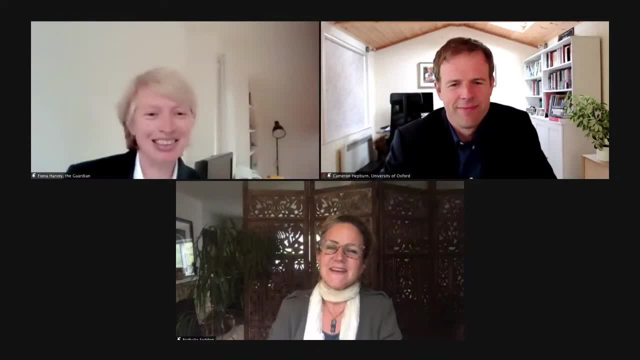 Professor Seddon, Thank you very much. It's wonderful to be here And thanks, Ydvinda, for a very stimulating answer. As you say, multi-scalar talk. I feel quite exhilarated after that, I have to say. 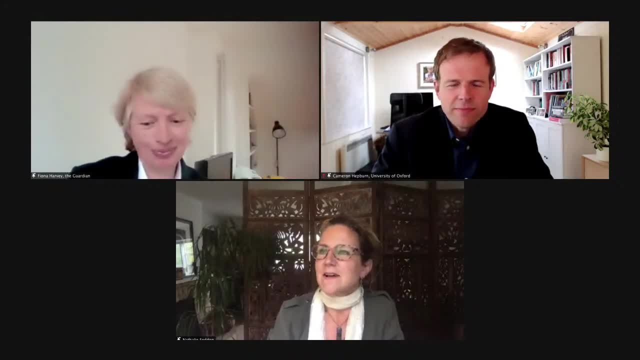 So I'm going to answer the question in a slightly different way by saying at least three ways, three things the university is doing that addresses local, national and international simultaneously. And the first is, of course, I think- and we've been hearing a lot about this today- aspiring to directly contribute to meeting net zero and net gain biodiversity goals, with a robust plan of getting there and inspiring other. 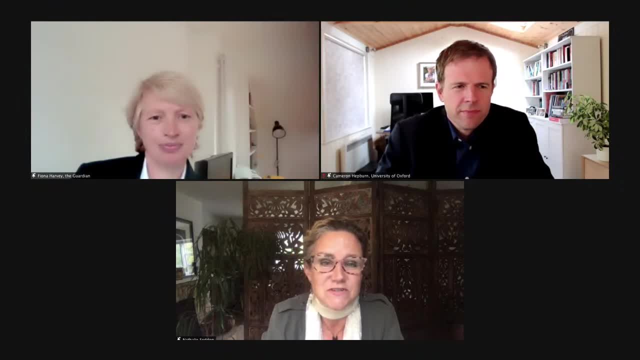 I think, organisations from the local to the international level to do the same And, as part of that, putting goals around climate change on the same plane as goals around biodiversity and, as we've been hearing, the interrelationship between those two is very intimate. 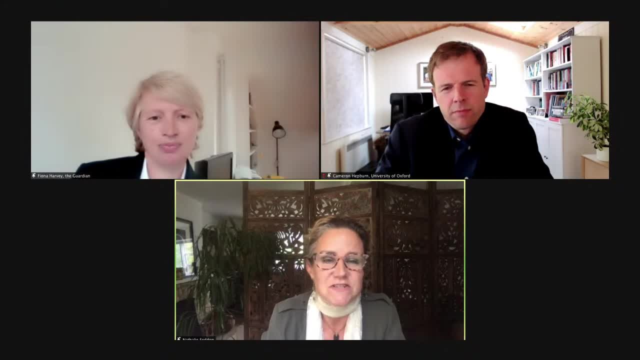 And we can't address one challenge without also addressing the other, And the university is recognising that And that is inspirational to all levels. Secondly, as Cameron said, I have to also, you know, back up what he said indirectly: we are through all the very high. 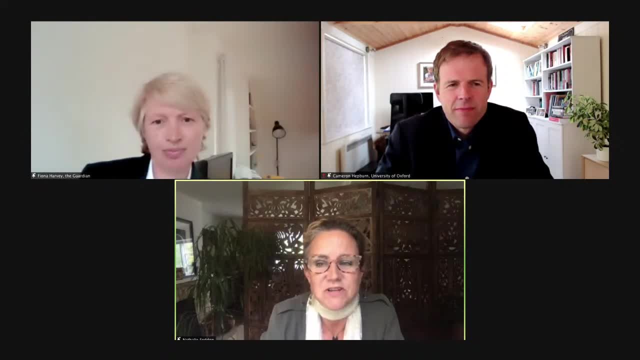 impact and increasingly genuinely interdisciplinary research we are doing, especially through all the new, current and upcoming initiatives around net zero, biodiversity in society, nature-based solutions, sustainable finance and so forth. we are now all really focusing on working together to find solutions in an integrated way to major global challenges and again providing a model. 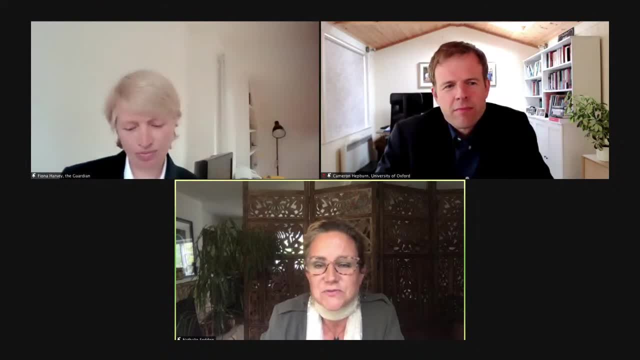 of how to do that, which we hope will inspire others at all levels. and then this year, I would say that many of us, many across the university, we are at the forefront of discussions and supporting decision makers and business and government, setting science-based, robust targets to include 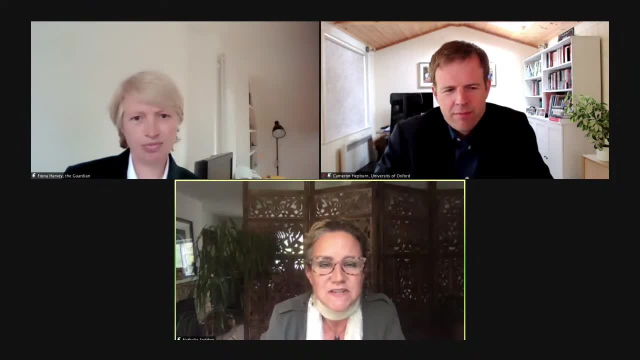 in the post-2020 biodiversity framework, to be incorporated into revised climate pledges, nationally determined contributions associated with the Paris Agreement, and we're all working hard to ensure that those science-based targets and plans for meeting them are aligned across all the different types of conventions at an 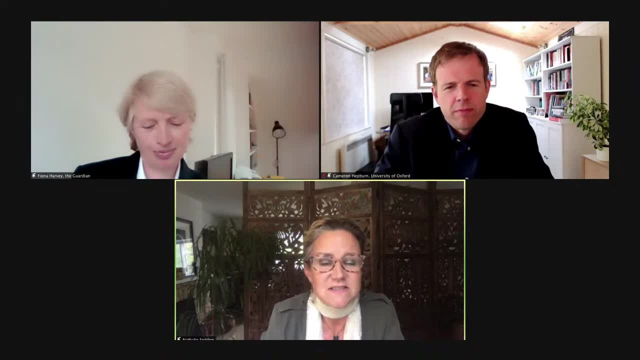 international level. you know what we're seeing- and Oxford science scientists have really played a massive role in- is bringing together communities of researchers, policy makers and practitioners who have previously not worked together before, in other words, the climate change community, the development community and the biodiversity community. thanks, 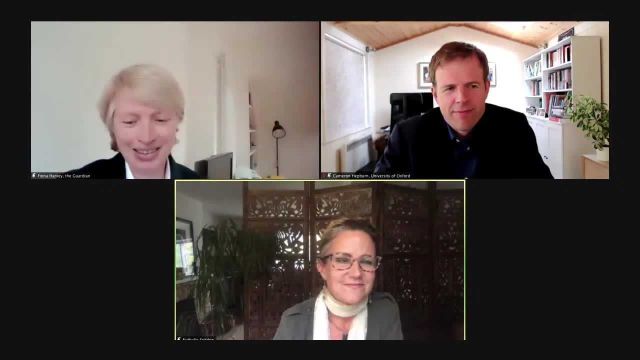 thank you very much for that. um, that's very useful and I'm sure we'll be hearing a bit more on some of those uh in a moment. um, I'm next going to introduce, uh, our third panelist, who is Guido Schmidt-Traub, who's a partner. 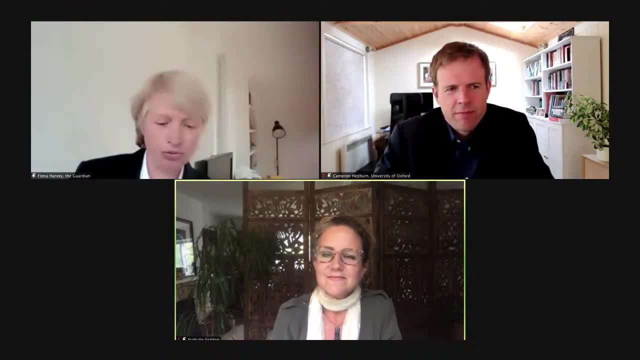 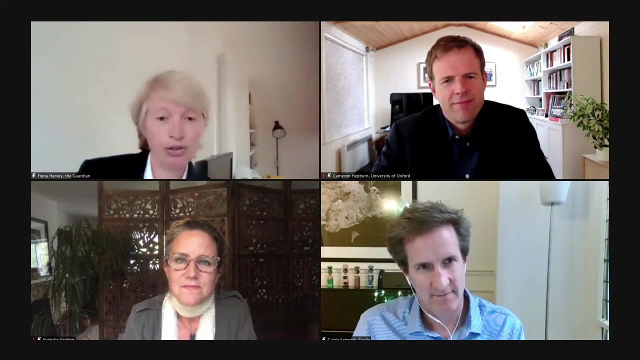 at Systemic Earth, which is a consultancy that does a lot of work in these areas. um Guido was at the Sustainable Development Solutions Network before Systemic and is also an alumnus of Oxford, and so perhaps you could tell us how the university is contributing to the sustainable development ecosystem. 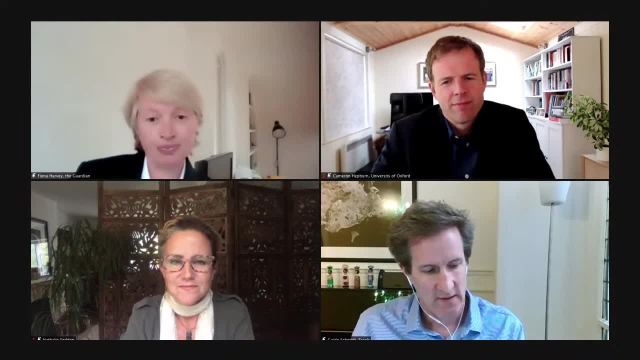 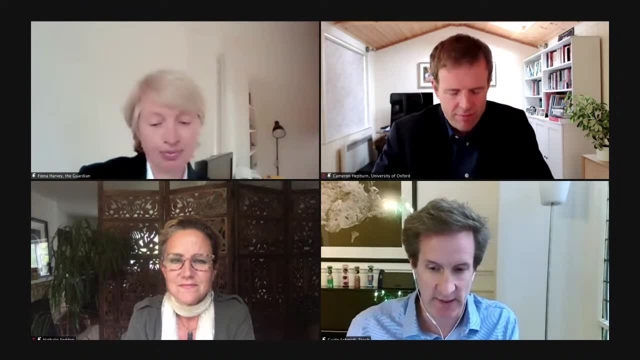 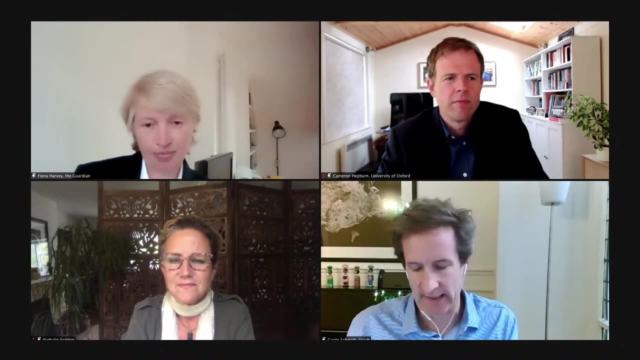 local, national and global goals. I want to echo everything that's been said. This is a very bold and extremely important commitment. It's a joined-up strategy that is honest about the scale of the challenge, the magnitude of the challenge. I also like the fact. 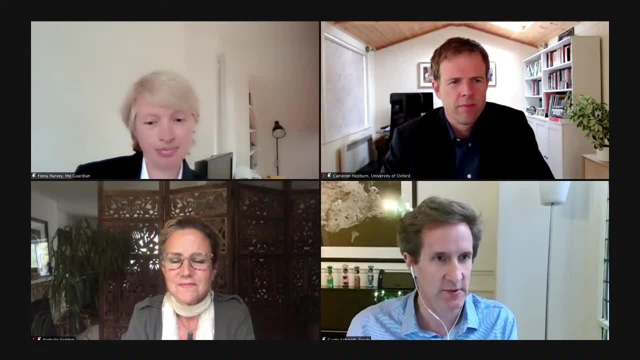 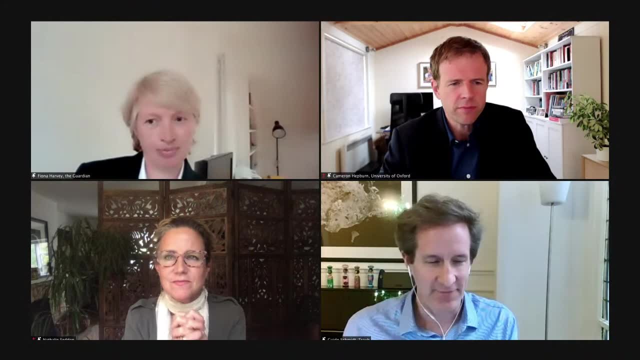 that it's not just counting greenhouse gas emissions but also looking at biodiversity and other topics that also often fall off the agenda. I haven't been privileged to be part of the design of the strategy, so I only know what's being described here. 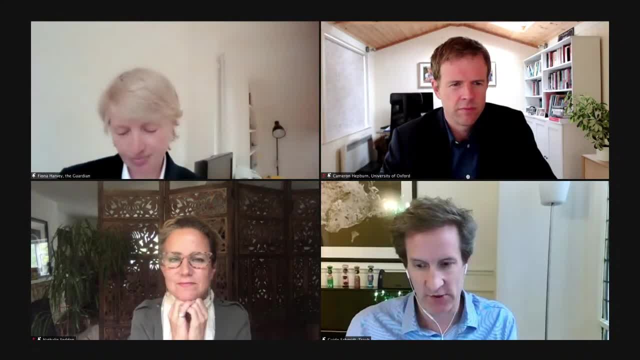 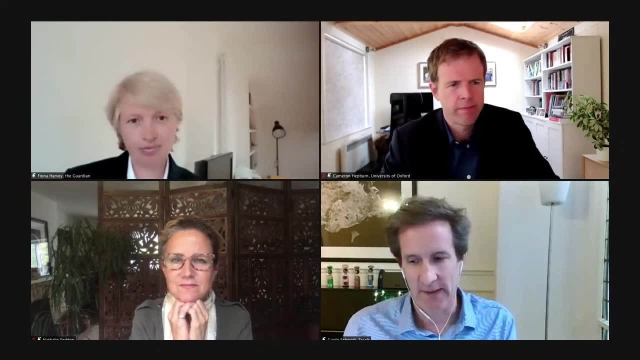 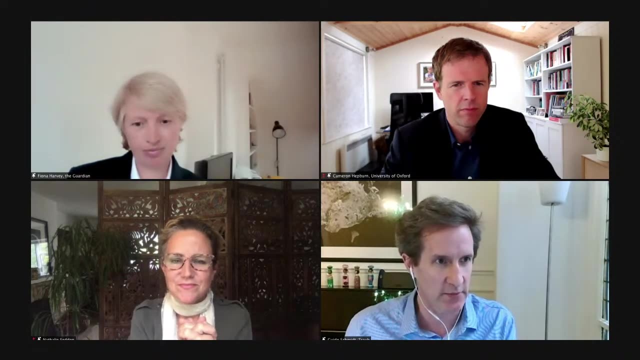 Let me maybe just outline some ways in which the university could perhaps even help further the world advance these goals. One is, of course, to teach these things. Oxford is privileged to have a structure that makes it easier to teach across subject lines, and I think that's really, really important. 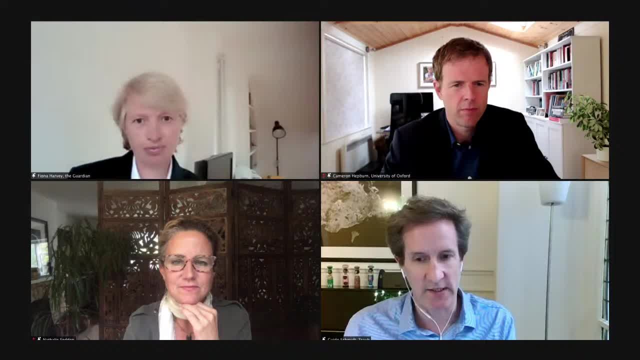 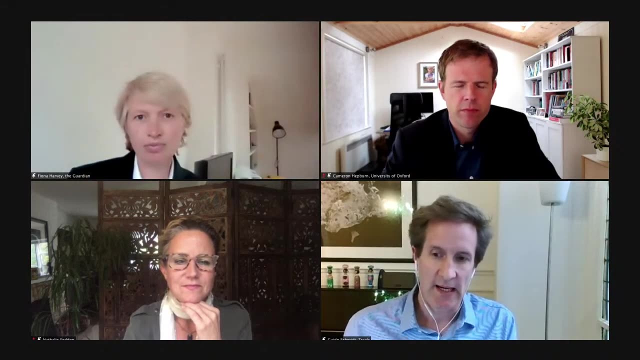 to take lessons and findings from those and to integrate it into the teaching, as has been mentioned by many, because today's universities don't yet prepare people for the practical problems of, or the practical problem-solving that's needed. Second, I and several of the speakers have 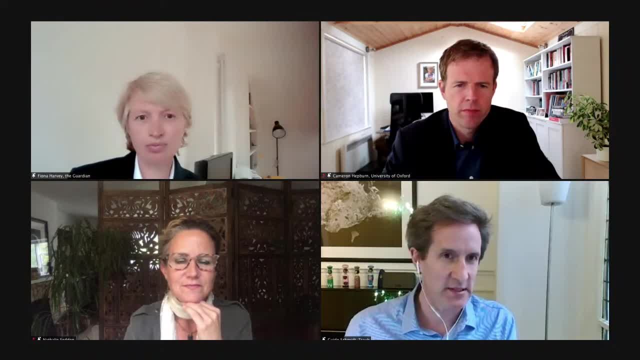 emphasised the importance of carbon budgets and targets. Essentially, this is a massive backcasting exercise. How do we get to net-zero emissions by 2035?? It's framing the problem almost the way in which an engineer would frame the problem. That's not how science typically works. 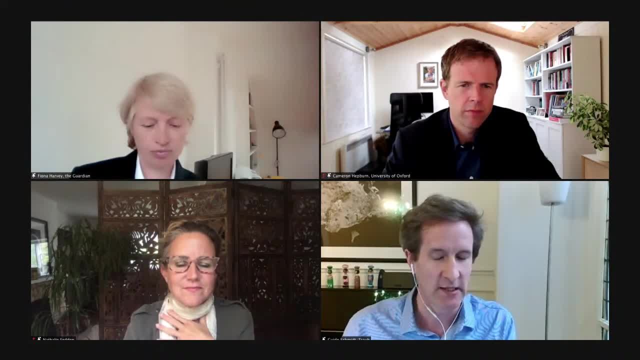 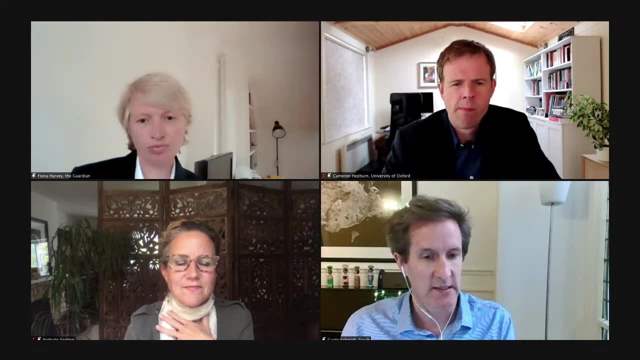 Science works for the undirected expansion of knowledge, But here we actually need to apply problem-solving skills to solve a very complex issue. that requires engineering, economics, all the social sciences and, of course, mobilisation inside the university. Again, this is a challenge. 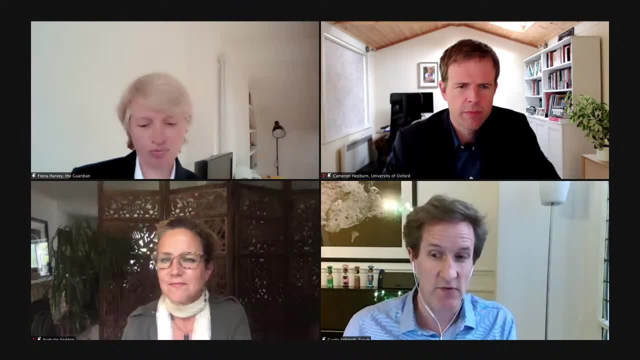 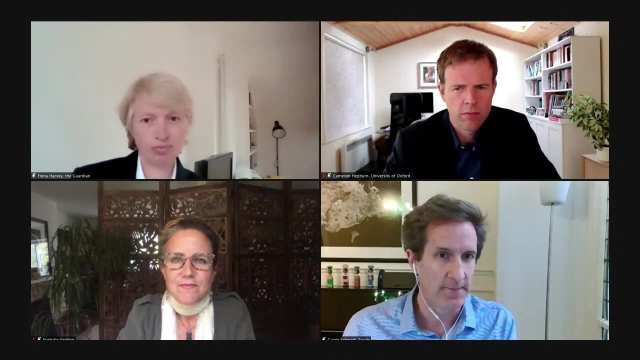 that science and universities and research institutions around the world are rising to but are not yet really well enough set up to do So. really thinking through how can a university coalesce around the question of how to meet long-term goals is a really important, almost methodological point. 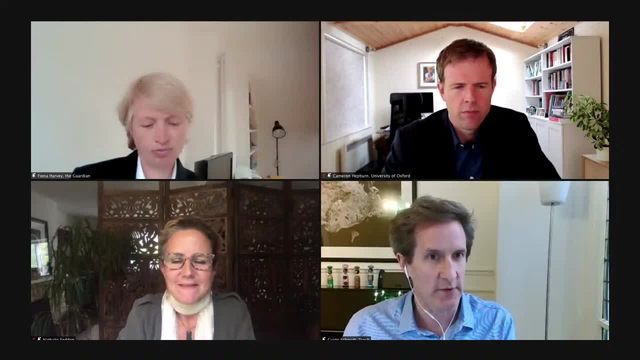 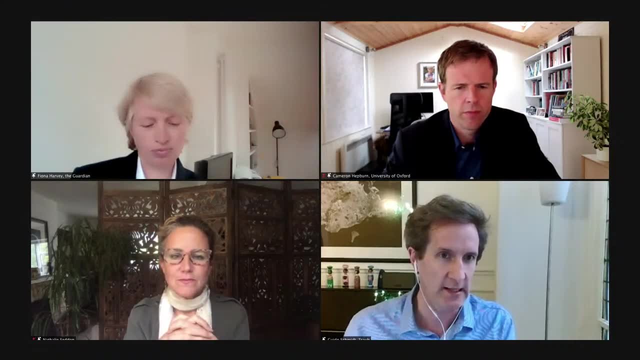 And it's one that we need to understand better how it works. It's one that we need to help other universities and other research institutions to apply as well. I'm seeing this also in discussions with some of the leading editors of major scientific journals, who are saying: 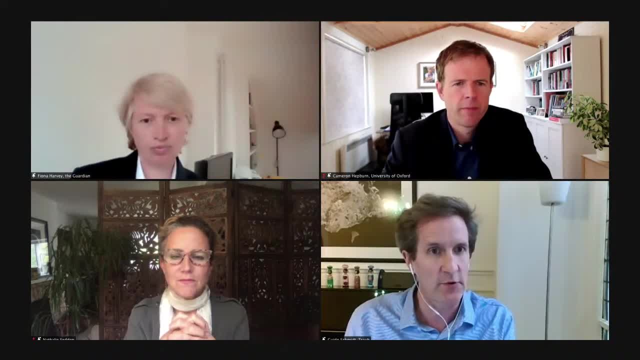 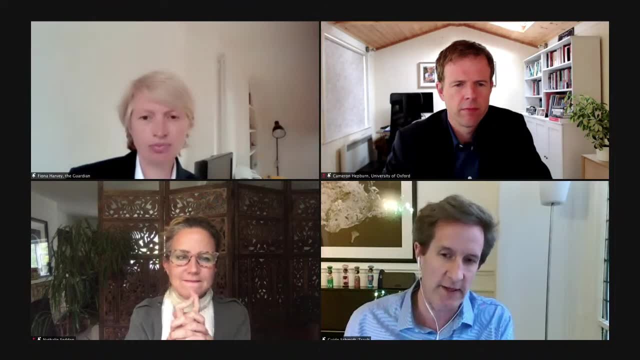 we're just getting individual papers that look at snippets of the problem. we don't get the integrated approaches, And so I think this is what Oxford has an opportunity to show. My final point is, as has been mentioned also, Oxford is privileged to have unrivaled 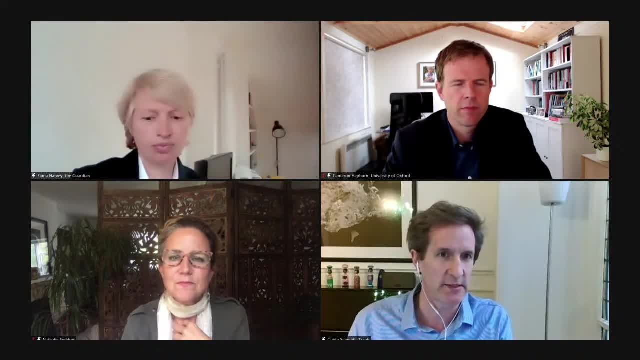 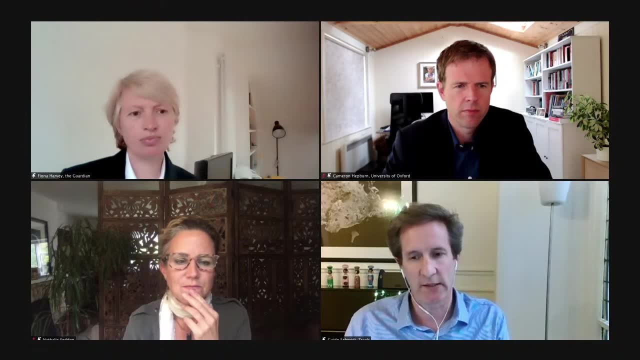 resources, both intellectually- in terms of its students mobilisation, and also financial. Many other places are not as fortunate, so I think it would be really good to think through how other organisations can benefit in real time from the learnings and also from the mistakes. 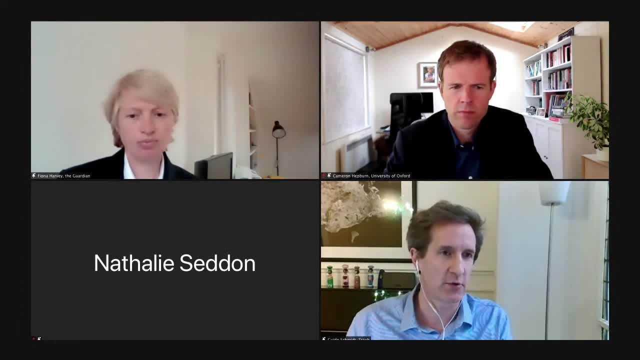 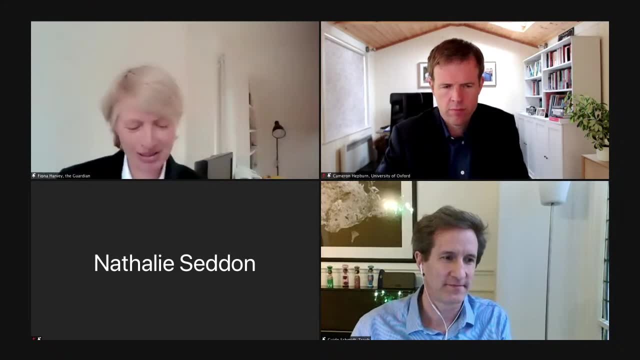 that invariably will be made so that more universities and more organisations can follow this path. Thank you, Thank you very much. Thank you for that insight there. That's very helpful, And I'm going to move on now to Kate Norgrove, who is: 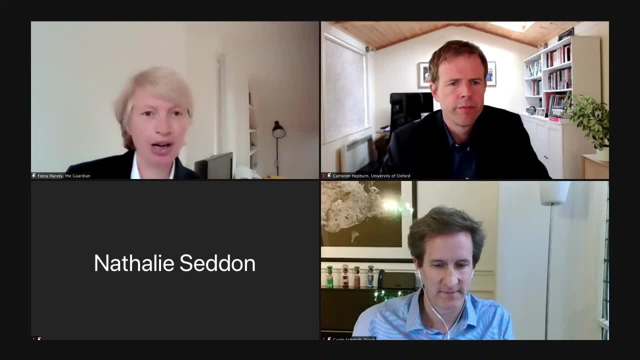 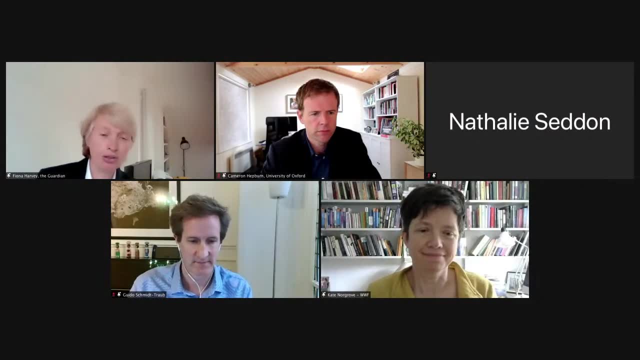 Executive Director of the World Wildlife Fund UK. Kate, you've got a different perspective there. Can you tell us why you think the university can contribute to these goals? Thank you, And unfortunately I'm not Executive Director of the whole organisation, just of advocacy. 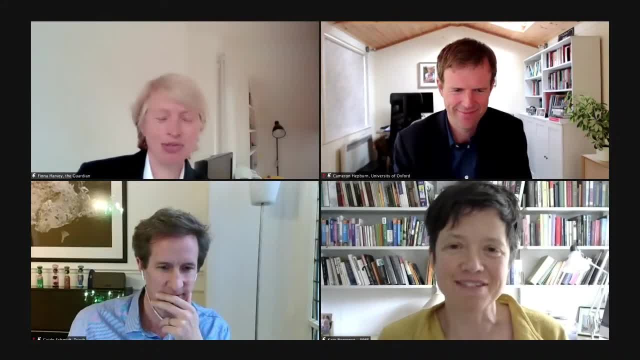 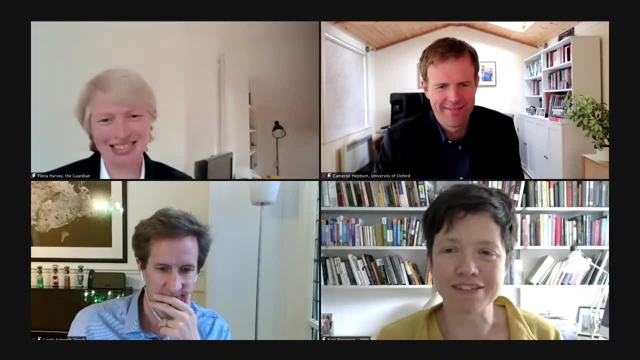 and campaigns? I won't. You've just had a promotion, there you go. Yeah, I'll give it a go. So this is the time for plans and responses that match the scale and the severity of the challenge, And so, in that context, I want to say: 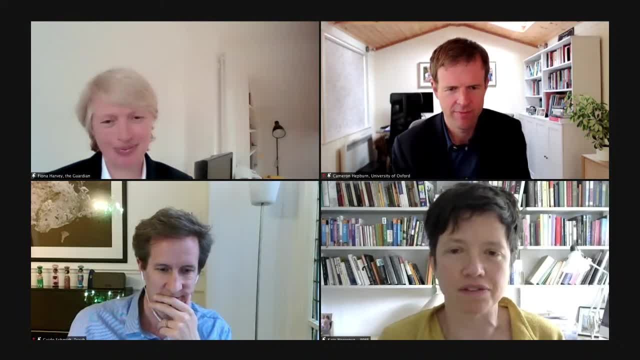 two things about Oxford's strategy, which is, as others have said, very ambitious: One on nature and one on climate. So on nature first of all, as Natalie said, we have a lot of. it's quite rare for institutions like this one. 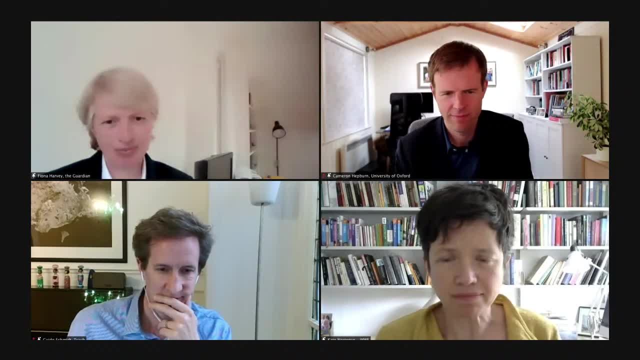 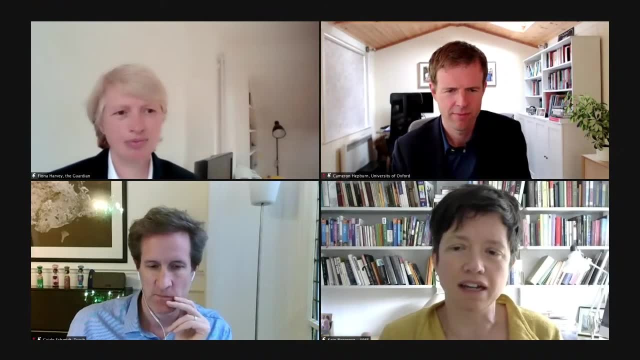 to put climate and nature on a level pegging, aiming to achieve biodiversity net gain by 2035 and net zero. And this is good because, as others have said, climate and nature are two sides of the same coin And one crisis can't be solved without solving the other. 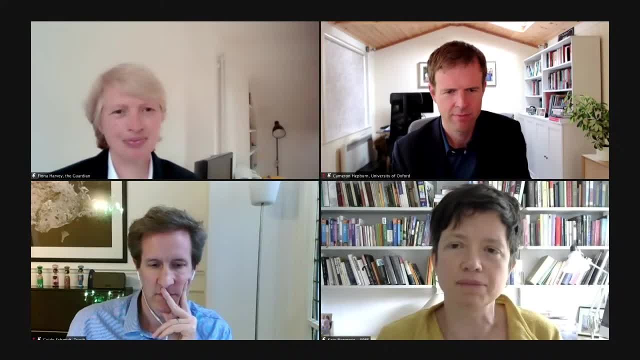 But my question on the biodiversity net gain issue is in how it's going to be implemented in Oxford and then globally as well, and nationally, because it can't be achieved just by, say, restoring land in Oxford, As Yadvinder and others have said. 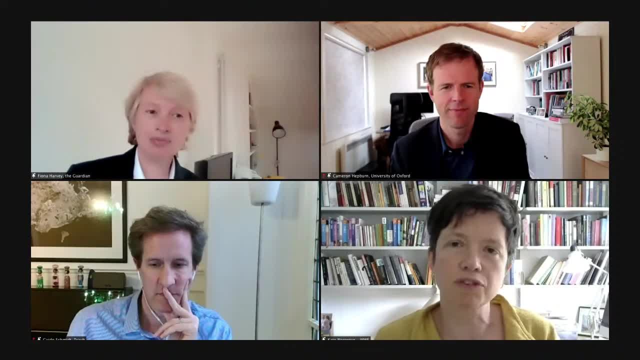 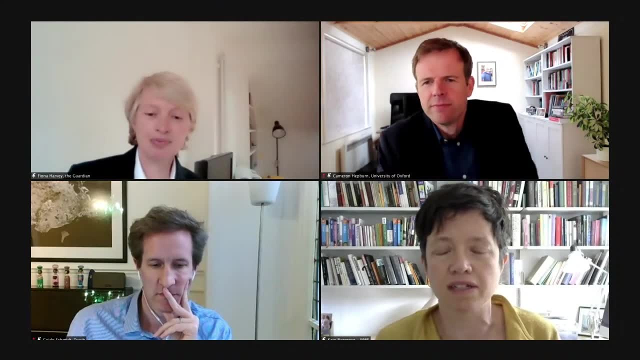 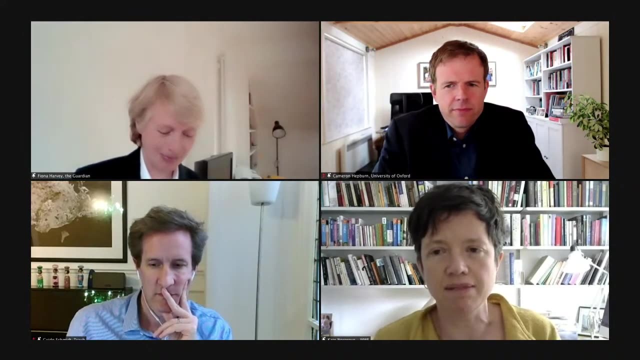 the destruction of nature that Oxford is responsible for comes from activities in Oxford's supply chain, So from construction projects to paper and activities in laboratories, also in food, as others have said, And that needs to be tackled, and urgently. So it's fantastic that scope three emissions. 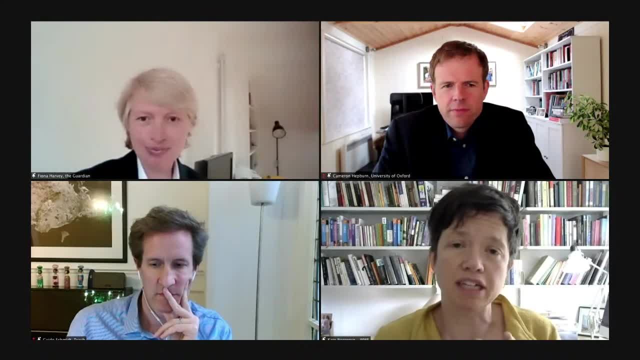 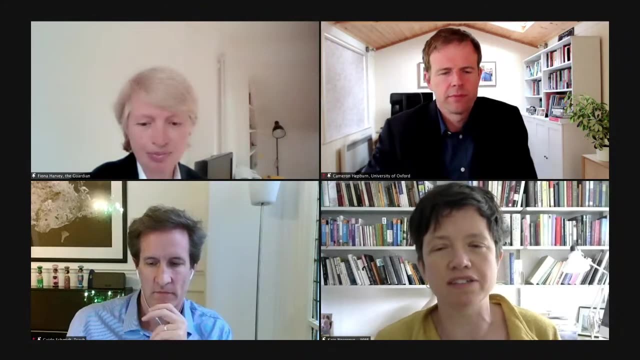 and destruction of nature are in this strategy, because tackling these supply chains effectively will have influence globally and nationally, And that's really important. The second thing I wanted to say is on climate. So this is a really ambitious and welcome plan, And it's fantastic that the university will prioritise. 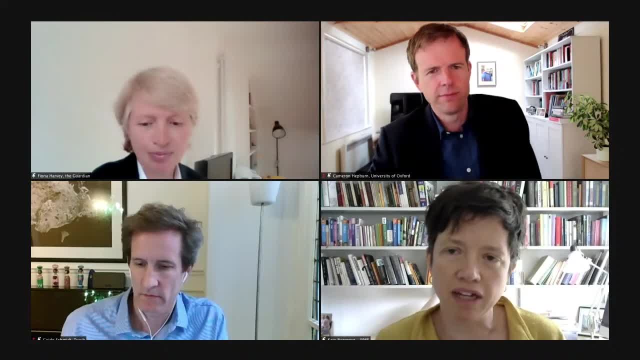 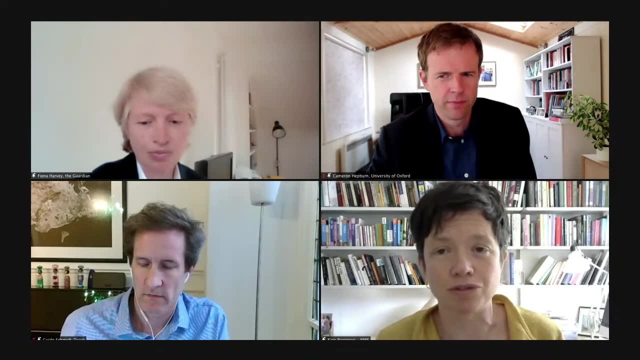 reducing greenhouse gas emissions, including a target on flights, before considering offsets. So this might sound a bit of a strange thing for conservation- someone from WWF, a conservation organisation, to say- But I think there's a risk that nature-based solutions 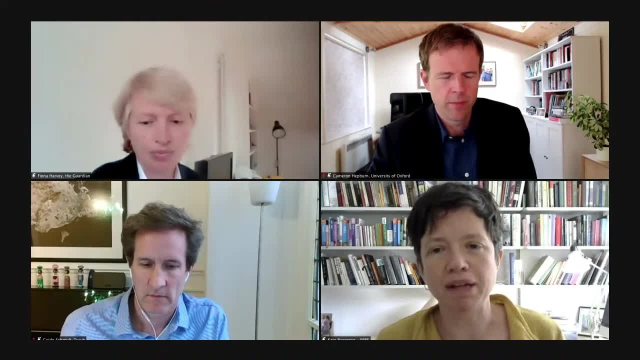 become a magic bullet. They're not. They cannot replace the substantial emissions reductions that we're seeing. We need to see first. It's almost as if planting trees is an apolitical thing. It's not apolitical, It's very political. 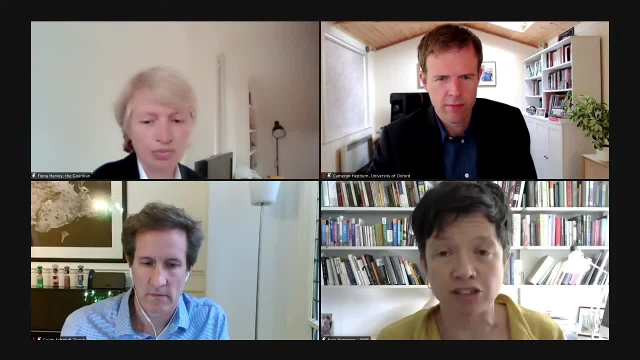 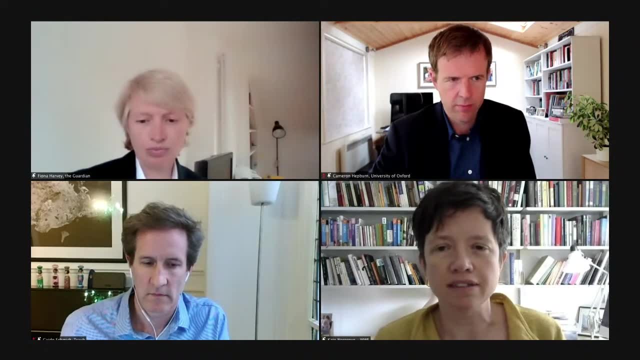 And implementing nature-based solutions are not a magic bullet and are not going to be easy either. We need to tackle emissions. So my question, though, for the strategy is on the continued scope in the strategy to continue carrying out research for, and in collaboration with, fossil fuel companies. 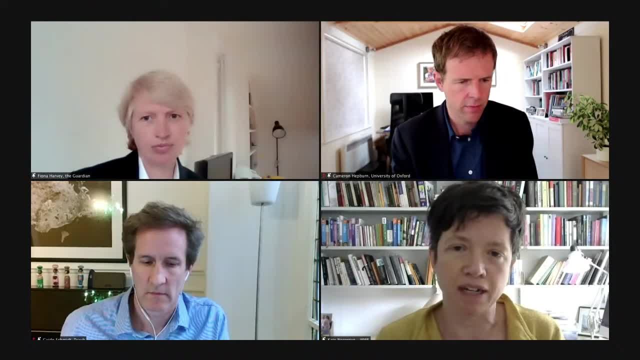 So, although it may be a minuscule proportion of research and investment, as we heard earlier, it's also important, symbolic and influential, And, in the same way that the plastic bottles on the table in meetings are, so is investment and continued collaboration. 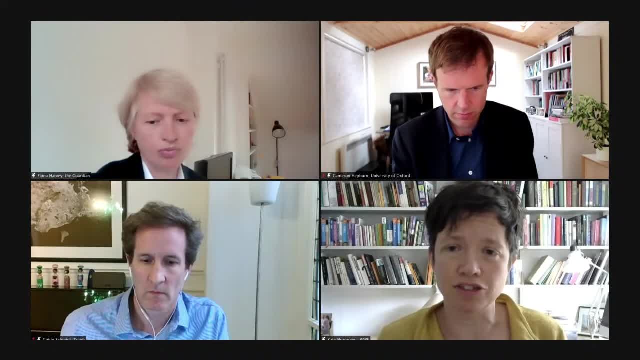 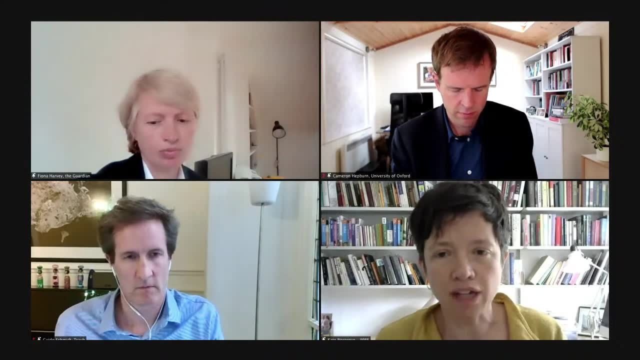 with fossil fuel companies. So continuing to accept these donations, of any size, facilitates the sort of greenwashing that we just don't have time for right now. All companies are going to need to transition to a 1.5 degree plan, and that will take time. 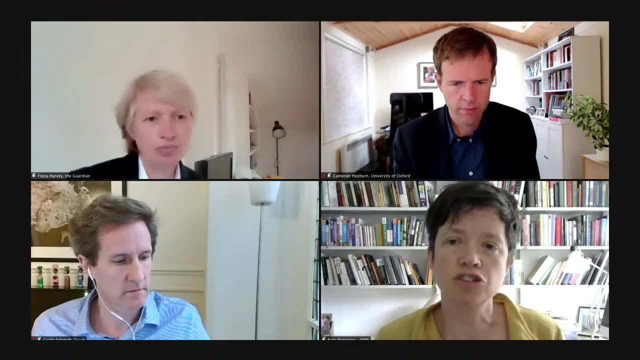 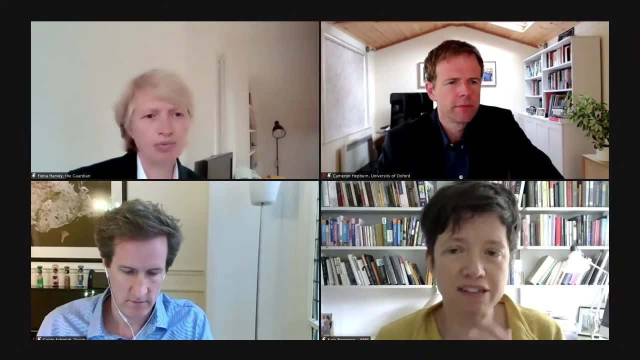 But a university whose primary mission is to facilitate learning should not be facilitated by the government. Instead, they should be leading the way on the new. So, really, in summary, we're facing a three degree world: the collapse of natural systems that sustain us. 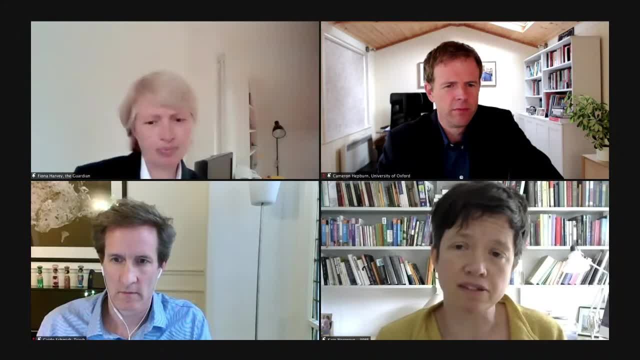 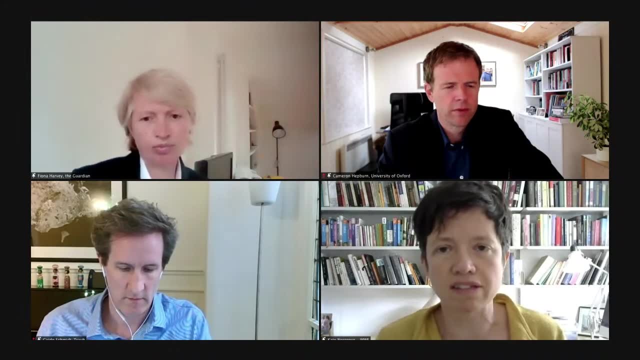 This is a really important start, but the scale and significance of this needs to guide all of our decision making in all of our institutions and organizations, And there's also a role for all of us here today to take that and make it much more ambitious, to influence both nationally and globally. 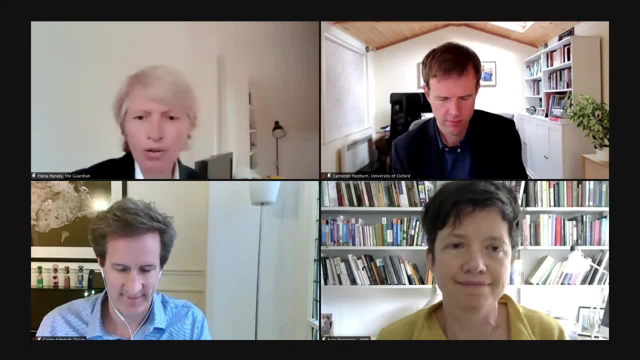 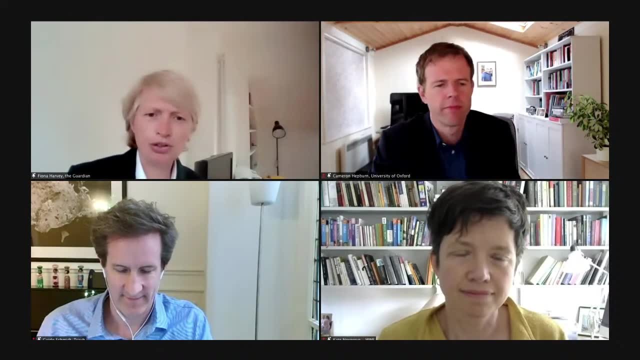 Thanks, Fiona, Thank you very much indeed for that. And would you, Kate, as I've got you, would you ban the university from researching into activities that would increase greenhouse gas emissions? Would you, for instance, ban the university from researching? 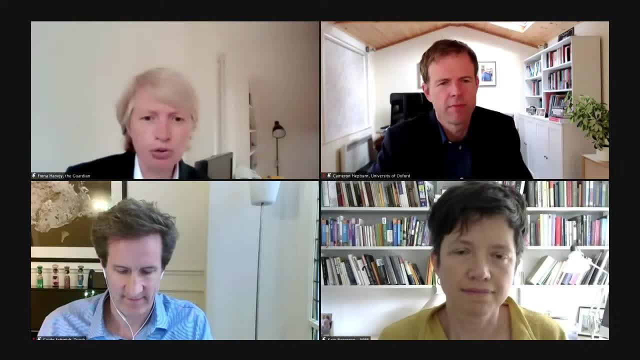 into extractive industries, and extracting fossil fuels particularly. Yes, I would do, Or I would at least make a commitment to do that within a short time frame. I'm aware that these things take time to extricate themselves from and they take money. 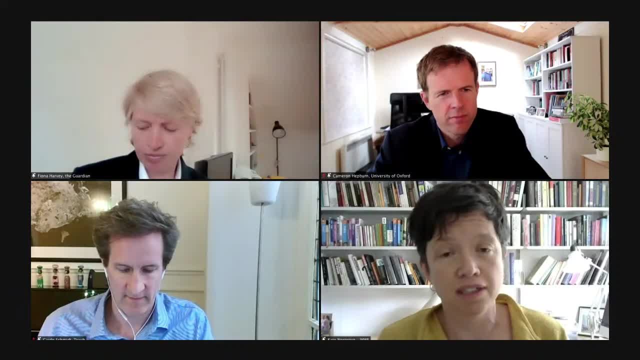 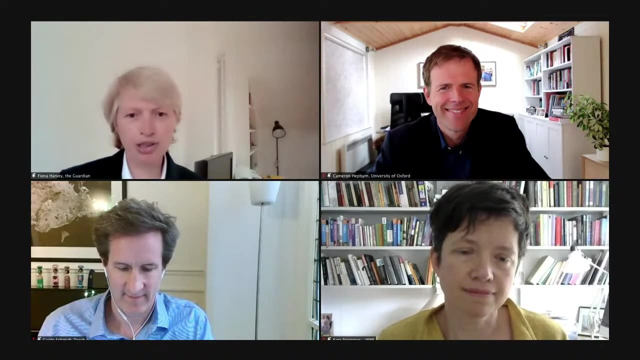 And you know, just working out where your emissions are takes time and money to do, But I think it's something that the university has money. It's symbolically very important And I think the university should do it Great. Well, we can ask our other panelists if they would do the same as well. 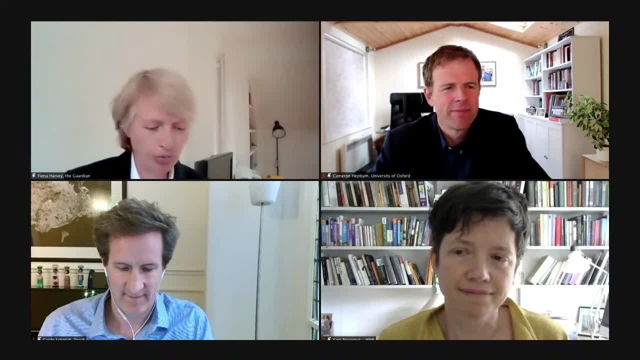 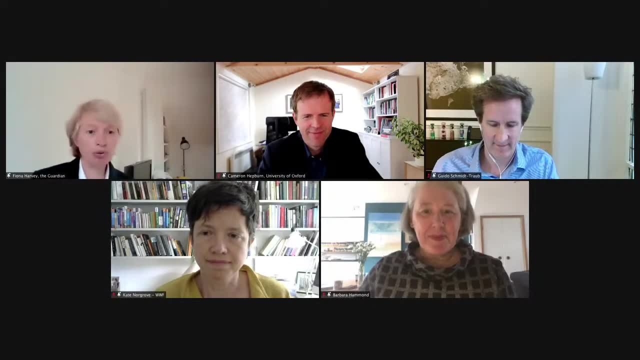 Thank you very much, Kate, for that. That's great, And I'm going to move on to Barbara Hammond, chief executive of the Low Carbon Hub in Oxford, to this same question, Barbara: How is the university contributing to local, national and global goals? 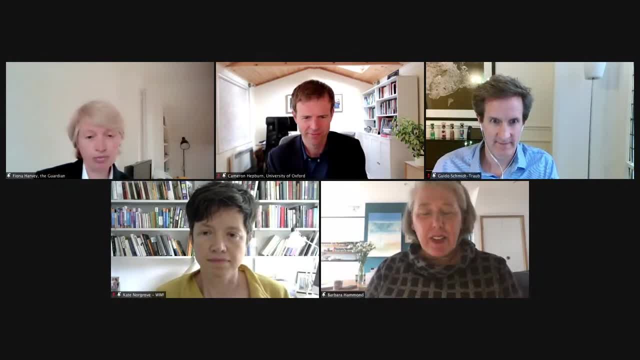 Thank you. Thanks, Fiona. Yes, I think the phrase was the one that Yadvinder used towards the end of his presentation. It's about communities of practice And I think over the ten years that I've been starting up and growing the Low Carbon Hub in Oxfordshire I've seen the university move. 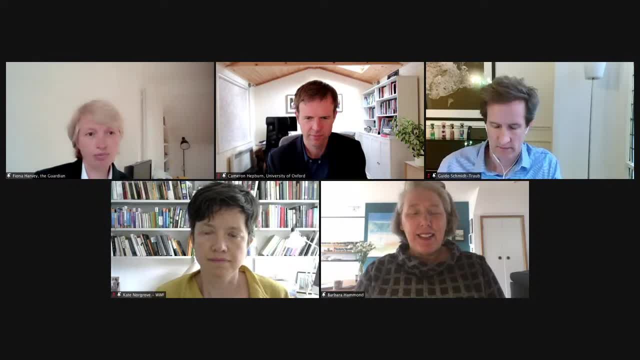 from an organisation that was thinking globally and, if it acted, acting globally, to one that really understands the obligation and the job that it has at the national and the local level. We haven't really talked about people yet at all this afternoon. We've seen lots of graphs and we've talked about systems and biodiversity and whatever. 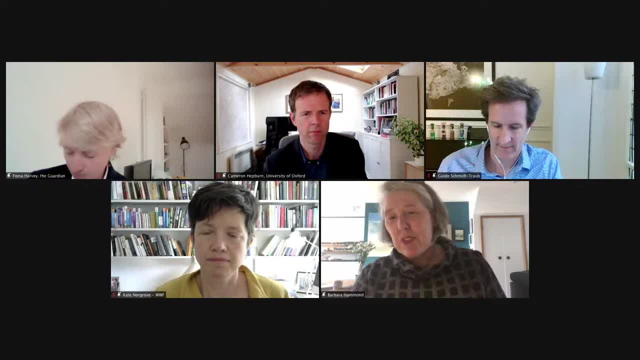 We've got to bring people along with us, And it's just very exciting to me to see how embedded the university now understands it to be in its local landscape and in its local communities, And so the thing that it is doing, and needs to carry on doing, is working in partnership. 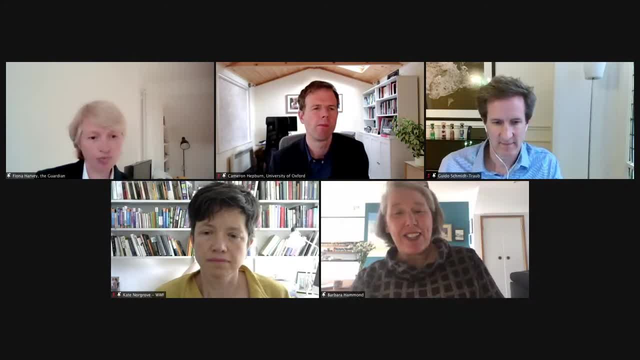 to involve local people in cutting edge innovation projects that are going to be demonstrators at the national level and hopefully repeatable at that level and at the global level. One of the examples that I know of and am involved in are two smart energy demonstrators: Project Leo, which is local energy Oxfordshire that's working out how to get the energy system. 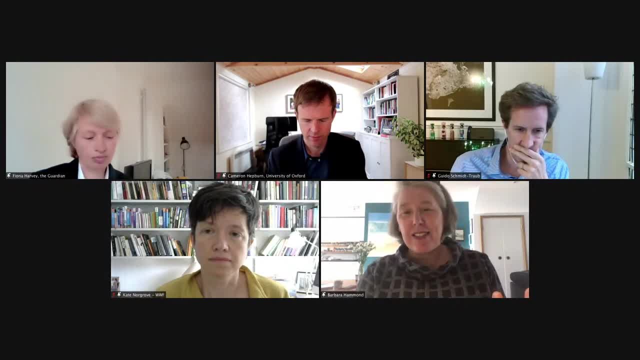 working at the grid edge rather than massive power stations at the centre, And the Energy Super Hub Oxford, which is about massive storage based in a city to start balancing the energy system. at that point, It's incredibly exciting That we have two out of three national demonstrators in Oxfordshire. 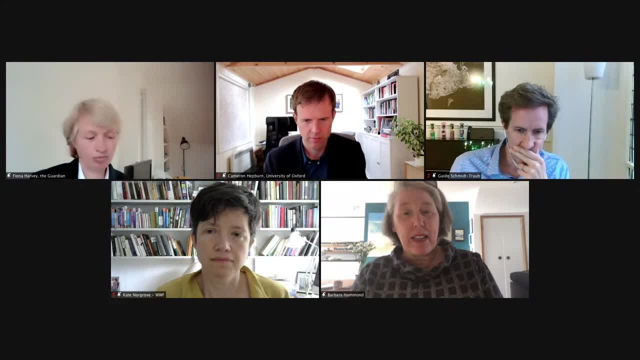 And that is because we have the community of practice here. Here we have the networks, And I want to get to the point where I'm as proud of Oxford because of the work that it's done on energy system acceleration And it's about to start a new centre on that, as I am about the vaccine and public health knowledge. 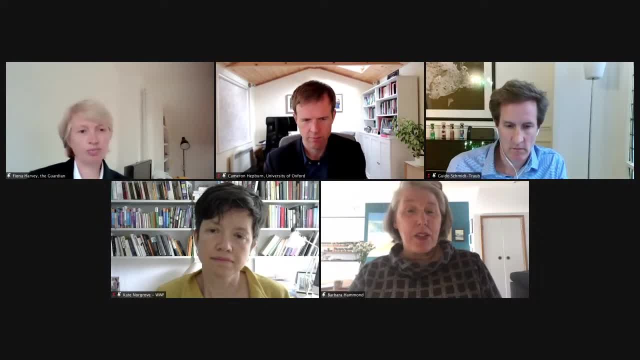 that it's contributed to- And it's about to start a new centre on that, as I am about the vaccine and public health knowledge that it's contributed to. Great, That's a great aspiration there. Thank you very much indeed, Barbara. 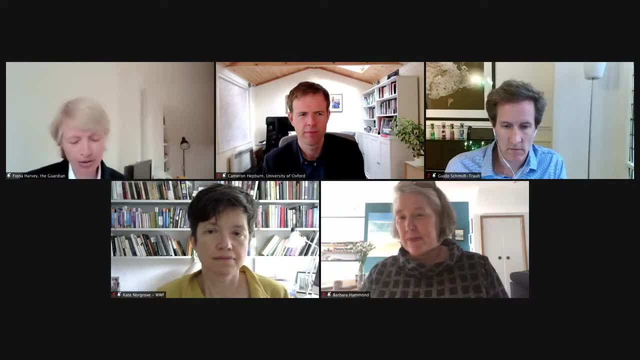 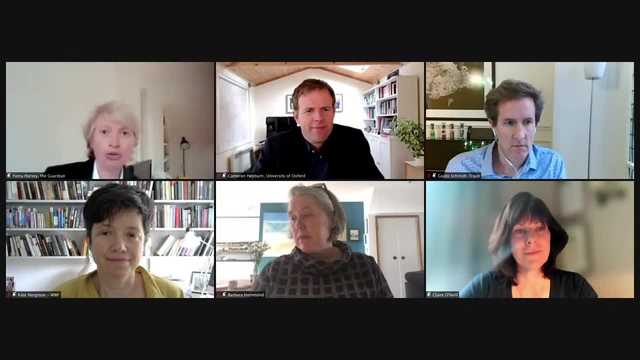 And I'm going to move on now to Claire Perrion-Neal, who's the Managing Director of the World Business Council for Sustainable Development. And, Claire, of course, you were the original president of COP26 for the UK and a former energy minister, I think. 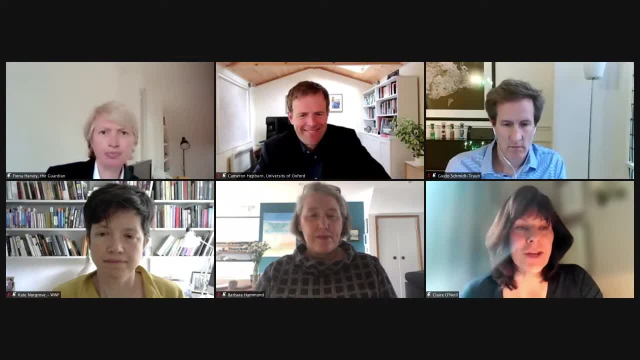 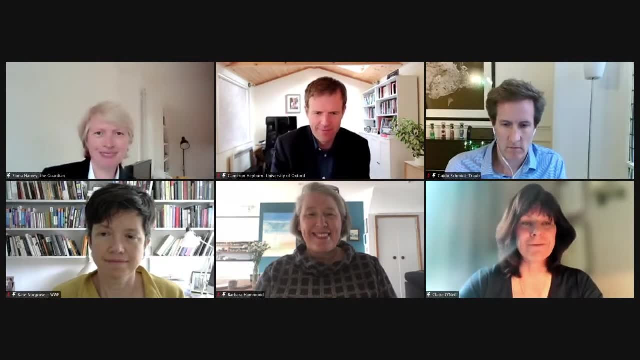 So perhaps you could give us that perspective as well. Thank you, Fiona, Fantastic to see you again, And the challenge going at this point in the panel is: lots of great answers have already been given that I would have tried to give, But I guess what I wanted to focus on is whether we're looking at a local, national or global level. 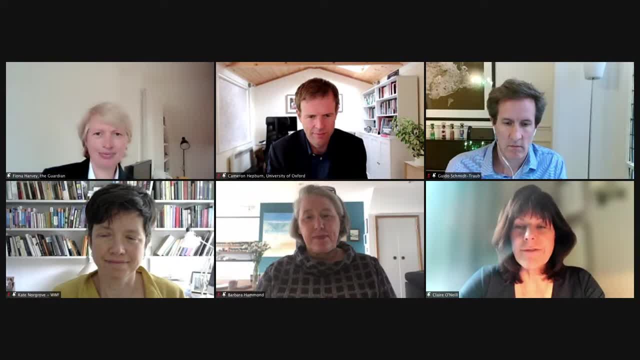 I think there are three persistent problems that we face, particularly as policymakers, And one of them is that there is just an ongoing disconnect between the debate and the science, and actually a persistent disregard, if you like, of the science. The second is there is an enormous gulf between pragmatism and ideology. 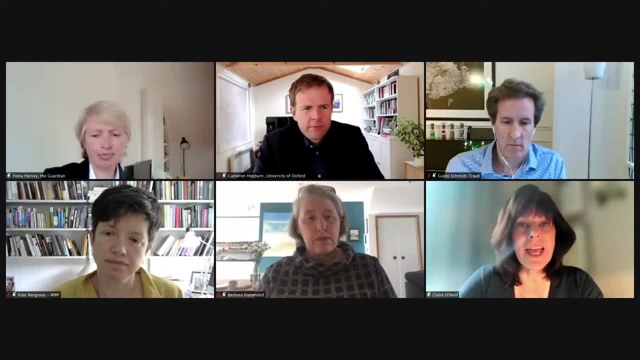 And it is particularly acute it might be when we talk about things like the energy transition in the developing world or how we actually mobilise nature-positive solutions to, as Kate has said, not be the answer but be certainly part of the toolbook. 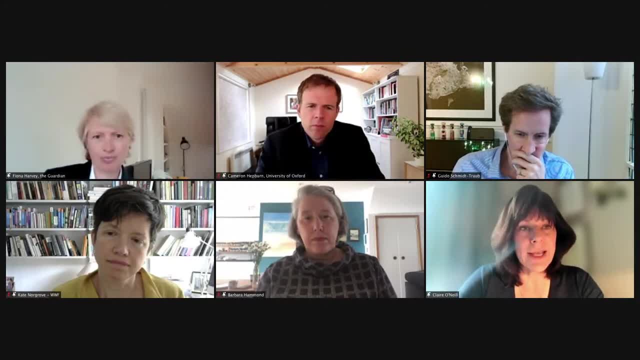 And we do ourselves a massive disservice actually by spending time fighting rather than coming up with practical solutions. and the last point is- and this is what's been so exciting about today's presentation- is the constant need to make linkages between the biosphere, between the atmosphere, between the 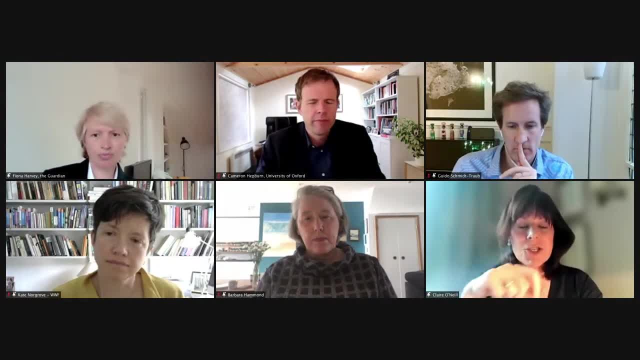 geosphere, between humanity. you know, those connections have historically not been made, because the best sustainability policy is trying to be climate positive, nature positive, positive and reduce global inequality. and i think, for me, what's so exciting about the launch today and the oxford um sort of offer is, first of all, you know this, the oxford team is underpinned with 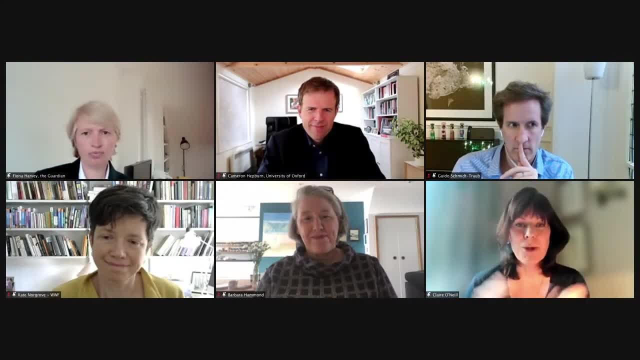 excellent science. i'm a school of geography graduate. for many years ago we were talking about this stuff- uh, many decades ago. that the, the scientific underpinning now what oxford has done and actually produced is, is incredibly strong. secondly, i think there is this great role of 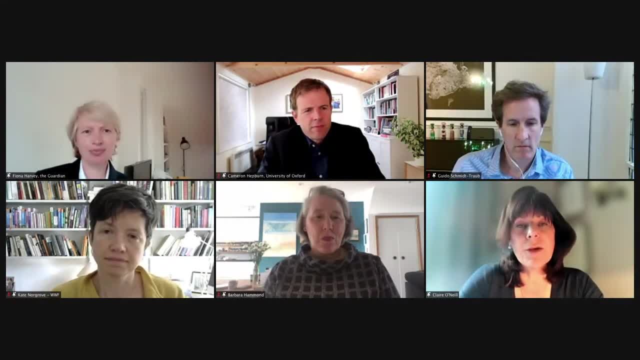 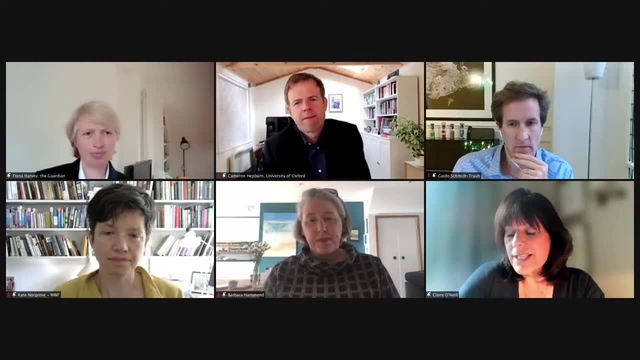 enlightenment. i mean it was fascinating hearing i've been to talk about the idea of the global metabolism, but also this integration of these different layers that need to be brought together and i think that sense of enlightenment also when it comes to practical proof points. so the oxford principles have driven. 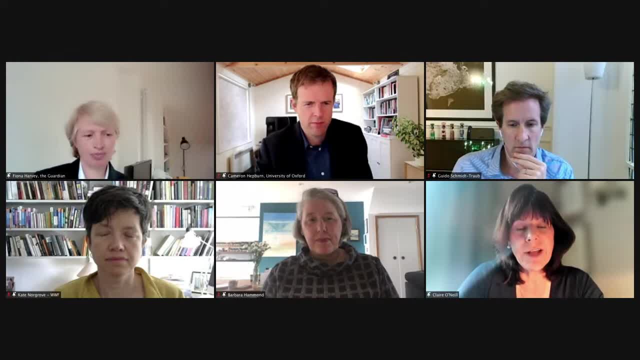 much of the progress we've made in voluntary carbon market development over the last year really fantastic proof points and, as barbara was saying, we're also able to see local examples on the ground that are replicable at scale and in volume right across the uk. and then i think the final thing is the ability to to kind of authoritatively advocate. i mean it. 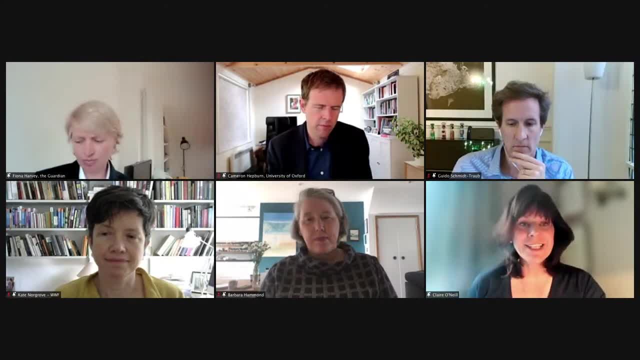 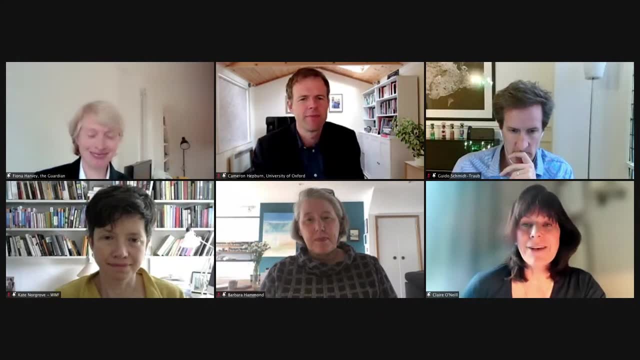 is rather shameful how little policymakers listen to scientists. um, i'm sure that doesn't come as a surprise to many, but you know we don't often sit around the various uh tables in government and have conversations that are science. informed science almost has to fight to get its voice. 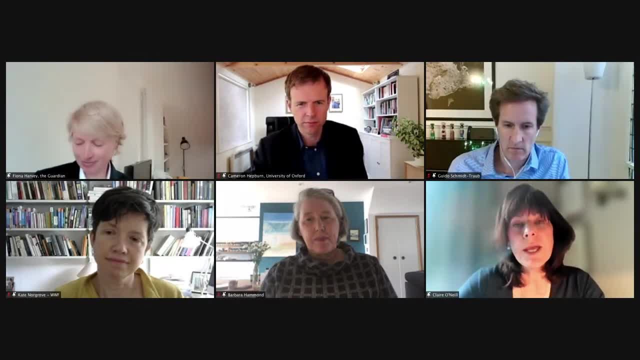 its voice heard and the ability to actually join up- uh, really strong policy messages, to link up as institutions- which i know the oxford team plan to do, so there is a really authoritative set of information and messages- and also to develop the skills, one of the other things we haven't spoken. 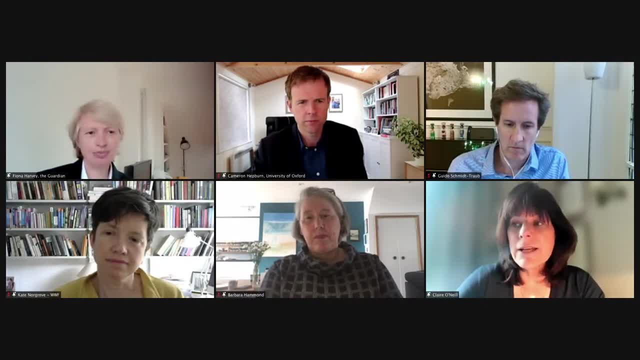 enough about, i think, is the role that oxford is doing in creating this huge network of sustainability professionals, both in academia but also going into the business world, and i'll finish on that point. i've drawn a thankful veil over my long career- 10 year career- in politics there. 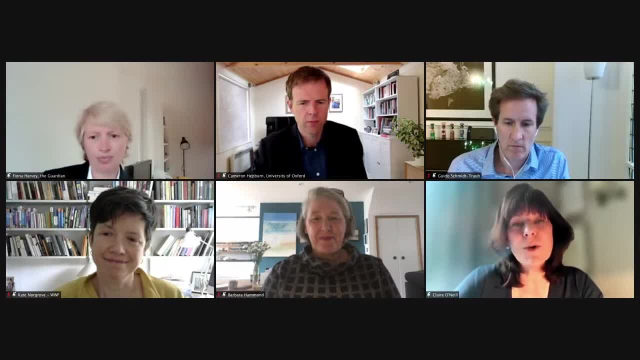 were some great points, but also it was tough. the opportunity now to work with the world's most ambitious businesses globally who in many cases are driving that sustainability, ambition and action far ahead of governments, is incredible, and it's great to see oxford kind of educating. that's that next. 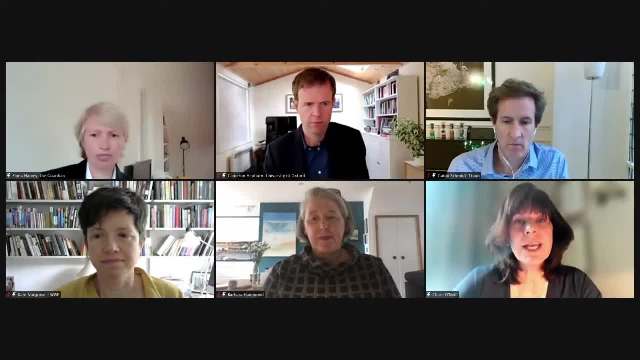 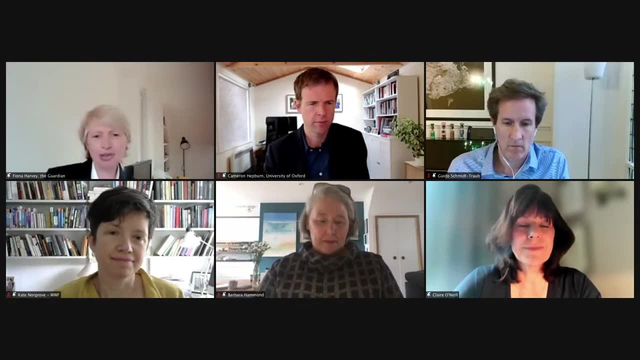 generation of sustainability professionals to take that message out into the corporate world as well. great, thank you very much indeed. um, it's very uh useful to have that insight, and one of the things that i think is really important is that we're not just talking about: well, i've got you there. uh, claire, i've actually got a question that's very specifically for you. 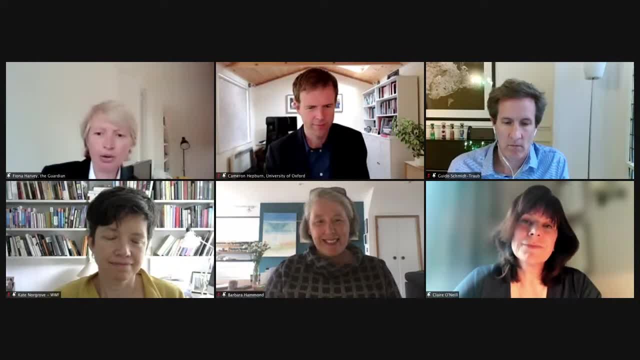 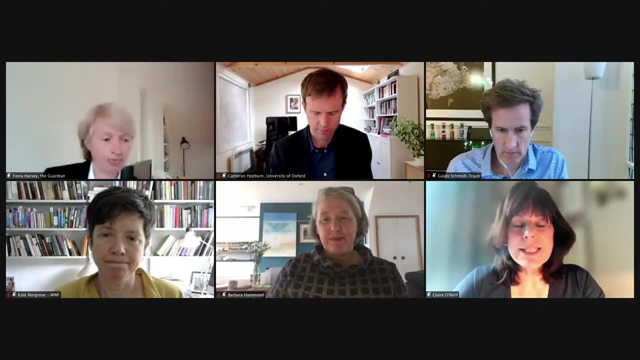 that i think it's appropriate to ask now. um, the question is from peter spark and it's: how is oxford university working with the world business council for sustainable development towards cop 26, if at all? you give us very briefly what you're doing there. well, i, i would love to. it's, it's, uh, love to. 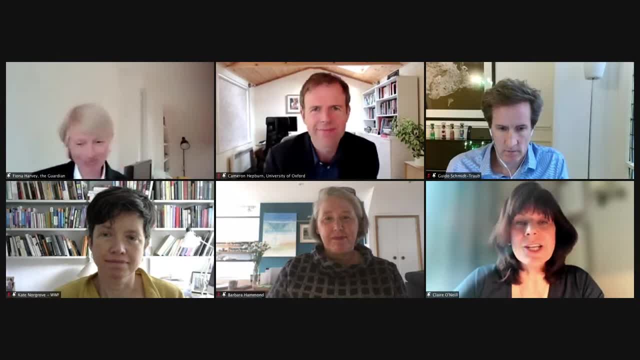 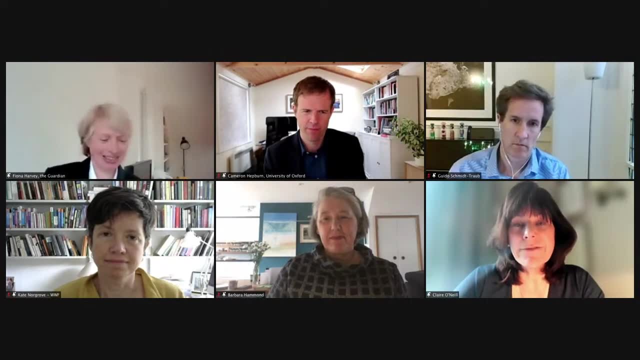 tell you that professor miles allen, who i'm thinking is speaking next- uh, is it- has actually joined the wbcsd climate and energy programs advisory board because we are working very specifically now on a whole suite of removals initiatives, both ncs, positive nature, positive ncs removals, but also increasingly 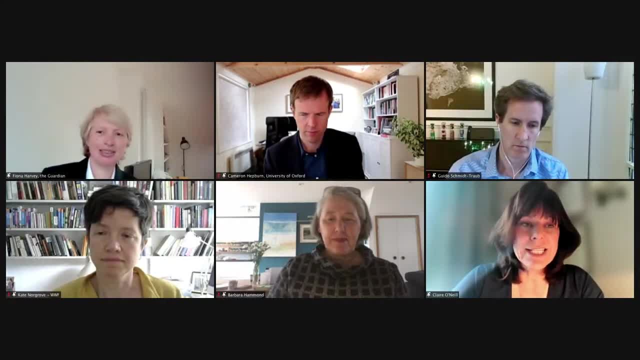 looking at geospheric removals. our companies are really keen to get into that space, so we're connecting very specifically uh with miles. i'm also doing some work with uh, the, the school of the, the economics programs and educational programs, to also be talking to them about. 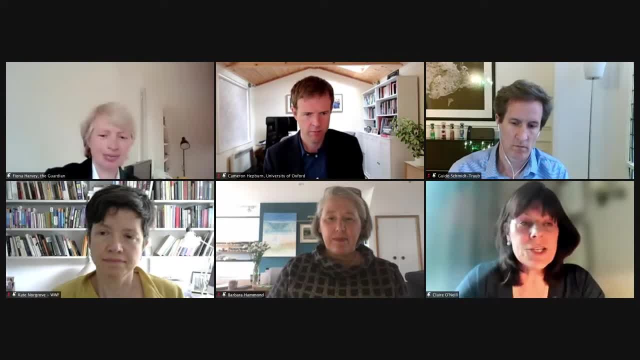 some of the sustainability needs we have. but this is why these initiatives are so great, because our members are desperate for this level of engagement and knowledge and, frankly, bringing the science to them. so many, many ways to work together- great, thank you very much indeed, and uh, you've helped. 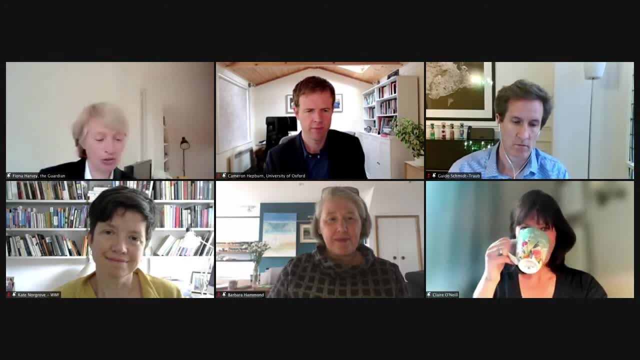 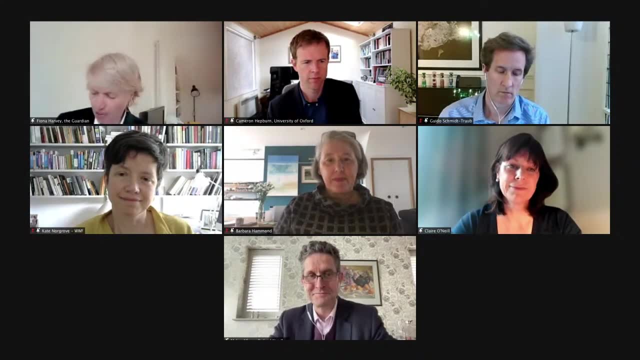 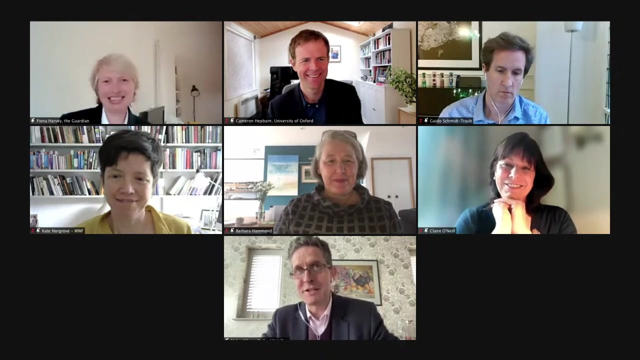 me to introduce our final panelist, uh, who is, of course, miles allen, a professor of geosystems at oxford, and miles, uh, as we've just heard, apparently. uh, ministers don't listen to scientists. is that a your experience as well? only some of us. well, we can but do our best to make ourselves heard, but so i think that it actually brings um. 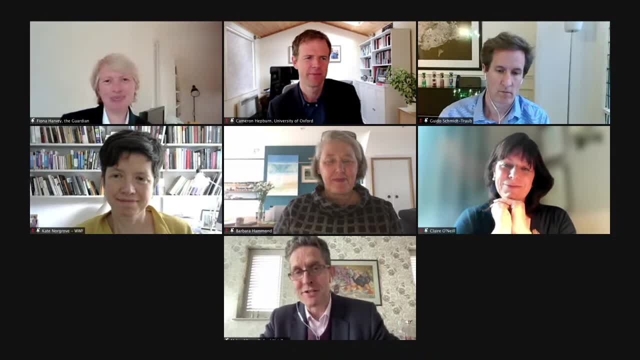 you know, the nice thing about coming at this point in the series is i can respond to lots of things that other people have said, and i particularly want to pick up on what kate said. i think you were absolutely right, kate, to challenge us on our continued engagement with 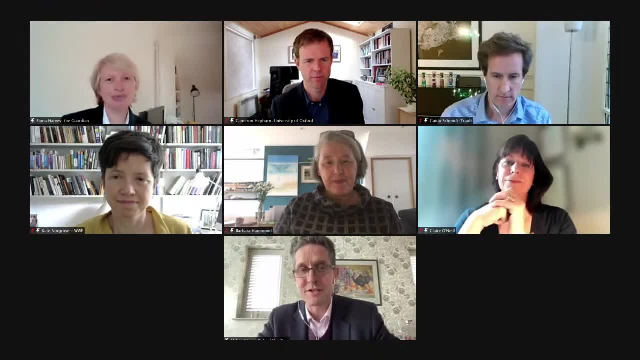 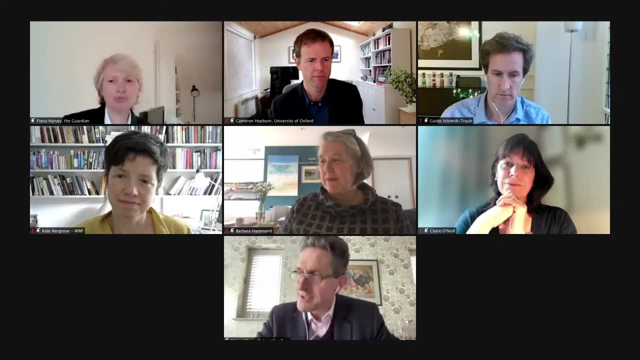 the fossil fuel industry. i mean it's. it is small, as david emphasized, but it's still there and it's an important symbol. um, and i and i'm- i will respond to you on this and say i'm, i'm proud that we continue to engage this industry. so this may not so this be speaking personally, i'm not on. 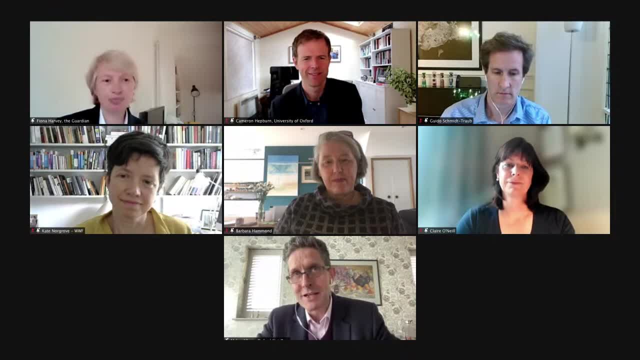 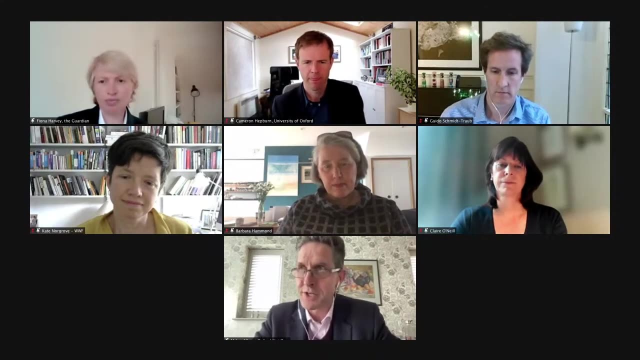 behalf of the university, and the reason is, um that the other great issue that the university is is grappling with at the moment, which we haven't mentioned, um today, but we have to always bear in mind, which is inclusion we need. we are a global elite institution, but we need to think at all times, and we have been 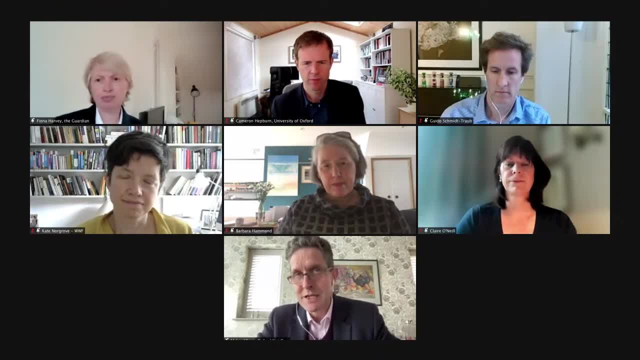 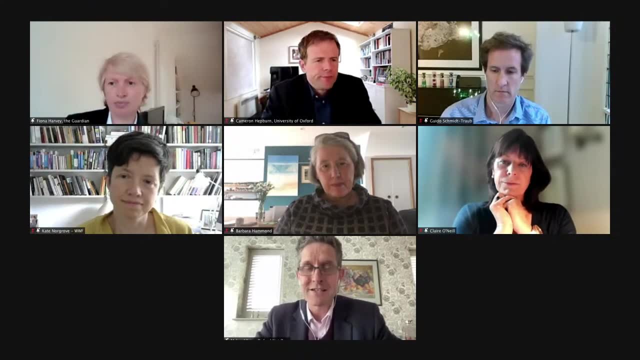 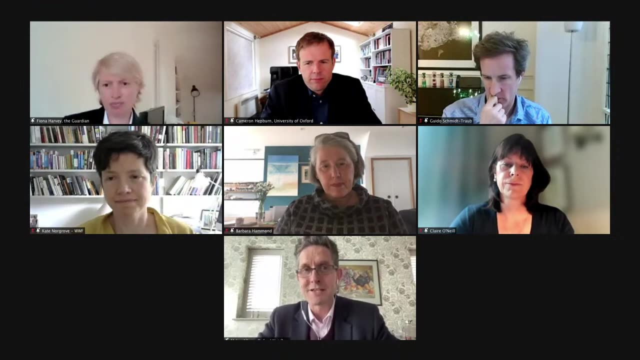 thinking at all considerably over the past couple years about how we increase our reach, increase our inclusion and when we're talking about net zero, net zero has to be inclusive, because there's no point in a net zero achieved by the world's elites that excludes large chunks of the world. 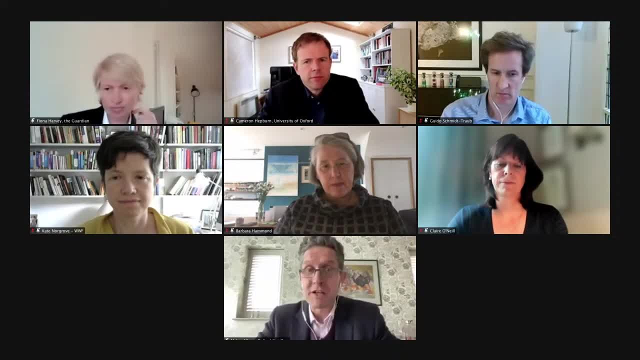 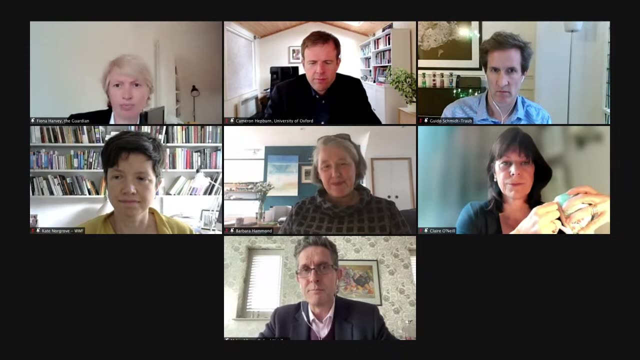 and inclusion can be tough. it'll mean including those who are currently working for the fossil fuel industry. maybe in 30 years time they will no longer be working for anything we would recognize as the fossil fuel industry, but they will probably want to have jobs. so we need to engage with them and what we are doing as a 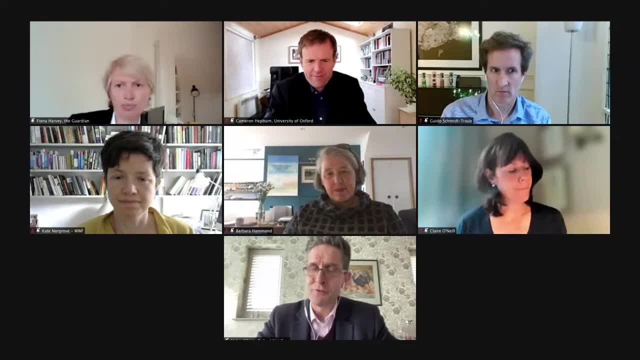 university, um, and, and this isn't- i don't think this is a formal policy yet, but i think it should be, and i'm going to say it now in the hope of making it more likely that it becomes one. i think we should absolutely apply exactly the same principles. 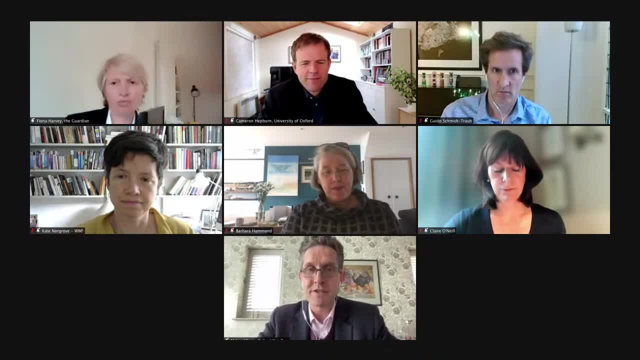 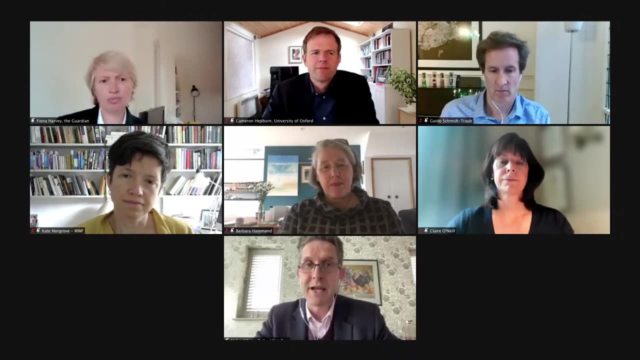 that we apply to our investment portfolio, which is the demand of any company we're invested in, or any company, therefore, that we're receiving money from, whether it's formally an extractive fossil fuel company or not, does it have a net zero plan that is consistent with the goals of? 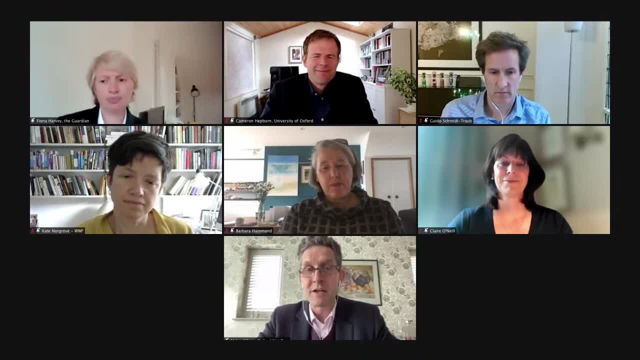 the paris climate agreement? and if it doesn't, why not? and can we help them get there? and if they clearly have no interest in getting there, then that's the time to disengage, but that's the time where we probably want to disengage, but that's the time where we probably want to disengage. 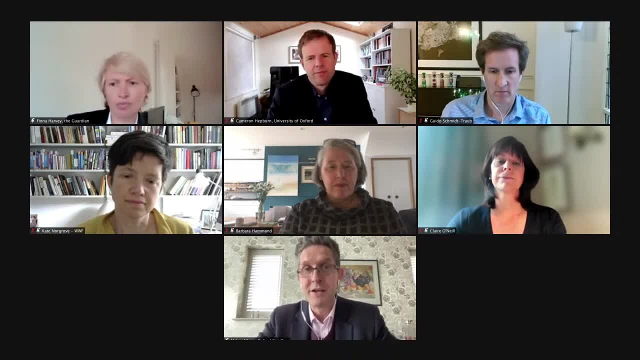 anyway, whether we're invested in them or receiving money from, because, frankly, a company that's exposed to climate related issues these days and doesn't have a clue about what its net zero plan is, it's probably not a company that's worth um dealing with in the first place. so so that's what. 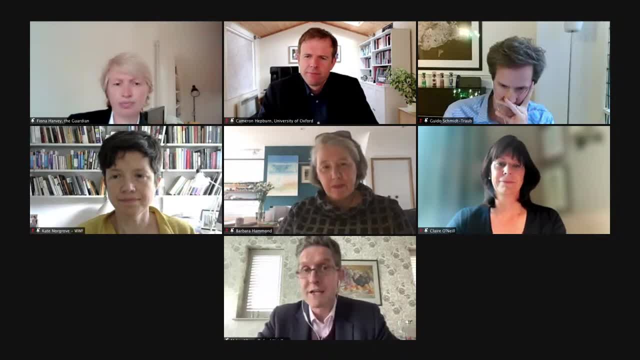 we're doing, uh, where we are therefore remaining engaged with the sector, um, i think that's the right thing to do, but it'll take some tough decisions going forward because, of course, there will be points where we will have to say, look, this isn't working out. we're going to have to. 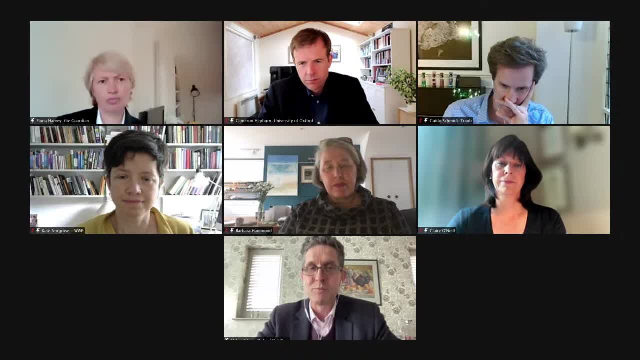 um, this, the, the company is just producing greenwash. uh, it's not actually serious. and those are the points where, going forward, we are going to have to make some tough decisions about disengaging um, but i think the, the rights, the right policy now is not a blanket sector-wide. 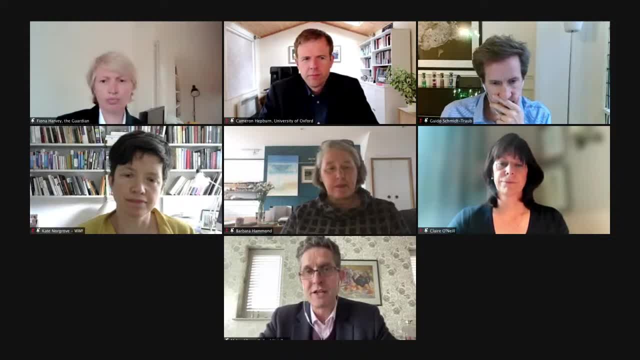 exclusion, but a, a policy of engagement with everybody we're dealing with to help everyone, and what we found actually since introducing that um congregation motion last year, the parliament um kaya played such a big role in shepherding through um and also things simple things like our, our careers service, um within, uh you know, a few weeks beforehand, just announced. 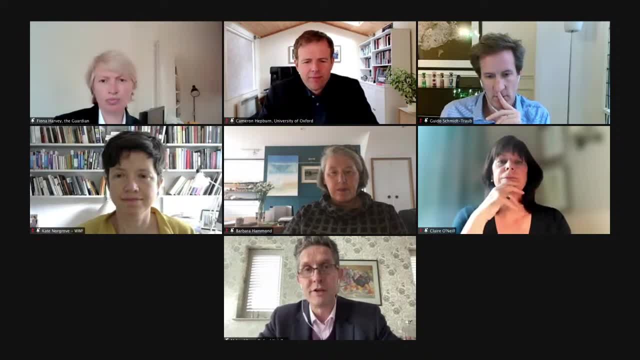 that they weren't going to let companies um join the milk round unless, um they produced a net zero plan and within you know minutes, apparently they was being phoned up by companies saying: can you help us produce a net zero plan? that's an example of how things can work in a very positive way. 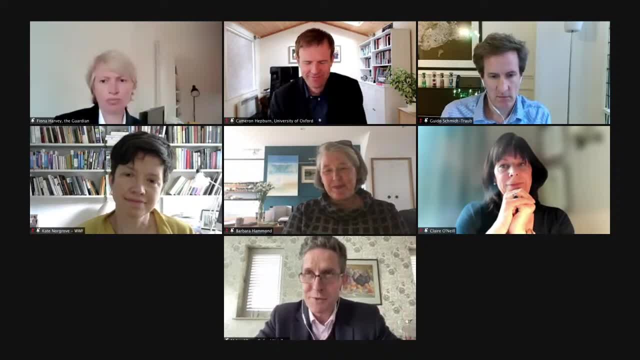 um, if we engage, and- and i so, i think we, i think that's the challenge for us. it's it's a hard one, and i accept that it means us dealing with people, who, who, some of our, our own students and indeed our own staff and our own academic 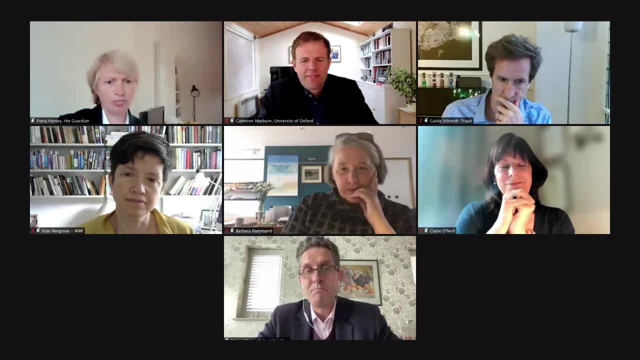 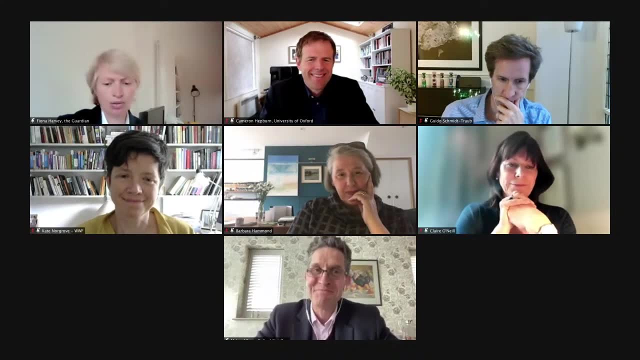 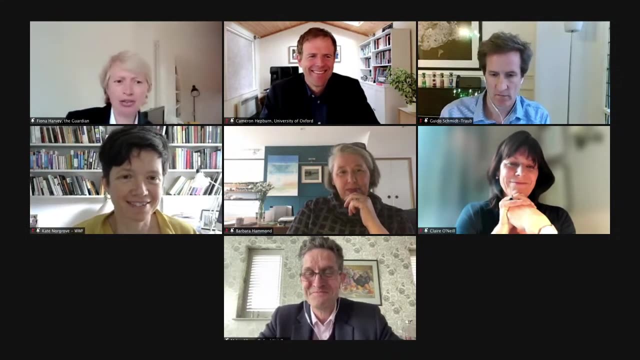 colleagues would feel, no, you shouldn't deal with them at all, um, but i think it's the right thing to do. but we also welcome you challenging us on this because we need the challenges. okay, thank you very much. uh, thanks for that. that would be controversial to some, um, and i'd like, at this point, i'd like to. 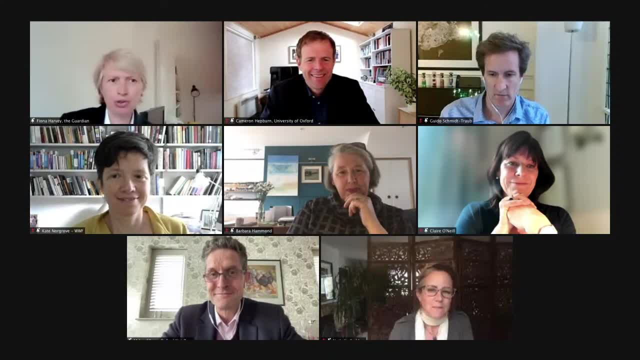 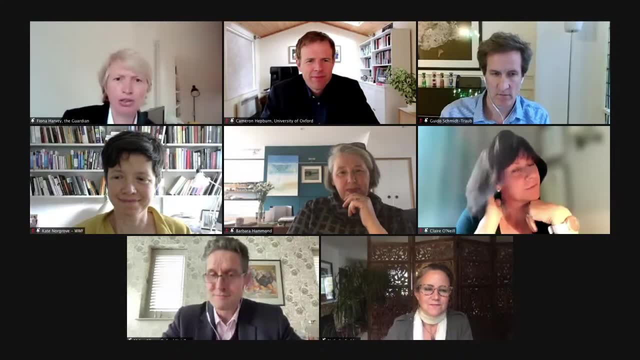 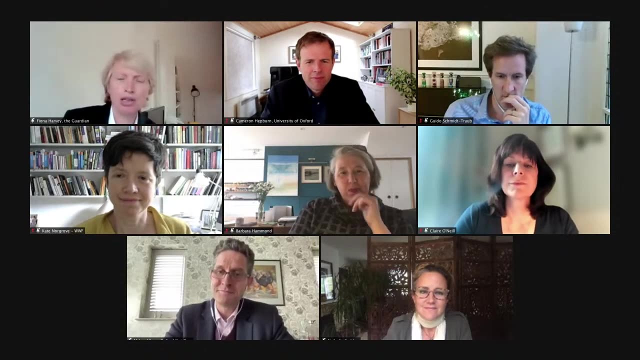 bring you back in uh? um, because we've just heard from miles that, um, you know all uh companies the university engages with uh should have net zero strategies. but what about biodiversity? um, should companies be judged on their impact on biodiversity, whether the university engages with them? um, i think companies 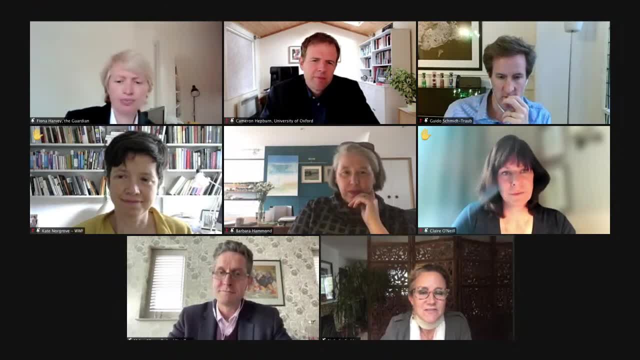 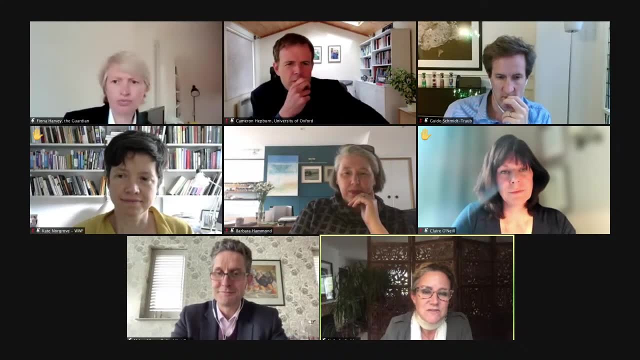 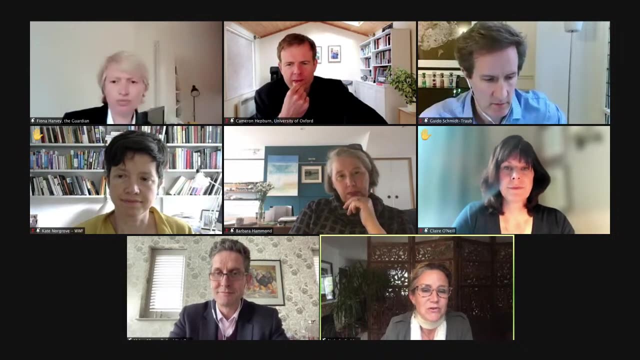 are increasingly recognizing the huge risks they face: reputational risks, liability risks, opportunities lost of not paying the debt they owe to the university- and i think that's a very in their development. there's widespread recognition that actually to future proof and ensure that you're profitable, that you also have to take into account in a rigorous way your impacts on the 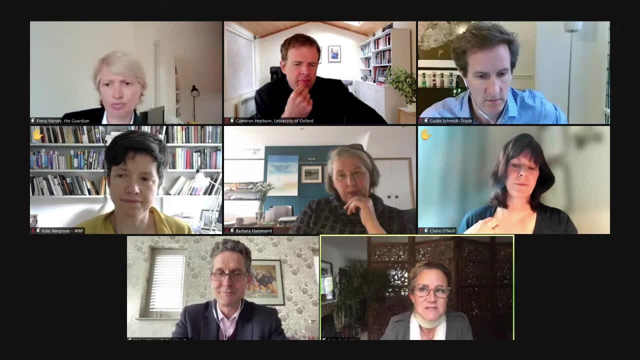 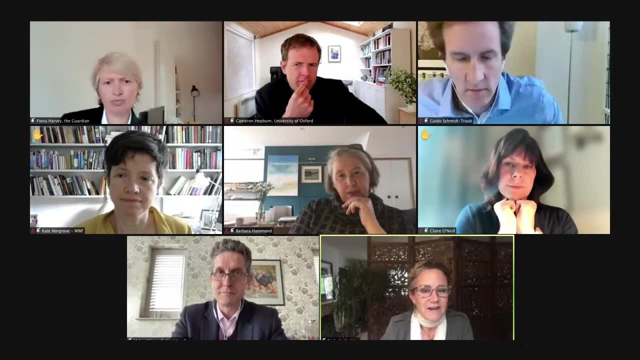 natural world, that the natural world is responsible for your proper profitability, ultimately, and so we're seeing a shift in the zeitgeist in recognition of that, and many companies are recognizing that they need to work very closely with scientists to ensure that the targets they set for nature as 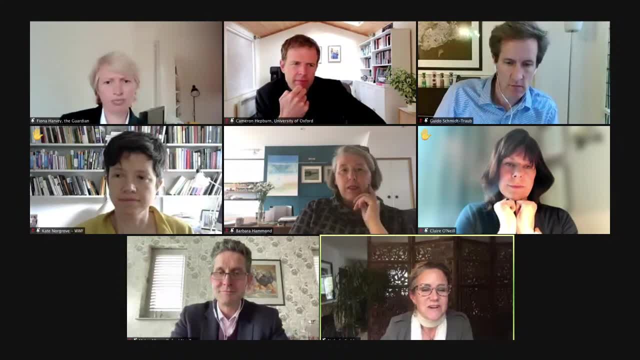 well as climate are not the same as the targets they set for nature as well as climate, and so um and especially those that they set for nature and climate simultaneously are meaningful, are achievable, are verifiable. so there's a lot of work to be done to ensure that you know it isn't. 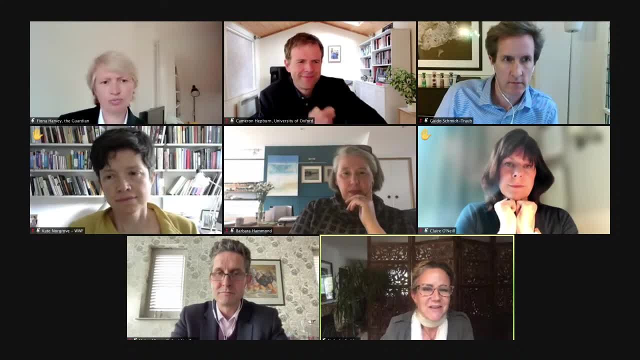 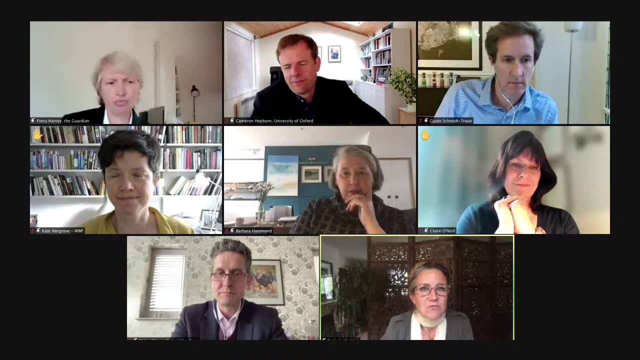 greenwashing, and it's or green wishing, or time washing or any of the other these terms that we're, that we're hearing at the moment. so absolutely, and i think there's, there's, there has been a shift, but there's a long way to go before we can. we can make those nature positive pledges achievable. 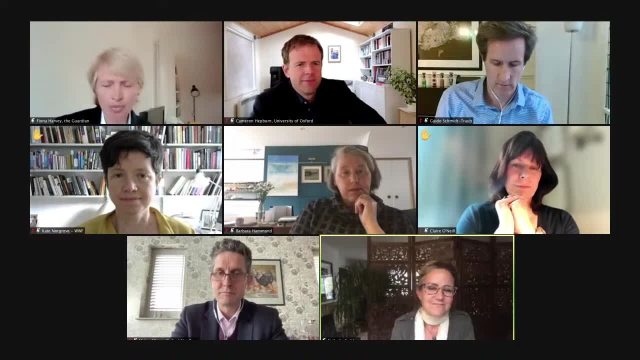 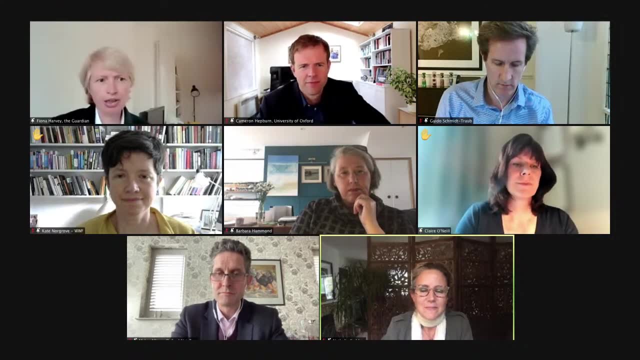 and meaningful. thank you very much for that. uh, i can see that claire and kate would both like to come in on this subject. uh, claire, i'll take you first and then kate. you started off this configuration. i'll take you in a moment. 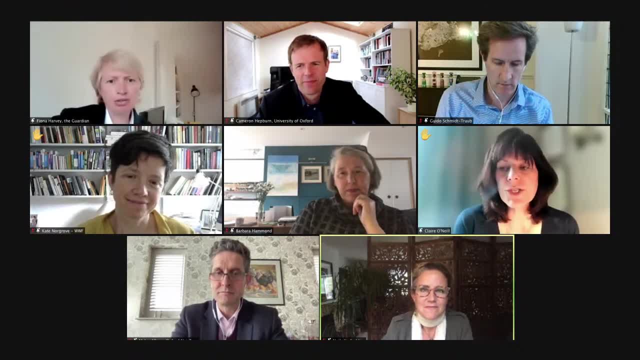 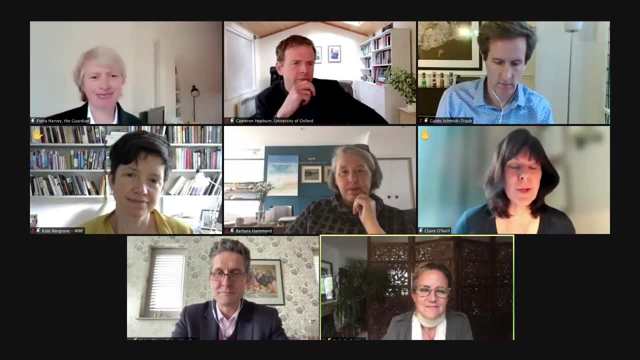 claire, please. thank you very much, fiona, and i just wanted to sort of violently, violently, agree with what natalie said and, and, i suppose, again point out that wbcsd- by the way, i'm not on commission and it's a not-for-profit organization- but the new membership criteria that have been put. 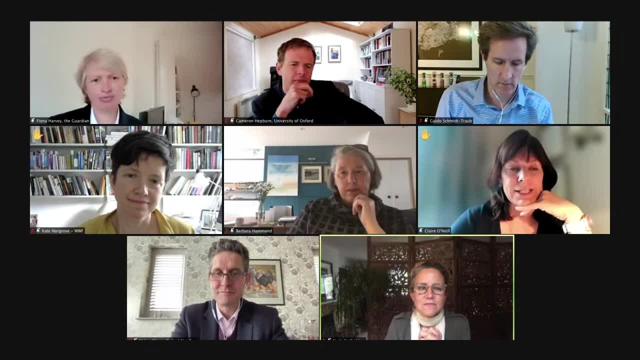 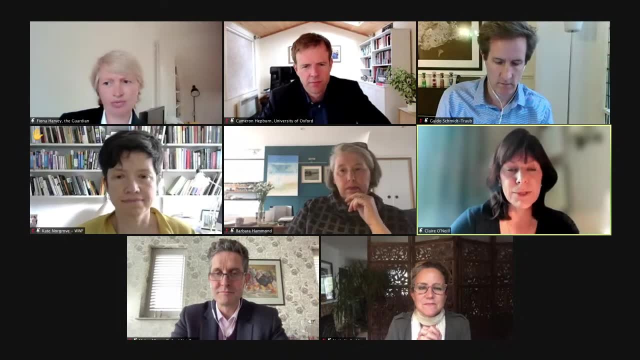 in place for 22 are both climate positive and climate positive and climate positive and climate and nature positive. and yes, while we're waiting for the sbti guidelines on nature, we're working to develop our own that members can sign up to, and i do think this is almost the next leg of the. 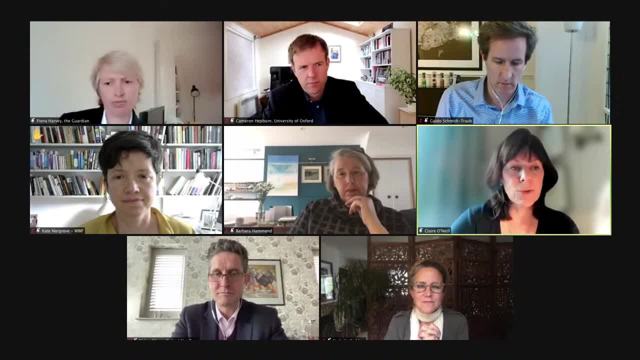 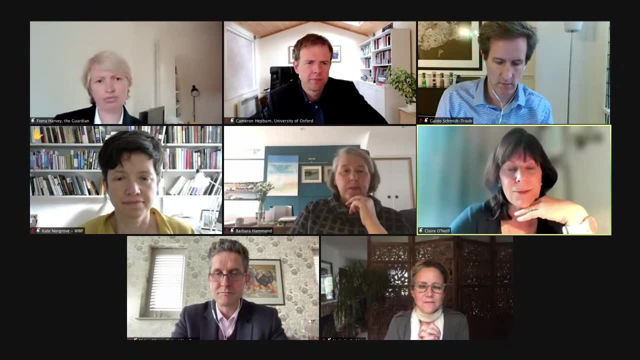 discussion and why the presentations today were so incredibly important. and again, the other third thing we're not, we have, we don't talk enough about is is inequality and the just transition element of it. so the world's most ambitious companies want to sign up to this multifaceted 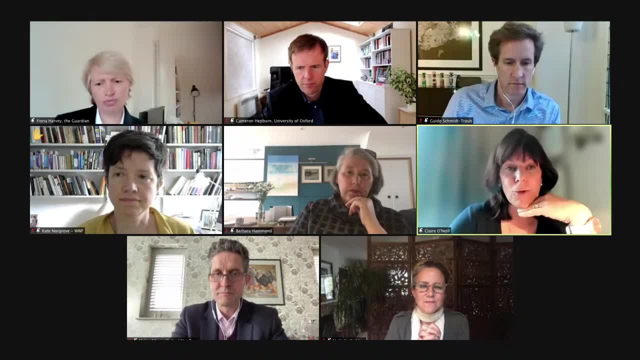 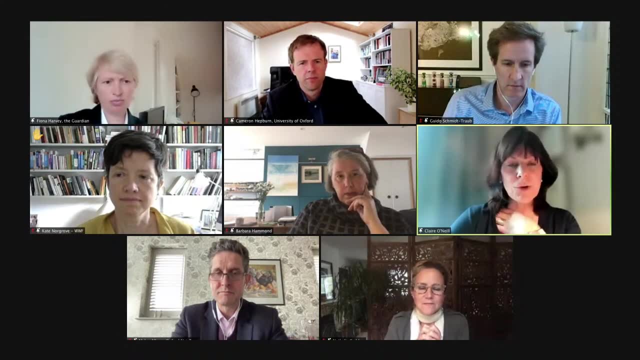 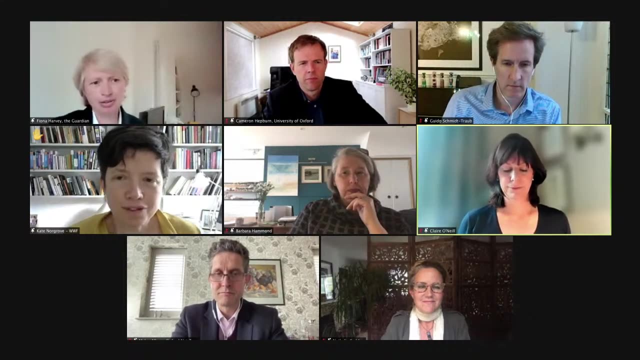 definition of sustainability and it, you know. and again, it will be a great calling card for oxford if indeed it was pushing some of that um, some of that multi-stranded, with the multi-stranded requirements as well. thank you very much. thanks for that. and, kid, what would you like to say? yeah, i was just going to say. 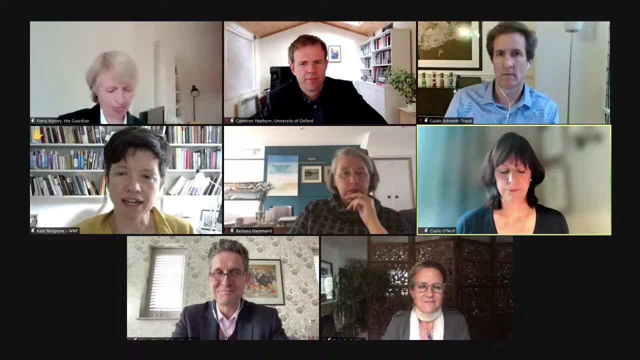 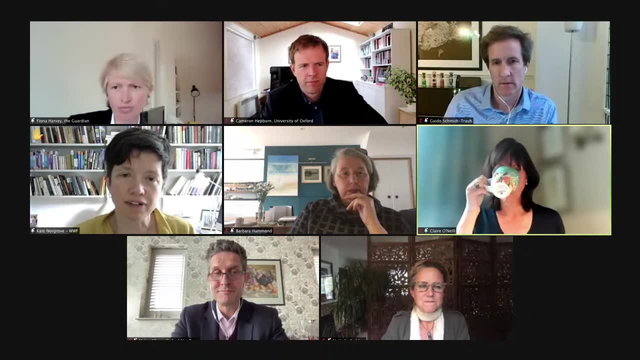 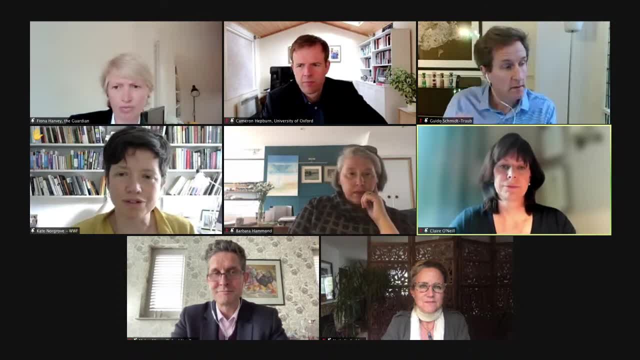 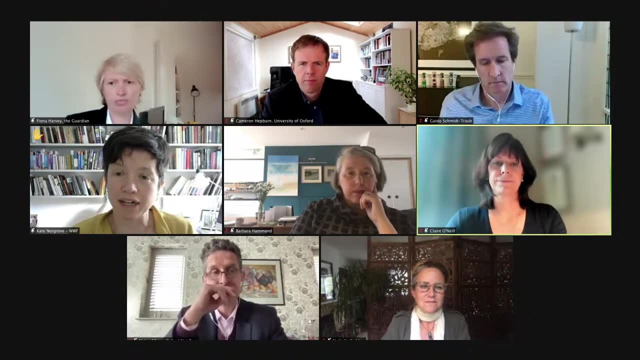 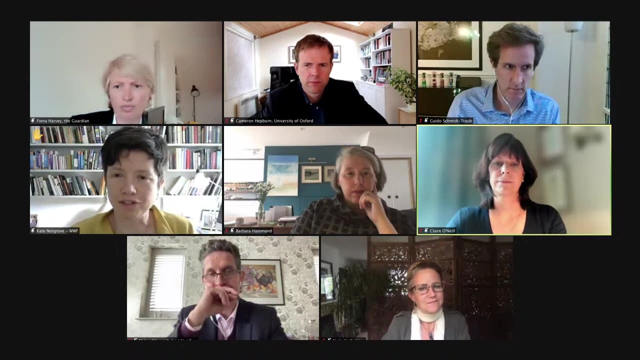 in development. um, i would endorse your suggestion miles of only working with companies that have a net zero plan. potentially biodiversity plan as well, um, but i would suggest that it would need to be a plan that's endorsed by the science-based targets initiative, and whatever you think about. 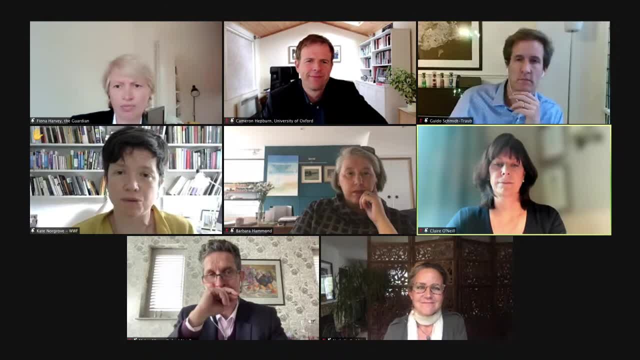 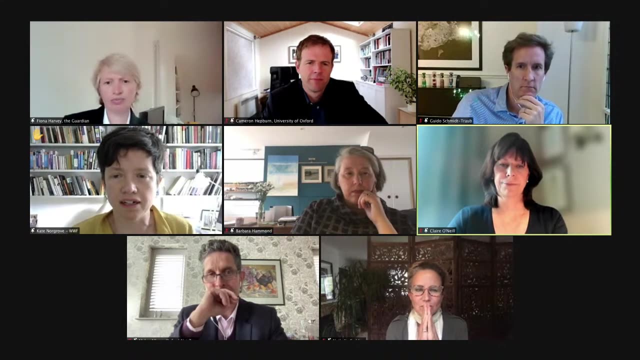 that initiative and obviously there's a lot of work, particularly on the nature side, to get it to a point where we have targets that are verifiable and possible to measure. it is a place where people can come uh to to get some certainty that the net zero plans. we see uh around and 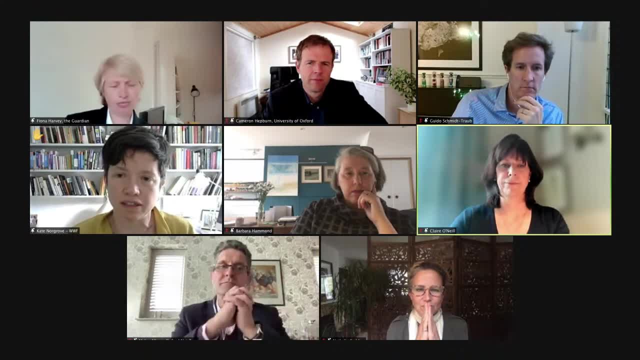 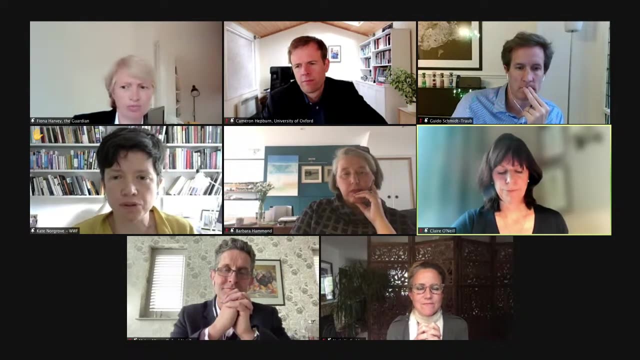 everywhere at the moment are actually um plans that are going to achieve um and uh and uh of any good quality um. i just wanted to say that i think also, it's very important to work with companies on a pragmatic approach to a just transition, um, and and it's important that there are people that 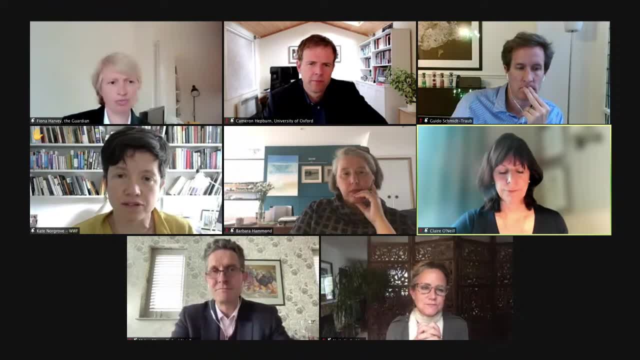 work on the inside. i mean, i work with hsbc, i also work with tesco's as part of the transition part of wwf and there are many people that would have us out of those companies, um, but it's important that in some areas we transition. my point was more about oxford university. should a 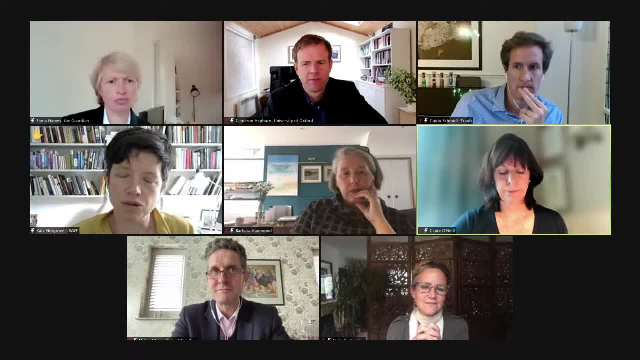 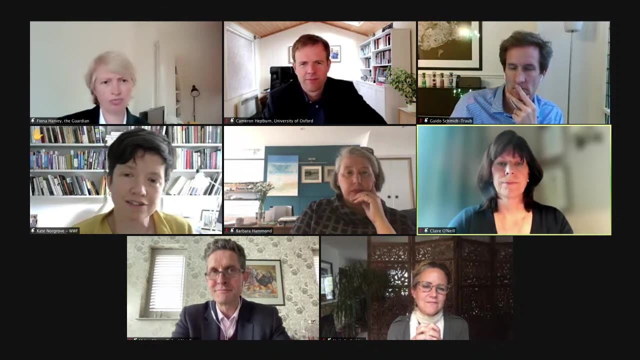 learning institution, uh be invested or be accepting these? uh this money, when we haven't seen the science-based targets? uh verified plan for these fossil fuel companies? um, and where there are, there is so much other money around that you could take instead, so i think that's something to think. 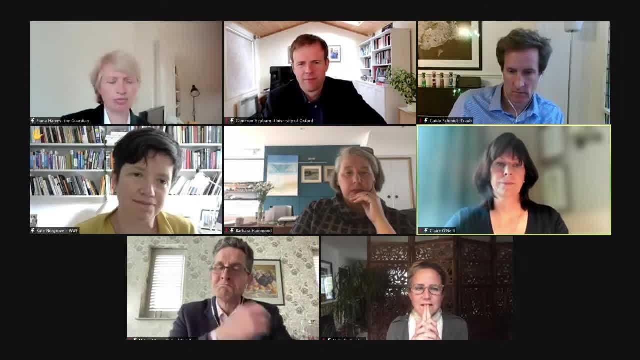 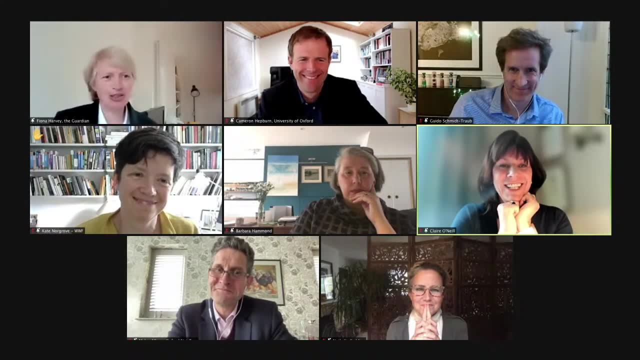 about and uh, and, but very much welcome the discussion. great, thank you. okay, i'd love to know where these uh pots of money that are that are lying around instead. but uh, we'll come to that another time. uh, i'm going to ask whether we can actually have one of our questions. wants to know? 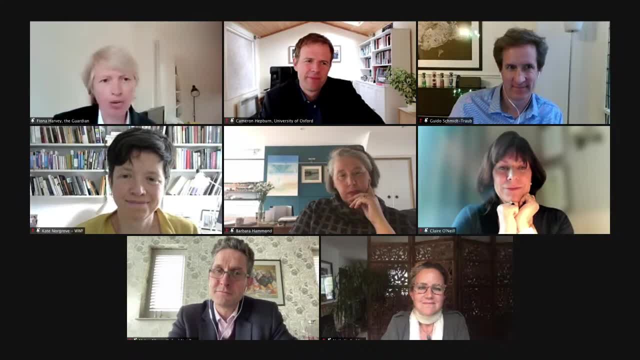 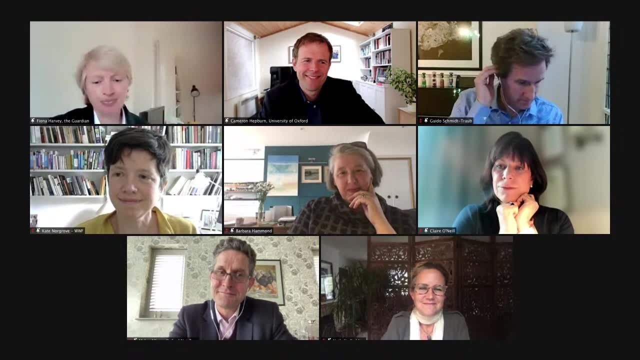 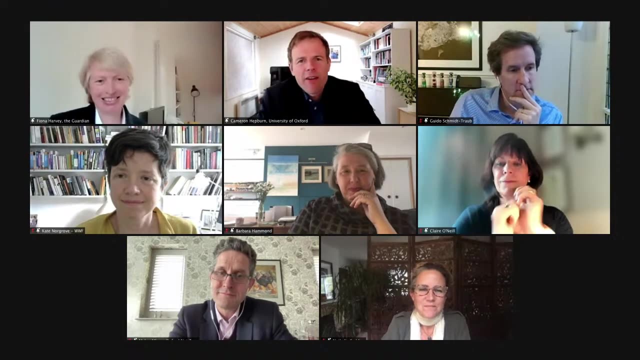 whether you can actually have economic growth and environmental sustainability. i'm going to put that to you, cameron, and to guido. please, cameron, first, that's an easy one, yeah, but the the kind of second layer of the answer is that i mean we clearly can't have it in the 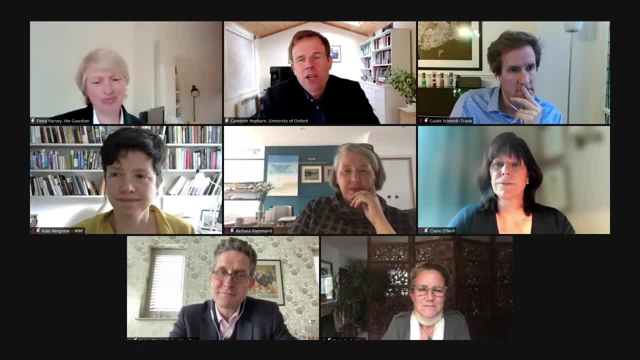 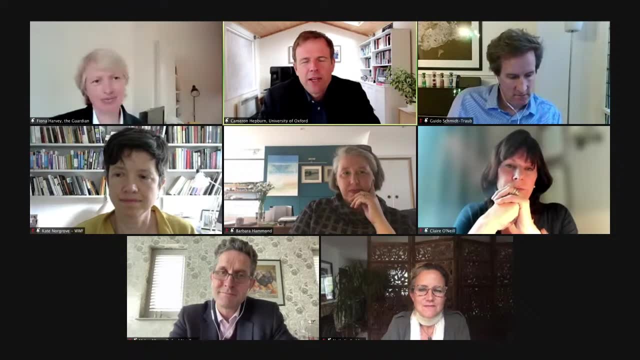 current model, economic model. it needs to change quite radically, and the way it needs to change is through a combination of human ingenuity, the kind of ideas that oxford's been offering the world for decades, actually, but but more of them, and new ones, uh, whether it's the future of plastics. 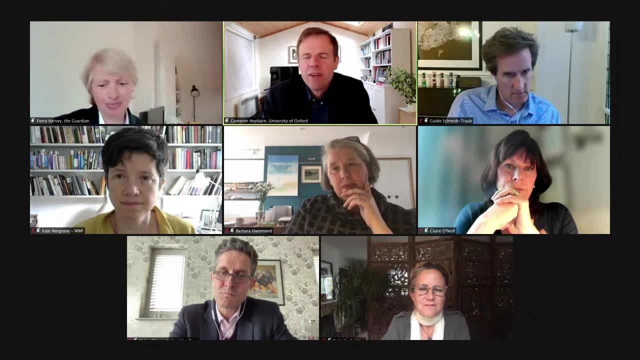 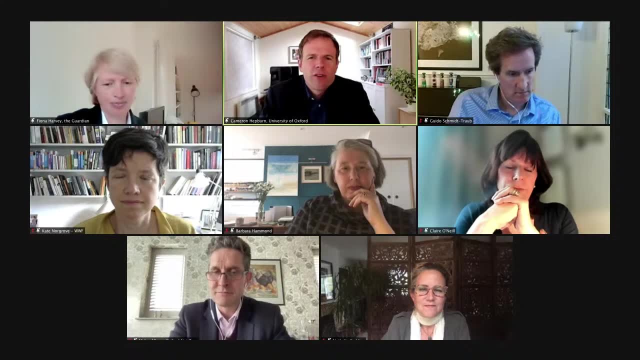 program, the sort of work you've been to just outlined in this lecture, what natalie's doing, i mean all of these ideas and more are required to shift the and technological structure of what we're doing, so it becomes nature positive, not nature negative. but it's not just technology. 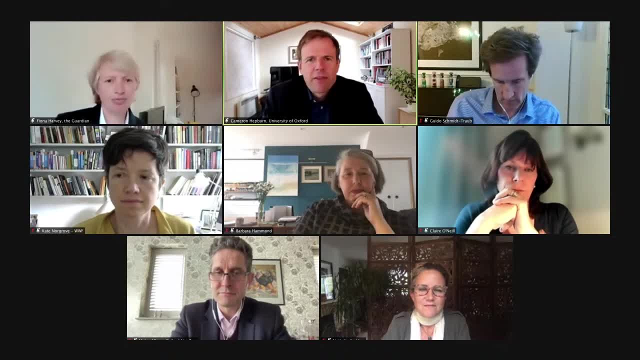 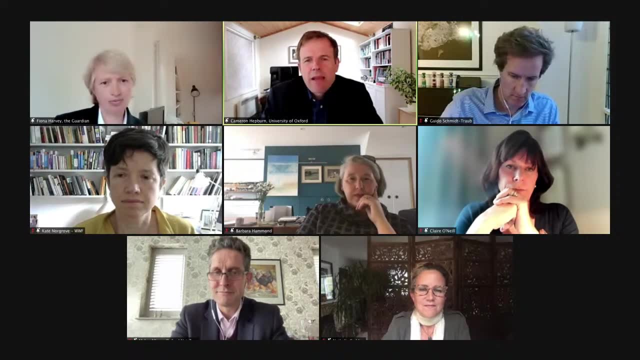 uh. i had a wonderful discussion with uh professor sapatha dasgupta last night from cambridge about his report on the economics of biodiversity and a big part of the story. to make uh continued economic prosperity and environmental protection compatible is how we think about our preferences. 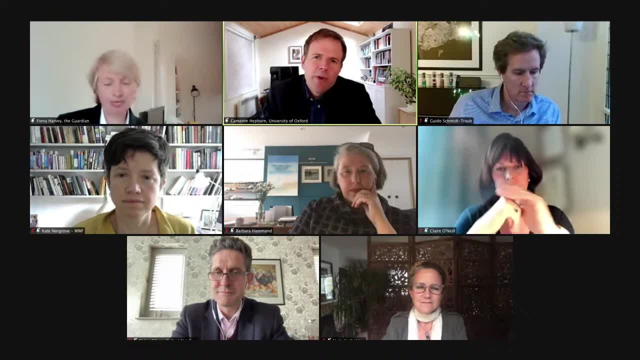 and our own decisions and choices and, as he's been pointing out for decades, they're socially embedded and but that doesn't mean we can't do something to change the way in which we all think about the choices that we make. so it's complex, uh, fiona and questioner, but it's certainly. thank you. 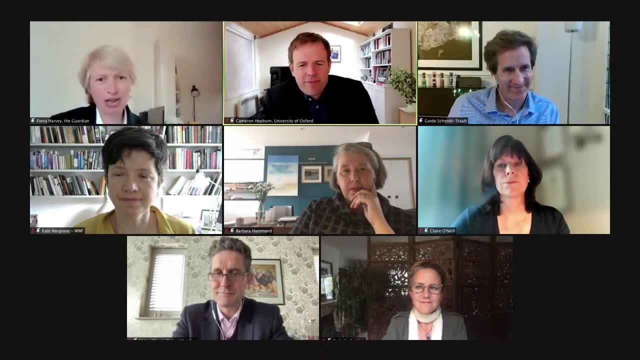 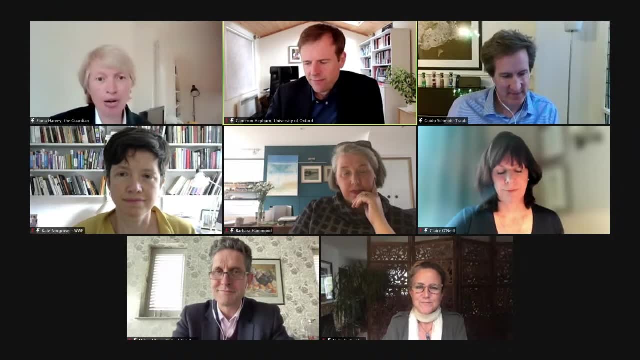 thank you very much indeed for that, guido. i'm going to give you a chance to address this as well, and then i'm going to put one final question, uh to barbara after this, because we're running out of time, uh. but, guido, uh tell us, can you have environmental growth, and or can you have 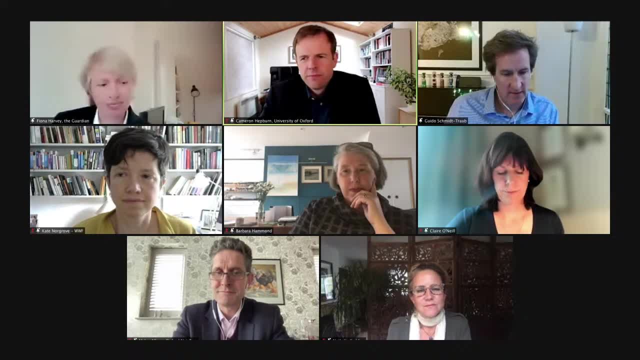 economic growth and environmental sustainability. well, yes, i am, i'm firmly convinced of that- share camera's assessment. but the truth also is, nobody really knows, because there is no high-income country that is environmentally sustainable, that has zero emissions. so, um, i have no question that we can solve this, that we can work this out, as camera said, but this: 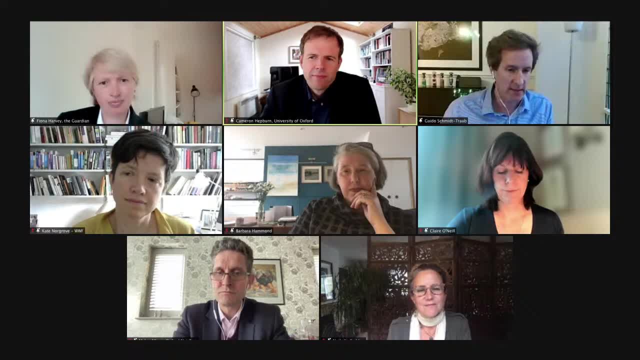 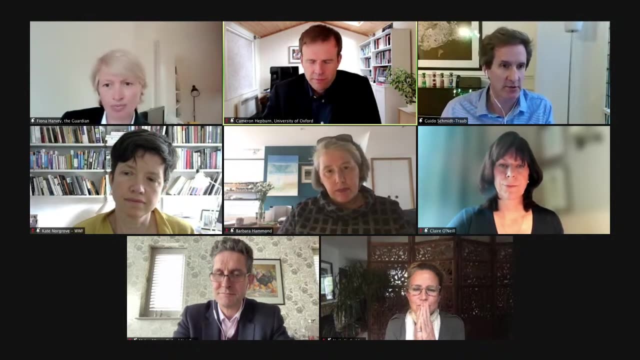 requires dedicated processes. we need to align market incentives with them. we need to have really targeted problem solving. and i think it's quite illustrative and quite instructive if you look at what the european union has done last week as its new industrial policy. first of all, it's rediscovering. we're rediscovering the term industrial policy. we do not 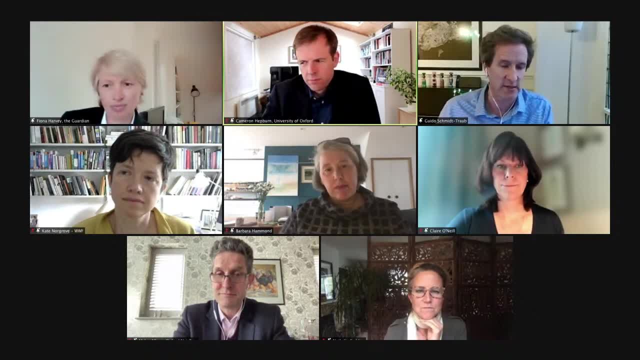 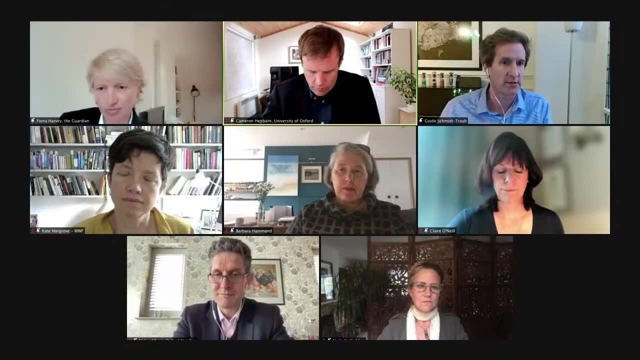 need to have forward-looking long-term strategies of targeted investments, or something, of course, which has been discussed in the uk a lot, and the eu ties it inextricably to two major challenges, and that's decarbonization, but if we should add biodiversity to that, um plus digitalization. 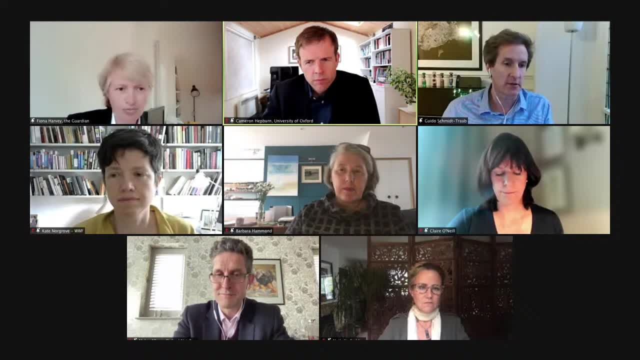 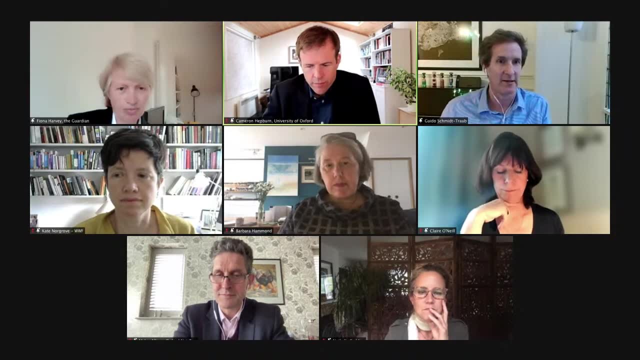 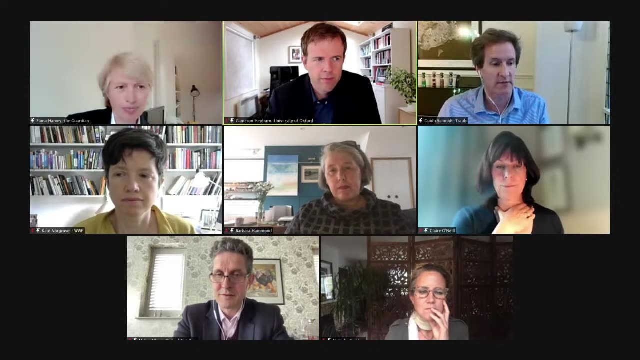 um, and it makes it a question about austin's long-term future and the long-term sovereignty of europe. because, um, if europe doesn't innovate in these areas and the uk doesn't innovate these areas, others will um and they will determine growth in the future. so i think this is absolutely possible. we're going in the right direction, but we need to invest far. 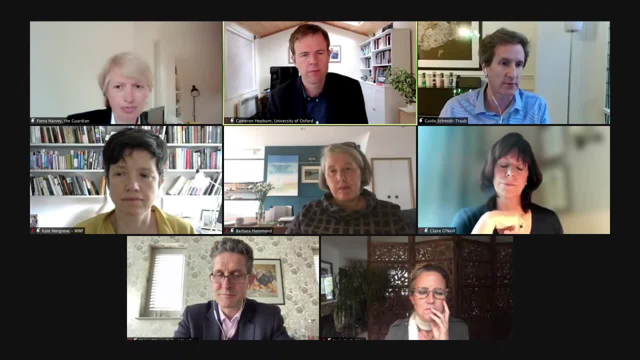 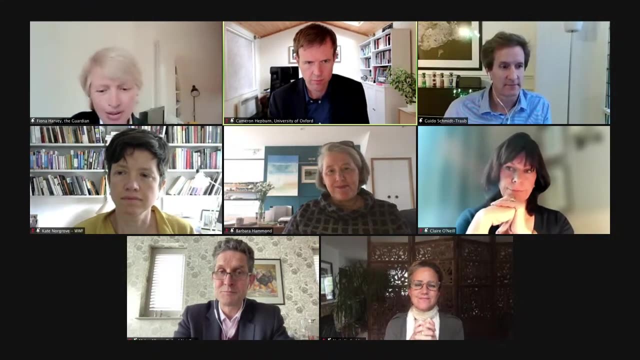 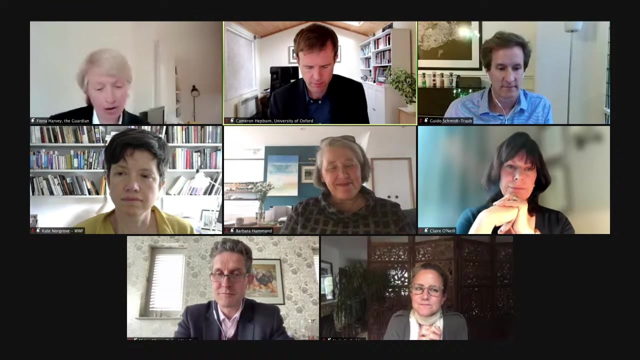 more um in these new technologies. we need much more creative public-private partnerships and that's why i think you know the net zero strategy in option almost is a laboratory thinking this through. also working with businesses is really an important piece in the puzzle of problem solving. great, thank you very much. thanks for that. uh and barbara, i said i'd come to you, uh, for one final uh. 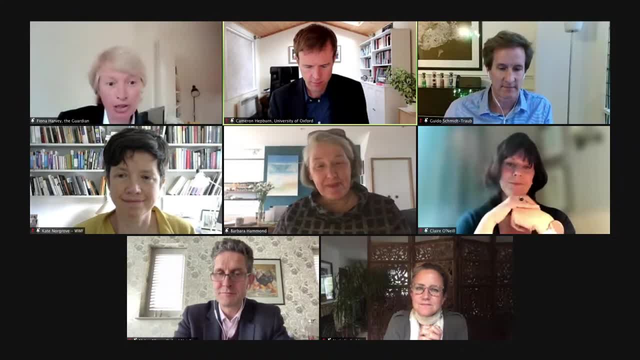 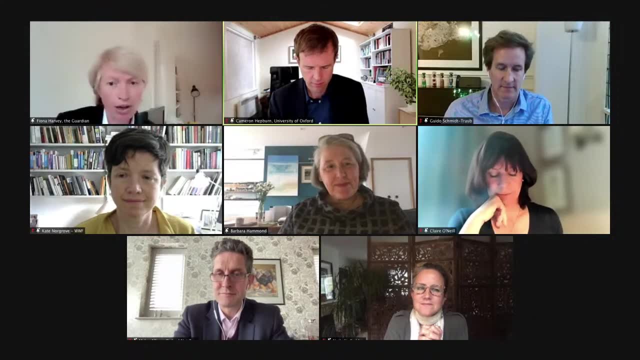 um, in fact, it's going to be two. actually, if you don't mind. one is very quick because you're the low carbon hub, uh chief executive of the low carbon hub for oxford, and we've got a question about making all uh university vehicles uh electric. do you think that's going to happen? 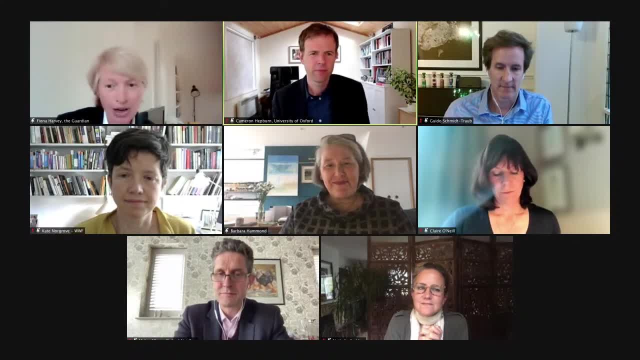 in oxford, um. and then i'd like to ask, uh, we've got a question about uh oxford alumni, um, you're one yourself, um what can the network of uh alumni around the world from oxford contribute, uh to these goals, please? okay, so question number one: um, we're all going to be in evs. 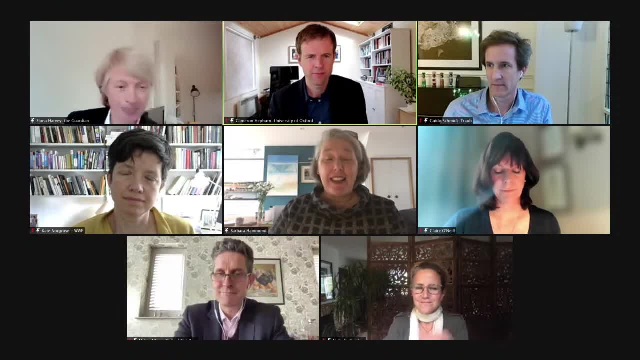 much more quickly than we ever thought we would be, and the uh. the issue is not about us all wanting to do that. we're all bashing the door down and getting very cross about how slowly the infrastructure is being rolled out and how unreliable it is. so, yes, the university is. 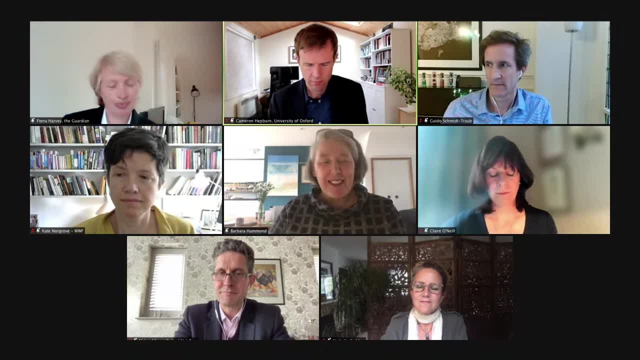 going to be all ev um. it's a question how we're going to provide the infrastructure, and hopefully we'll do that in a way that balances the energy system and doesn't need masses more um generation than actually we do need because we're over providing for peaks. 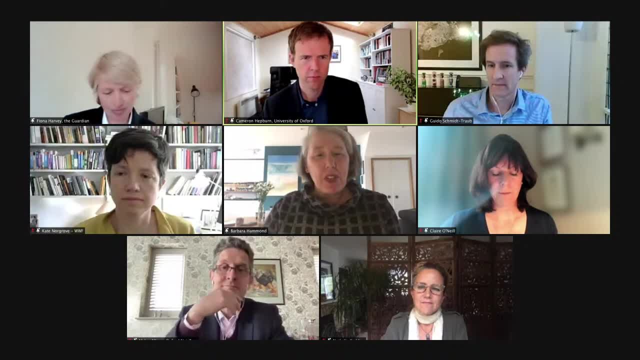 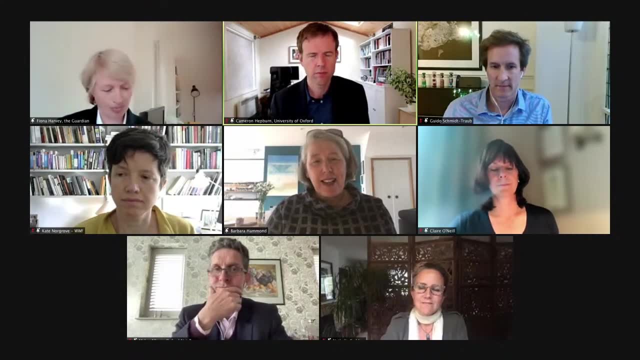 um, so that's thing number one. um, thing number two: alumni. yes, thank you for that. um, i am, uh, an alumna of um of oxford. um, i'm not a scientist. by first degree, um, i was a modern linguist, and so one of the points i wanted to make this is that i'm not a scientist. i'm not a scientist, i'm not a. 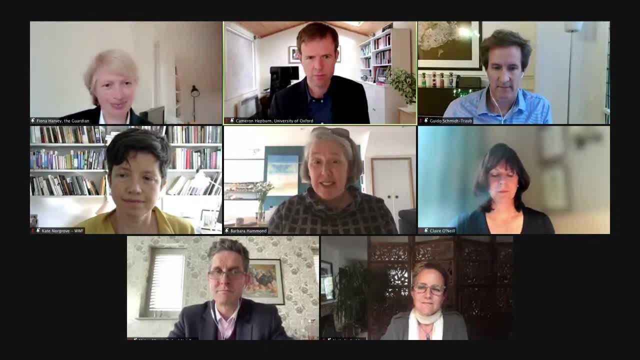 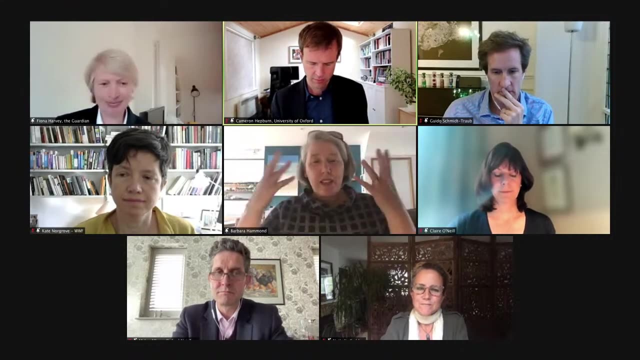 you've given me the opportunity to do is this is not just about science and technology, and the one network in oxford i hope is going to involve arts and humanities as well, because they have masses to bring to the way that we think about, um, how we describe these things, how.